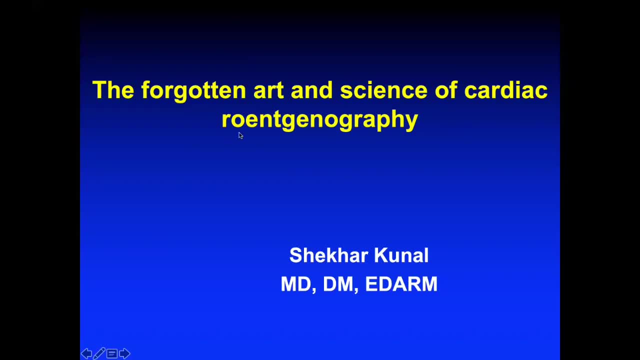 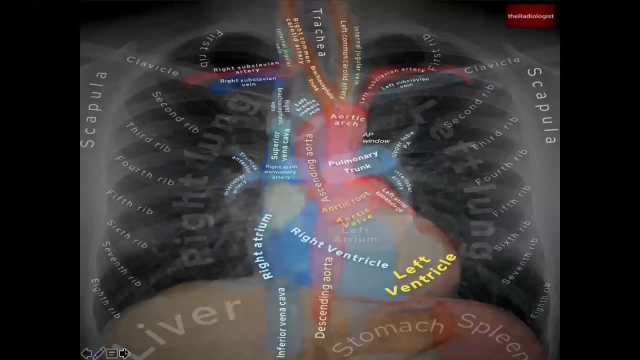 Good evening everyone. So today we are just going to discuss the forgotten art and science of cardiac rogentography. Now, this is all what we are going to see or read in a basic cardiac x-ray, and this is one of the composite images where everything has been summarized in just a single image. 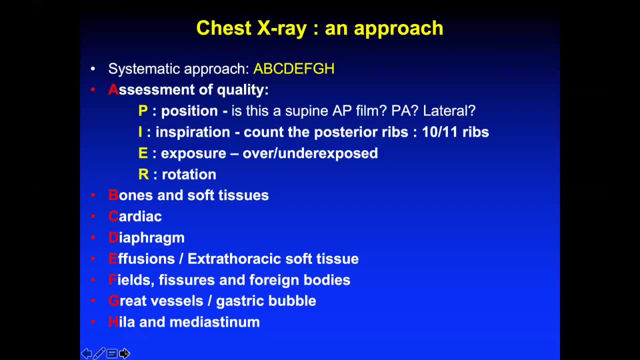 So let's see whenever you are reading a chest x-ray. So we'll start with the basics, that what should be an approach of reading a chest x-ray. The reading of a chest x-ray should always follow a systematic approach and the systematic approach just clarified as A, B, C, D, E, F, G, H as an 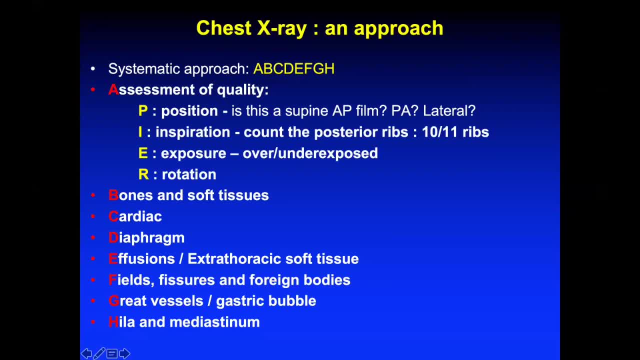 approach. So first thing would be assessment of the quality of x-ray, and for that either you can use a mnemonic pier or ripe. That is, P stands for position. Now, is this a supine film? is an AP film, PA film or a lateral film? Then you see the inspiration: whether this is an inspiratory 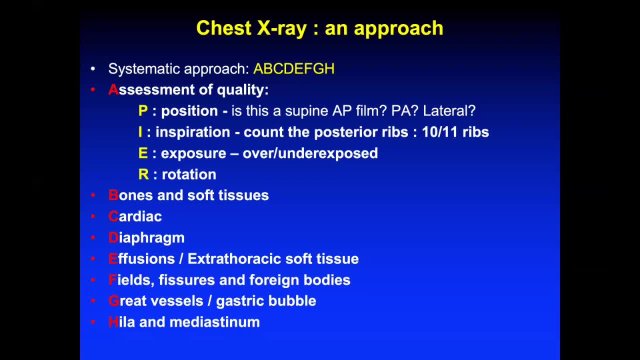 film or expiratory film. You count the anterior ribs, Then you see the exposure, whether it's overexposed or underexposed. and last of all is rotation, whether it's rotated to the right or left. Then we come to the bones and soft tissues. C is the cardiac, the cardiac margins. Then you see the diaphragm. Look for the. 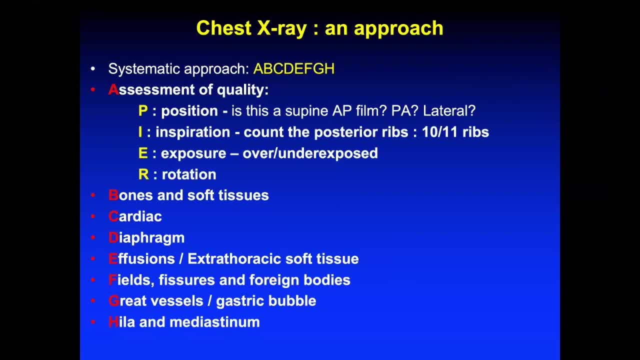 effusions or the extra thoracic soft tissues. Then the fields, that is, the lung fields, the fissures, the horizontal oblique fissures if they are visible, and the foreign bodies if they are present. G stands for great vessels and the gastric bubble. Now, gastric bubble is an important point. 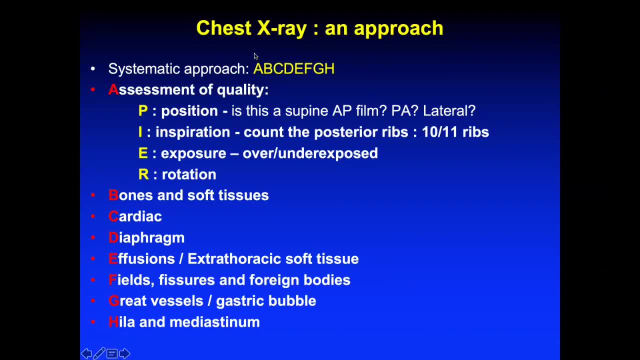 in making this a diagnosis for situs That will be later on, and then we look for hyala and mediastinum. So this is what we go from A to H. This is the approach and this is what one has to even follow, even in your exams or whenever you're interpreting an x-ray in your routine practice. So 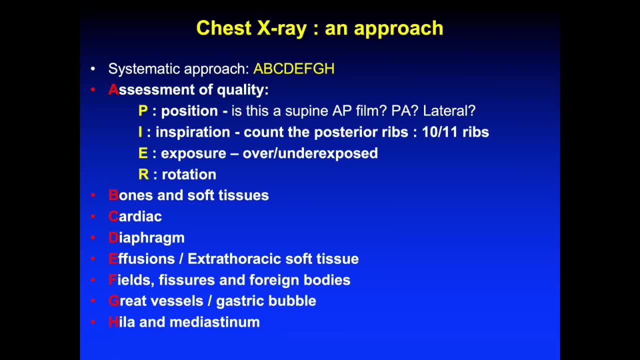 this is the systematic approach. Never go haphazard, that once you just describe the x-ray, you just say: and then directly you reach the lung fields or directly you know any opacity which appears as an abnormal. Never do that approach. Always follow a systematic approach and that is the easiest way. 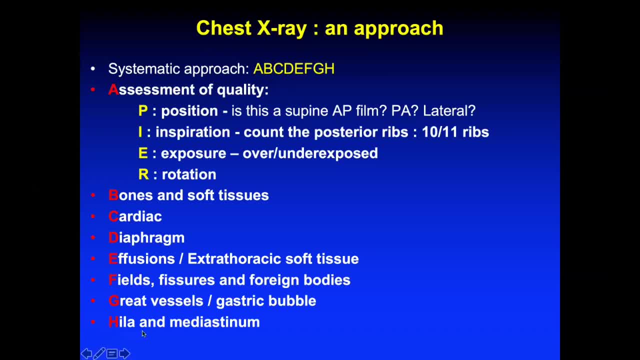 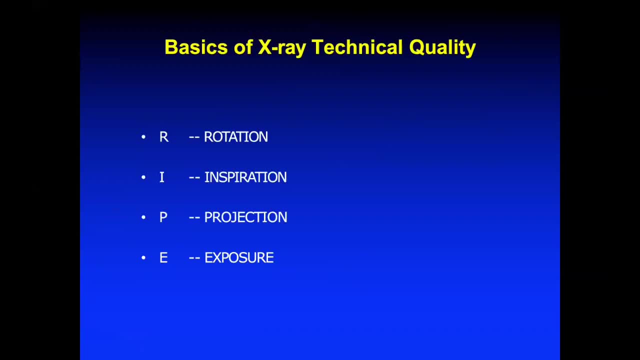 out even in your exams, whenever you're given to describe an x-ray. So first thing would be the basis of technical quality and this is the most important, because whenever you're going to analyze an x-ray, if the quality of the x-ray is not right, you should not comment further on what opacities. 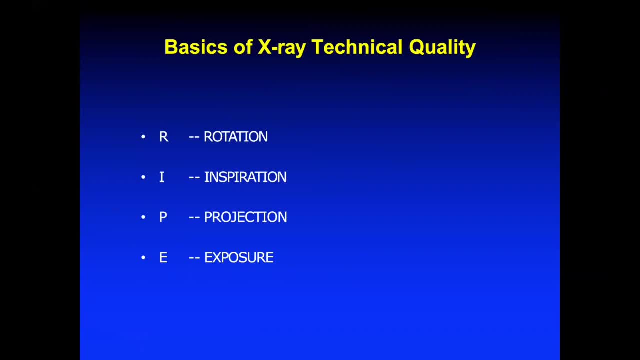 or impurities are there. So in exam, if you're given an x-ray and the quality of the x-ray is not fine, just mention to the examiner that okay, this is the right word- rotated x-ray film, or the poor inspiratory film, or it's a underexposed or an overexposed film. So you should always mention: 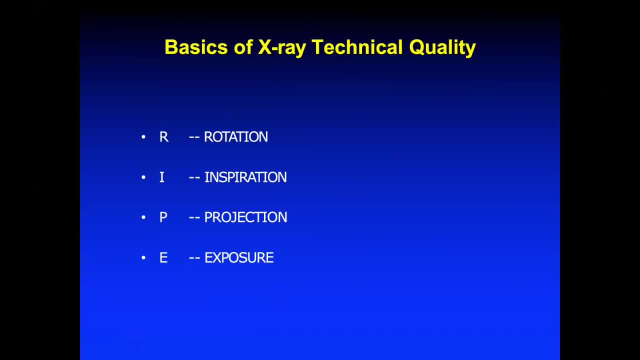 this before you go on describing any abnormality in the x-ray. So we have four things to look at. the technical quality First would be the rotation, then would be the inspiration, then would be the projection and the exposure that the mnemonic is right. So first thing would be rotation, The first 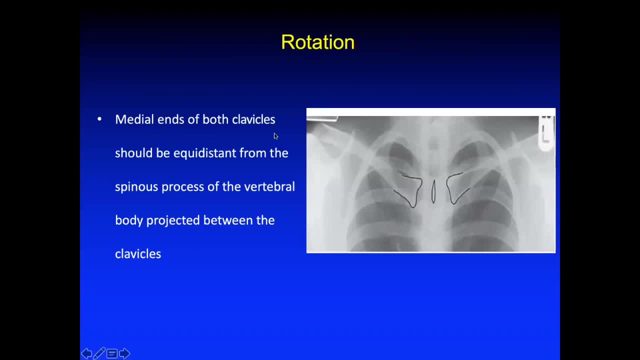 and foremost thing to be describing rotation, whether the x-ray is normal or whether it is a vertical rotation. you just see the medial end of the clavicle and the spinous process of vertebrae. so here you can see clearly the spinous process of this vertebrae. where is the vertebrae and the 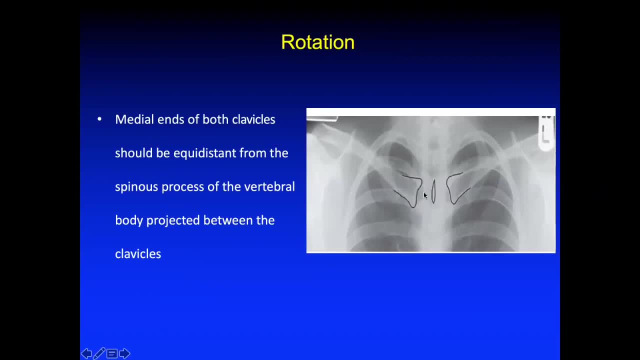 spinous mócus vertebrae. Normally, when the film is not rotated, the distance between the medial end of the clavicle and the spinous process on both the side is equidistant, so this should be distance on either sides. So medial end of both clavicle should be equidistant from the spinous process. 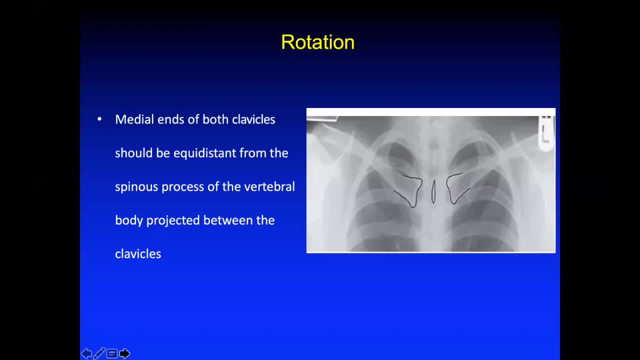 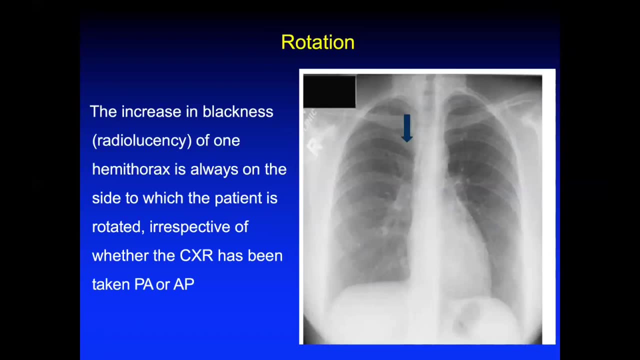 of vertebral body projected between the clavicles. This is the normal rotation. there is no rotation whenever there is rotation. why we are more concerned about it? because towards the side of the rotation. suppose the x-ray is rotated towards the right side. on that side there will 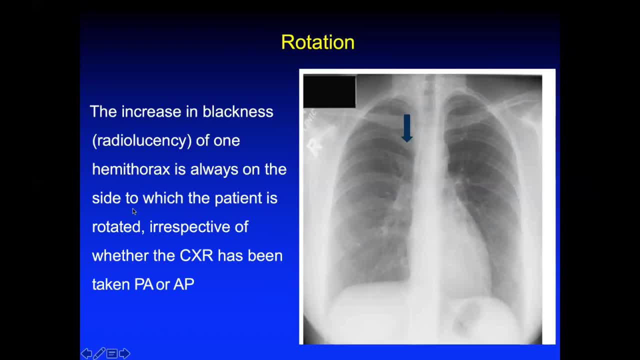 be increase in blackness. that is, radiolucency on the hemithorax, on the side to which the patient is rotated, whether the x-ray is PA or AP. so irrespective of the AP or PA film, whatever is the side of the rotation, there will be radiolucency. so you cannot comment on the opacities, whether 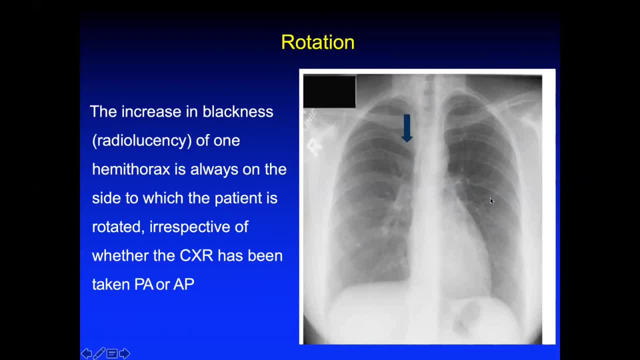 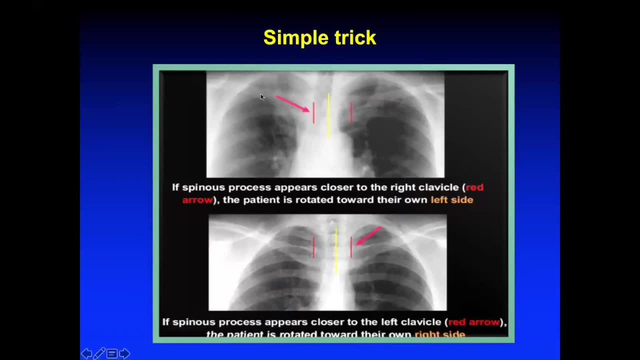 this area is hyperinflated or the other area will be an abnormal appearing. so, first and foremost, you determine the rotation. a simple trick to how do you say that, whether it is right rotated or left rotated, this is the spinous process and this is the median of the clavicle. so towards the side. 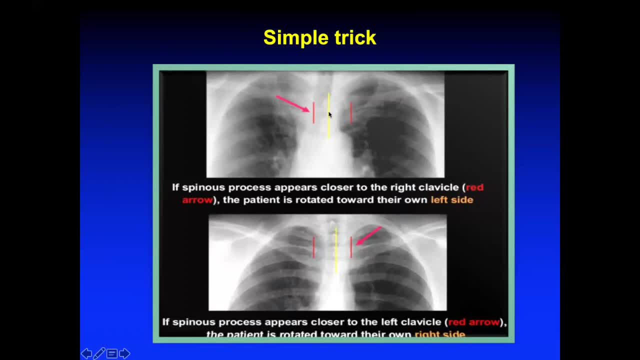 which is the smallest distance. always there is an opposite side rotation, or wherever there is a farthest distance, that is, from the median of the clavicle to the this spinous process. see, this distance is large, so the rotation is towards on the left side. so this is a very good, simple trick. 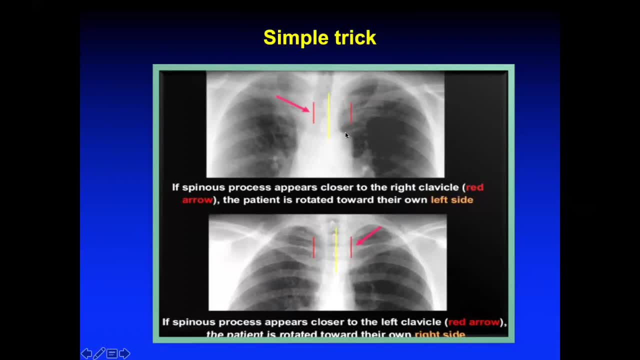 that just measure the distance and whatever the distance appears to be larger, it is rotation on the same side, or whatever distance is smaller, the rotation of the opposite side. now here you can see the left upper zone and the right upper zone. there is a mark distinction between that. this appears to be more radiolucent. this 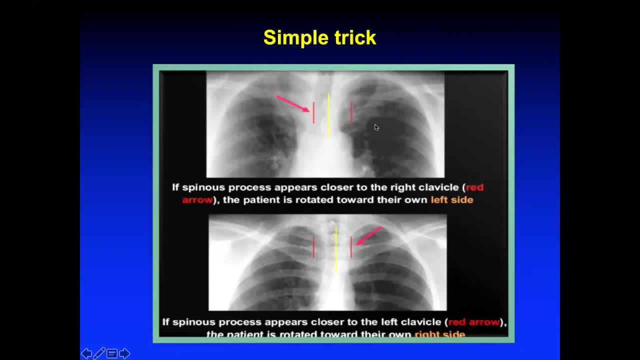 appears to be more or less radiolucent. so, since this was a normal x-ray, still, you know, because of rotation, on the side of the rotation there is increased radiolucency. same here now. here this end distance is less, this distance is more. so the rotation is on the right side. 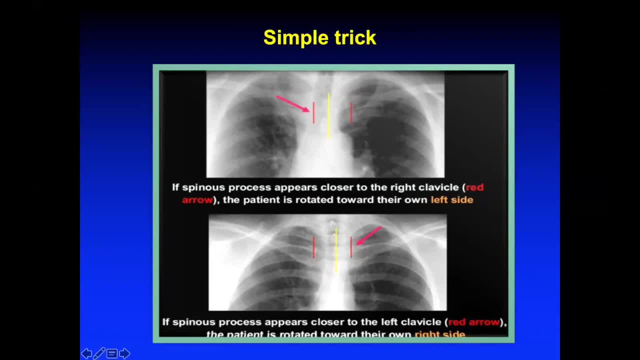 so this is the easiest way out. even if in exams you are going to describe or we get given an x-ray, that okay, which is the side, rotation is there. just follow this easier principle: you never confuse on the rotation side. so always the greater the distance the rotation is towards the same side. 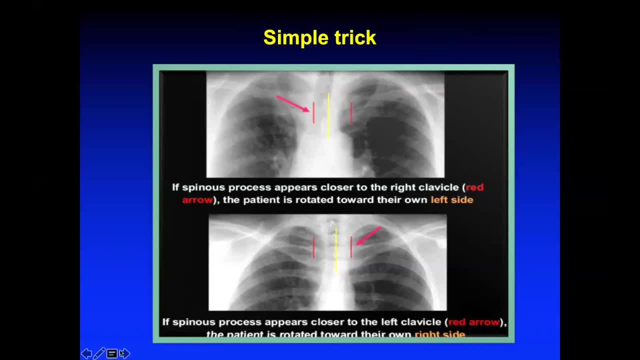 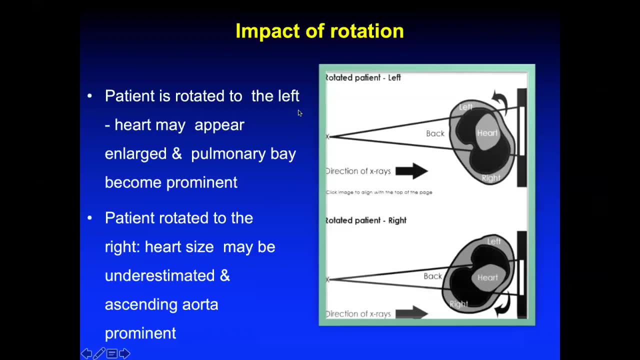 so that is very important. so then, the impact of the rotation. now why we are so much worried about the rotation. the biggest worry about rotation is because your apparent cardiomegaly. so here you see, this is the x-ray which is taken in the PA view. 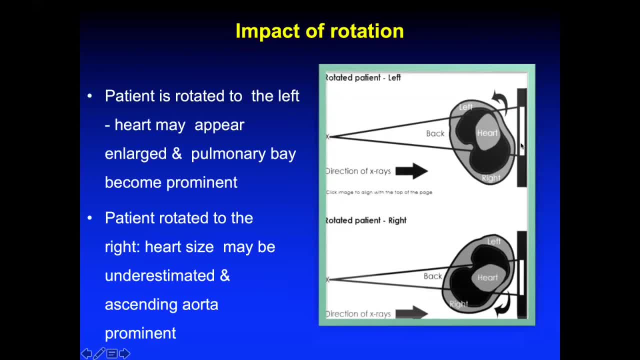 that is, the images are being projected from the back and on a film, so the heart is rotated. that is, you have a left-sided rotation, so rotation, the patient rotates on the left side. so from the back, the projections are there, so there is an apparent cardiomegaly. normally if it had been in the center. 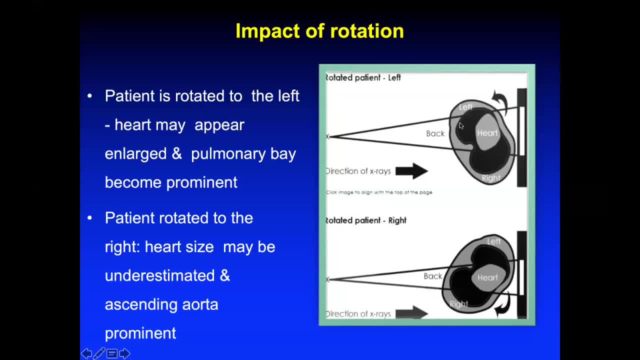 so till here only the x-ray of the heart would be projected. but here the beam widening is there and there's an apparent cardiomegaly. so on the left-sided rotation there's always an apparent cardiomegaly, the heart appears enlarged and the pulmonary blade that is the main pulmonary artery. 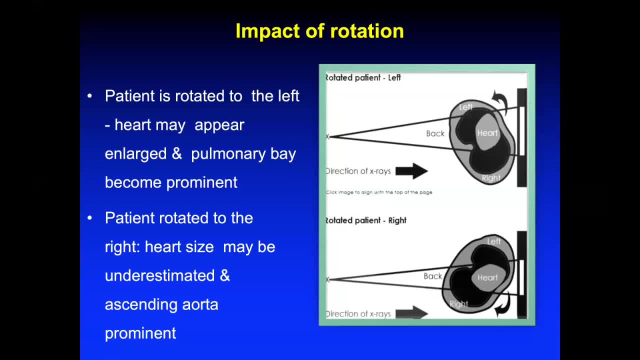 and its branches, they become more prominent. so a left side rotation is associated with a cardiomegaly and a pulmonary which is enlarged. a right-sided rotation always leads to an underestimation of the cardiac size. so there is less amount of bb's passing, but towards the cardiac shadow. so your heart size appears to be pseudo in a smaller size. 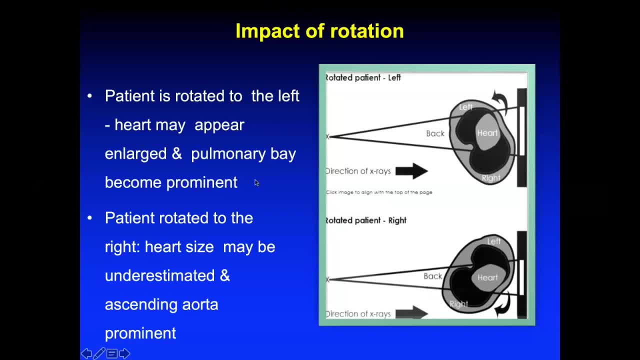 ascending aorta becomes more prominent, so you can make a diagnosis of an ascending aortic aneurysm. as a false diagnosis can be made based on this uh rotation. so this is very important. that why we need to have a rotated rotation in the x-ray. once you have confirmed that, okay, the x-ray there. 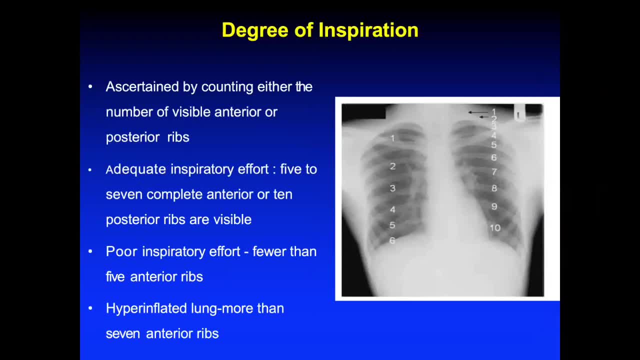 is no rotation. next, you should always comment on the inspiration. so in exam you will always be given to count out the uh rib spaces or the ribs. that is, either you can count the anterior ends of the ribs, which are the broad end, so the ribs generally in a pa view, the rips will follow. 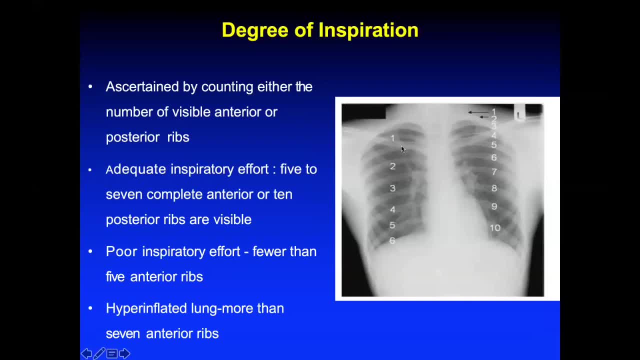 from the spinous process to anteriorly. so this is the first trip. this is the anterior end of the second rib. this is the anterior third rib. this is the anterior end of the fourth rib. this is the fifth rift, six rips. so these are the anterior ends, whatever ends anteriorly. and uh, there is. 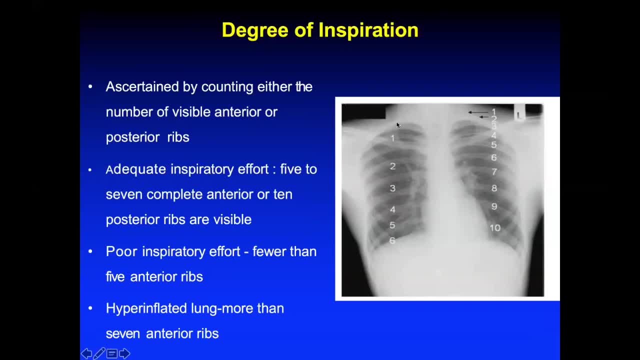 space out here because there's a posture cartilage, so this is an anterior. so you can count the anterior end of the ribs from one, two, three, four, five, six, or you can count the posterior, posterior end, that is from the spinous process, posterior margin. so 1, 2, 3, 4, 5, 6, 7, 8, 9, 10. so 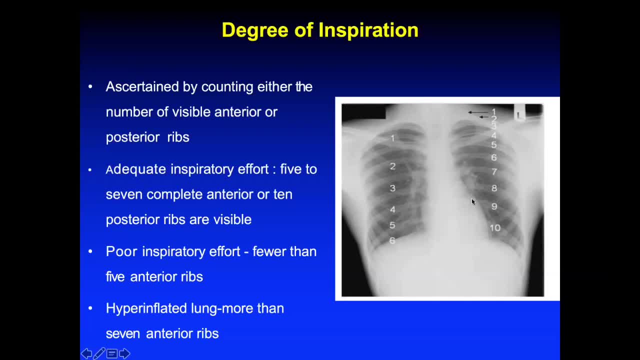 whatever which is appearing more towards the heart, these are the posterior ends, and whatever it's appearing within the lung fields, these are the anterior. so this is a very easy way to remember that, obviously, which are closer to the vertebral body or closer to the heart, these all will be. 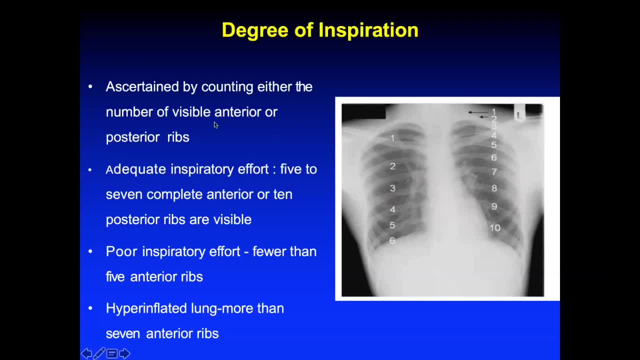 the posterior end of the ribs. so you can kind of either anterior, posterior. so a good inspiratory film will have either 5 to 7 anterior visible or at least 8 to 10 posterior ribs. so 10 posterior and at least a 6 more than 6 ribs on an anterior film. so this is basically a requirement for 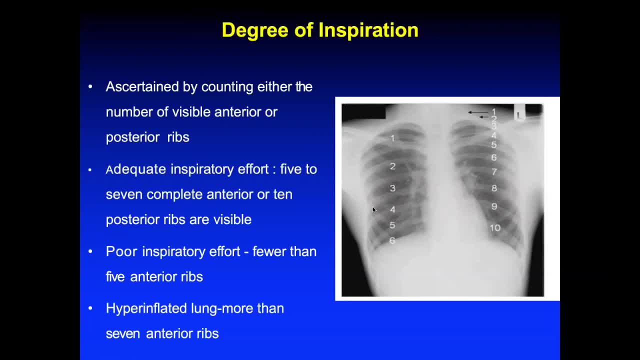 calling it a good inspiratory effort. now, poor inspiratory effort is less than 5 anterior ribs. so if there are 5 anterior ribs are not visible, it's a poorly inspiratory film. hyperinflated is more than 7 anterior ribs in the mid clavicle, like just six and a half or some places mention. 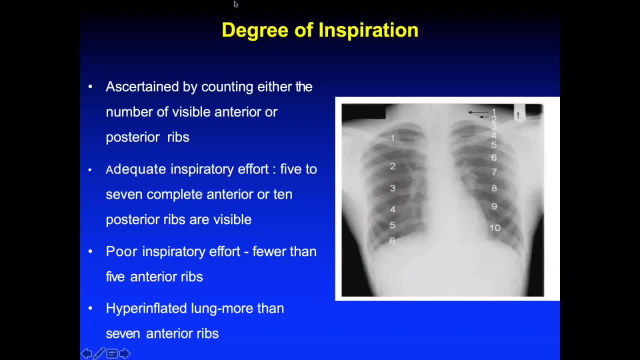 a six and a half anterior you in the mid clavicle line, or you can always just remember as seven ribs which are present in the mid clavicle line. so this is very simple way where you can count the ribs and whenever you have counted the ribs, either anterior or posterior, you can say that inspiration now why we are more. 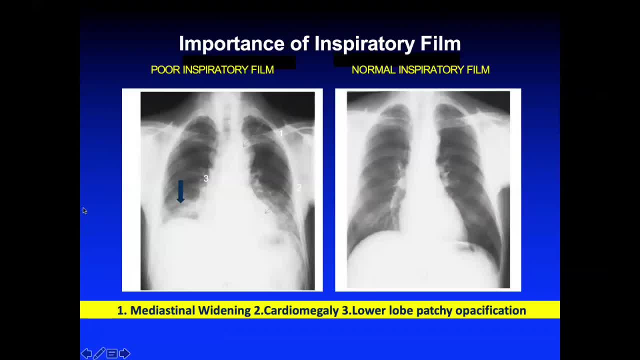 worried about the inspiration. just see this x-ray. so here you will have the first rib, the second rib, the third and the fourth rib. so only four ribs are present anteriorly. so what you have: an appearance that there is some amount of cardiomegaly is there. there is right lower. 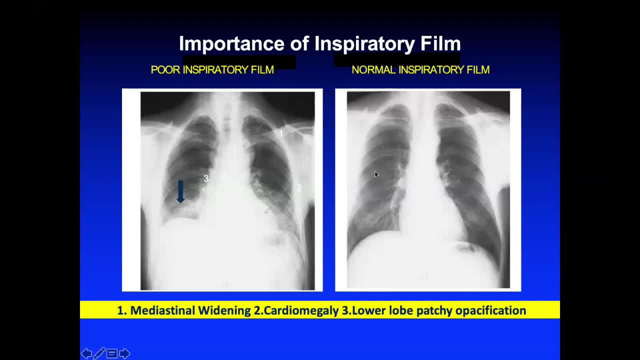 zone. haziness is there. the same person was asked to take a deep inspiration and you can see a one, two, three, four, five, six. so six slaves are coming anteriorly and this opacity disappears. the cardiac size become normal again. the left lower zone opacity also disappears. so this is very important. 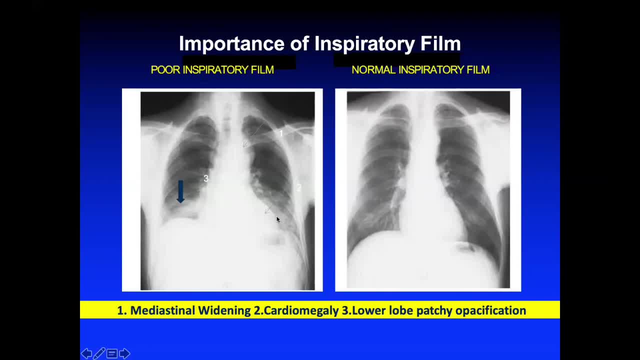 the same person was diagnosed initially as a k2, bilateral lowers or pneumonia or a lower zone haziness with apparent cardiomegaly or with cardiomegaly, and the same x-ray if it was repeated. so this is coming out to be normal. so, uh, you can see we are going to use that same x-ray here if we. 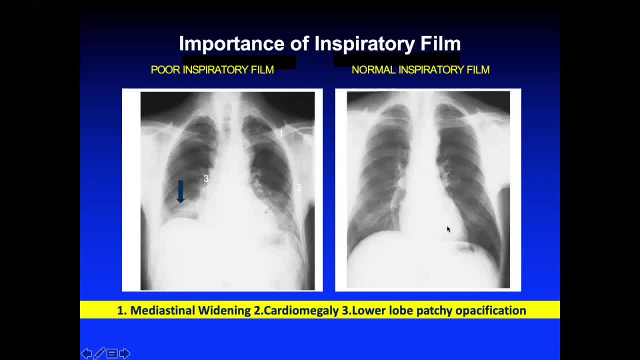 have to repeat the same x-ray. let's get see when we repeat this. okay, let's just begin with this. replay exams also. sometimes you are given a spotters, you are given the same x-ray and then you are asked that, okay, what could be the possibility? and then you keep on describing the differential and that. 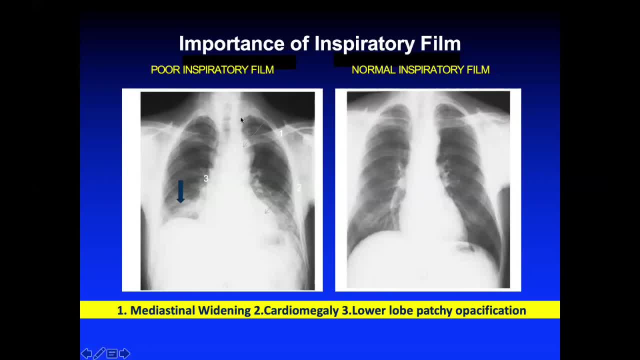 differential without looking at whether it's an inspiratory film or an expiratory film and what is the degree of inspiration. so this is very important. so mediastinal whitening, apparent cardiomegaly and bilateral zoological haziness that disappears on a normal inspiratory film. 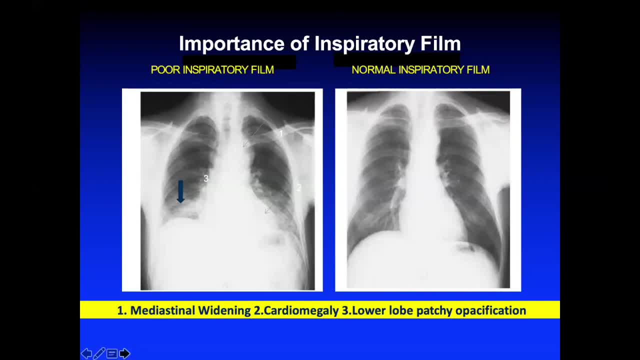 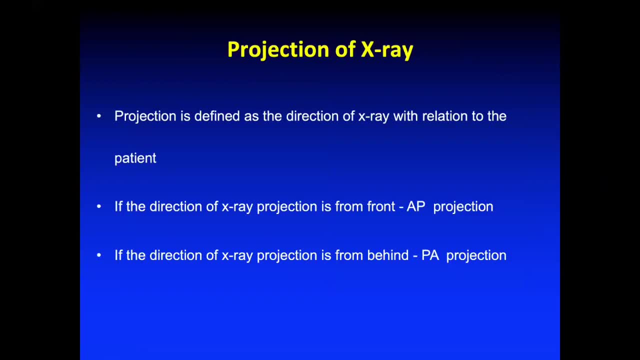 so one should be very careful when you are interpreting these x-rays. next is the projection of the x-ray. so you have to always describe in your exams also that, whether the x-ray is an ap view or in a pa view, mostly in a critical care setup, whatever x-rays, if they're given or if 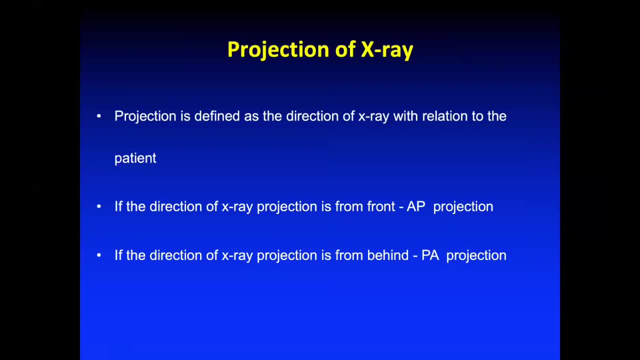 you're taking uh given some critical care, or like an x-ray from the ccu or from the icu, you'll always have an ap projection because the patient is critically ill, patient cannot stand, patient cannot uh face uh the plates. the plates are just kept below the uh body of the patient and the 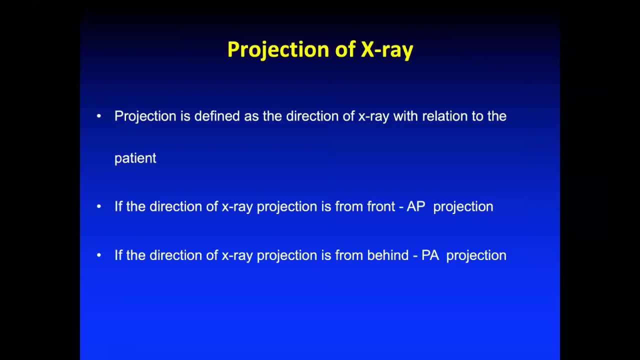 images are protected, uh, from the anterior aspect. so that is an ap projection, so that the direction of execution from front, that is called the x-ray. so you have to always describe in your exams also that, whether the x-ray is an ap view, AP projection, if the direction of x-ray projection is from behind, that is, from the back, the x-rays. 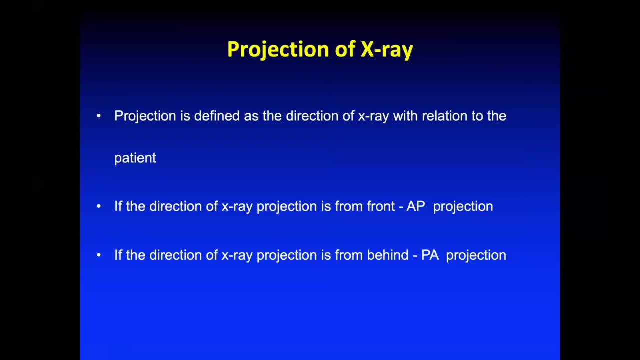 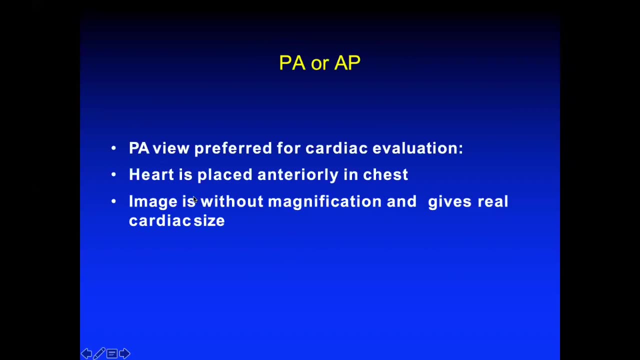 are going and the film of the plate is placed anteriorly, close to your sternum or chest. that's the PA projection. so this is the basics. so which view to use for cardiac evaluation, PA or AP? PA is preferred for cardiac evaluation. you know why? because heart is placed anteriorly. so whenever 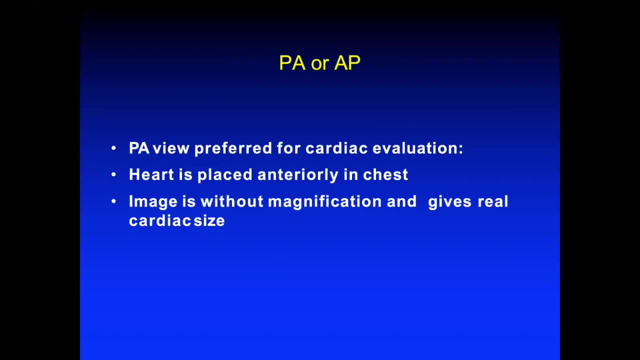 you are having a AP view, there is an apparent cardiomegaly. why? because there is an image magnification. so when you have a PA view, image is without magnification and gives the real cardiac size so apparent cardiomegaly is very problem with AP views and especially when you are evaluating. 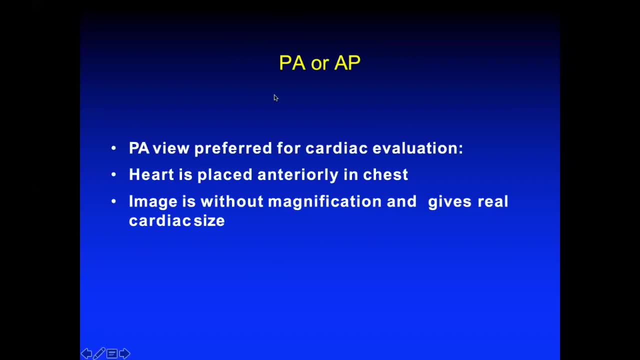 patients in a critical care setup. so whenever- never comment on, you know cardiomegaly- whenever you are evaluating an x-ray in a critical care setup, especially, you are given a PA film. so that is, and a very important point, when you are given a PA film rather than AP film. now one important: 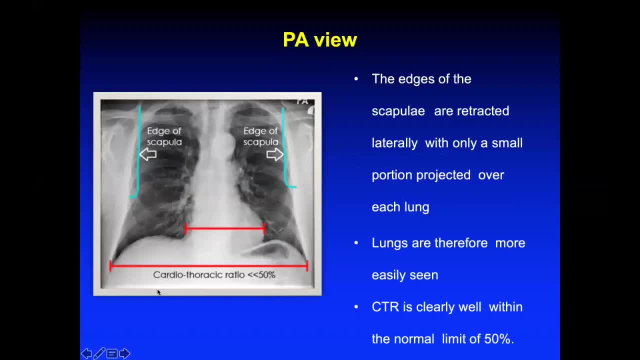 point. more to be added always: how do you evaluate for a PA view or whether it's an AP view? so how do you say basic rules are there now, if you are having a PA view, the edges of the scapula, that is, the medial edges of scapula, out of the lung field, so they should not be there within the lung fields. so 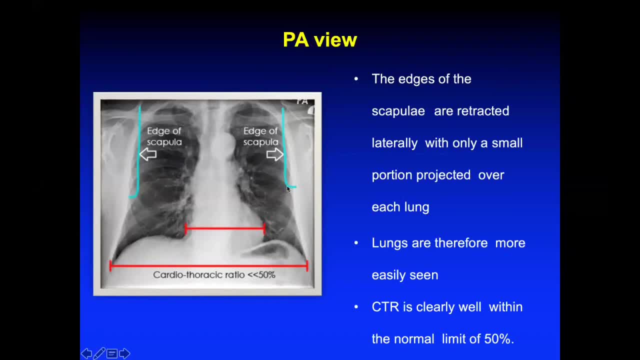 they're out of the lung fields as compared to AP view, where these are within the lung field. so all the AP views the scapula edges are within the lung fields. first thing, the clavicle is more horizontal in a PA view as compared to an AP view. clavicles are more oblique in an AP view, so the 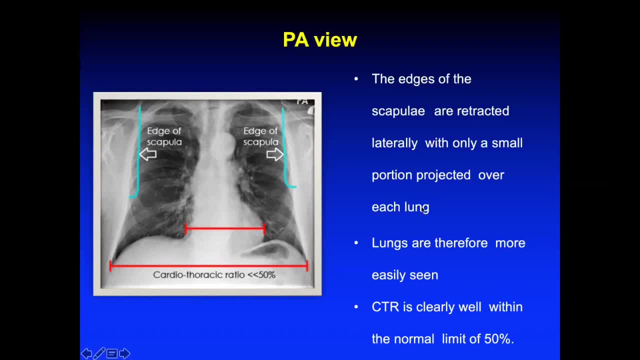 edges of scapula retracted laterally with a small portion projected over each lung. so lungs fields. you can easily visualize the lung fields clearly in a PA view and there is no cardiomegaly. the cardiothoracic ratio in a normal individual will be less than 50 percent. so 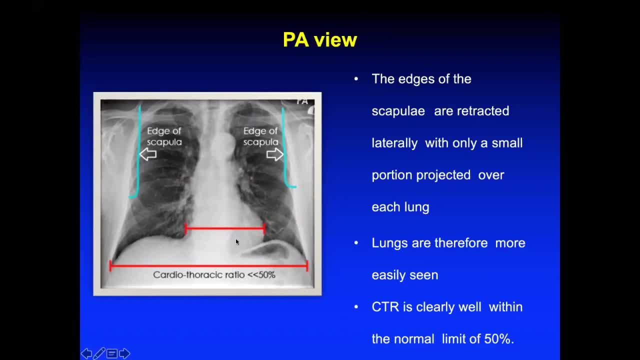 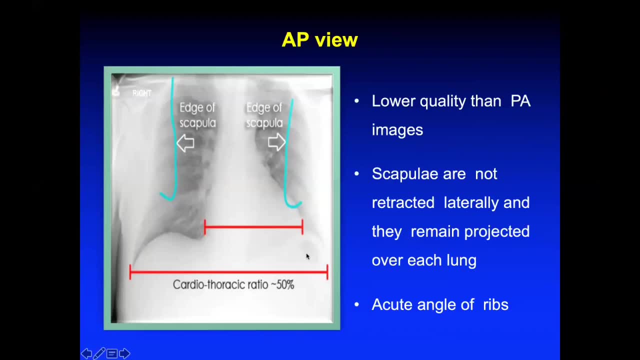 cardiothoracic ratio is clearly well within the normal limit of 50 percent. this is basically a description of a PA view, while on the AP view you know what you have is a cardiomegaly which seems like CT ratio is more than 50 percent and the edges of scapula are within the lung fields. 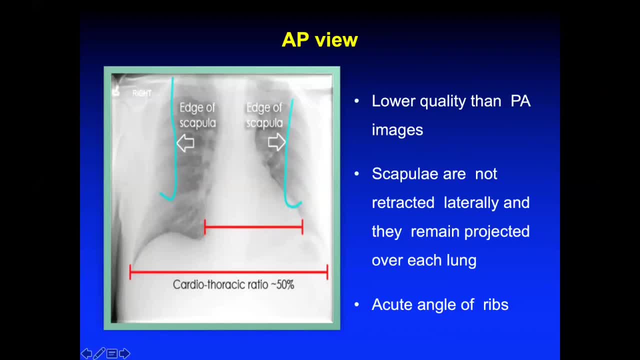 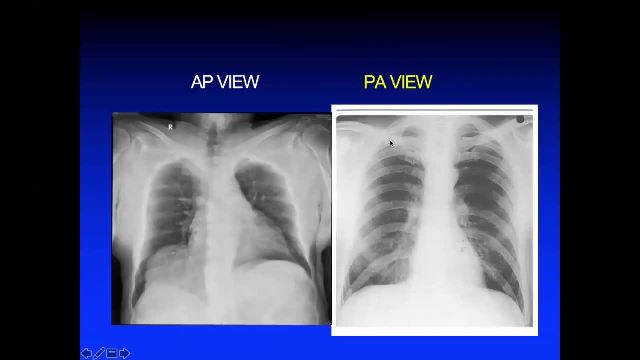 and the clavicles are always, always they are obliquely placed with an acute angle of the ribs. that is an AP view and we can see that with this example we have bed loss. this is the most simple example. this is an AP view and this is a PA. just look into the edges of the clavicle: the 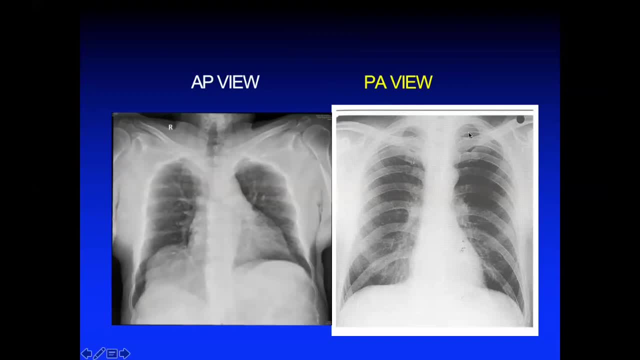 clavicles are within the lung fields. as compared to this, the clavicle's out of the lung field. they're not. the lonfish are clear first. second would be the this, the scapula. sorry, the clavicles are more oblique, where here the clients are more horizontal. the scapular is out of the lung fields. 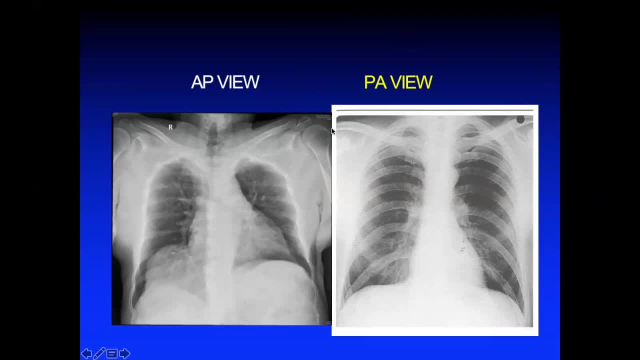 within the lung fields and out of the lung field, and the clavicles are more oblique. the clavicles are more horizontal. so this is the sound example. a, depending on your side, they are very similar to two basic differences: when you are making and uh the same person. when you are doing the same uh. 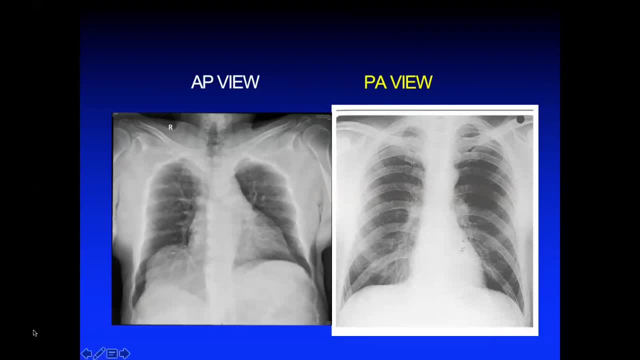 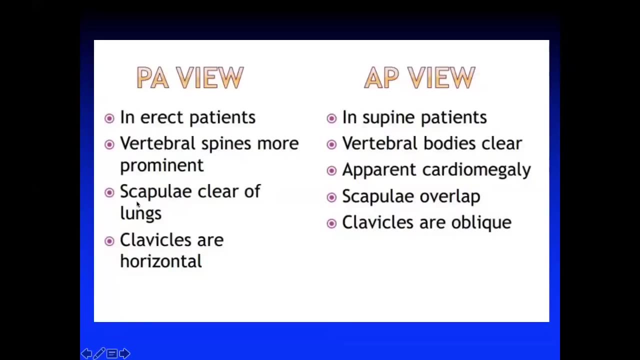 uh, this, uh cardiomegaly will be present in apu. that will disappear in the pab. so same in a pa view, the erect is the erect patient. the vertebral spines are more prominent, scapular, clear of lung fields, clavicles are horizontal, while vertebral bodies appear more clear, the apparent cardiomegaly. 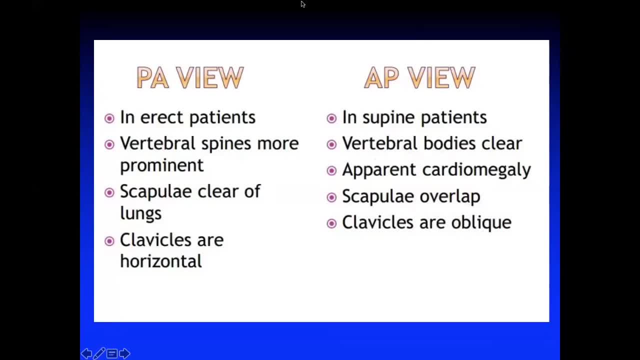 scapula overlap and the clavicles are oblique. so these are the differences. in exam you might be asked to initiate the differences. someone will ask in an examiner: what is the difference between a pa view and an ap rule? so one should be clear that these are the basic differences and one 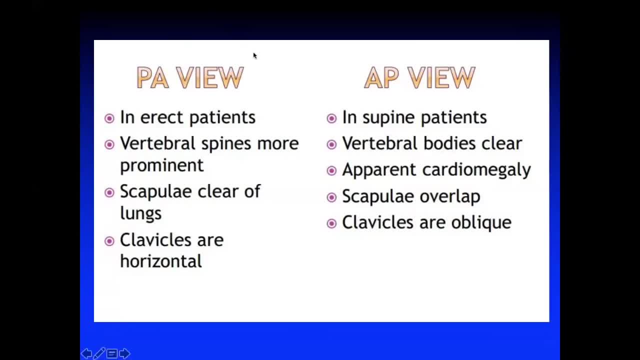 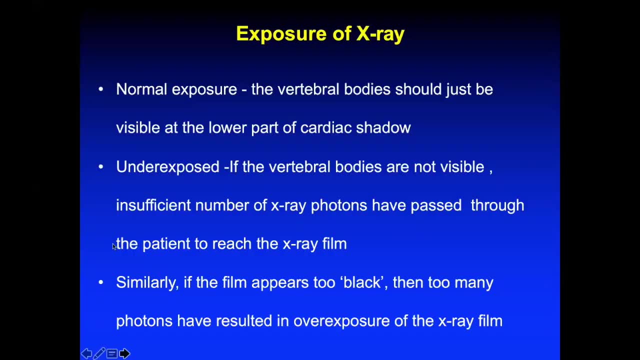 should be always uh. whenever you're interpreting the x-rays also just try to look. most of the x-rays it's just mentioned as pa and ap. if it's not mentioned, then you have to use a clinical judgment. first thing then would be the exposure again uh. the last technical quality is that uh. 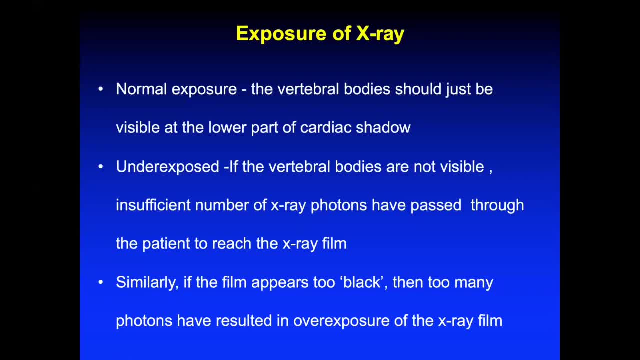 you should always evaluate for the exposure. so how do you say the x-ray is not normally exposed? so the normal exposure is that vertebral body should just be visible at the lower end of the cardiac shadow, that is, whenever there is a cardiac shadow within the cardiac margins. 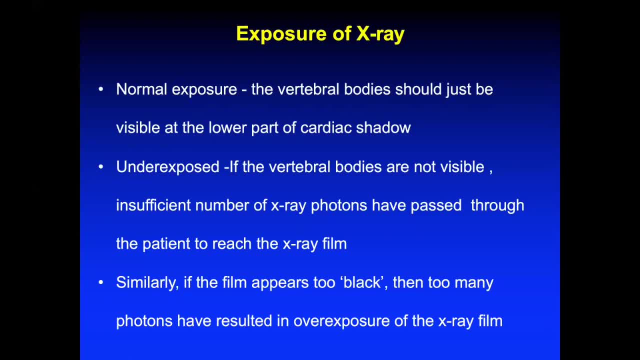 that is within the cardiac heart shadow, the vertebral body should just barely be visible. so if it's an underexposed, the vertebral bodies are not visible. insufficient number of x-ray photons are passed through the patient to reach the film, and it is not too much of white, uh, the. 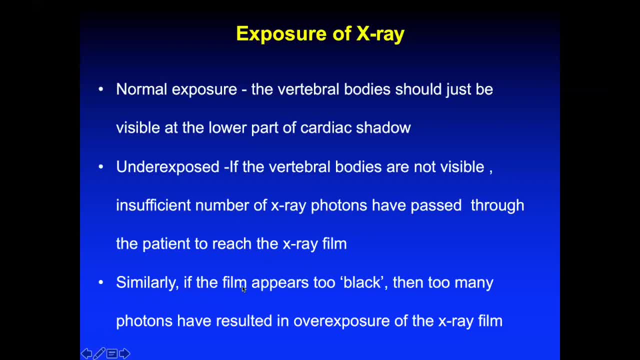 x-ray is very much whitish appearing. that's underexposed. if the x-ray film appears too black, a little too dark, then there are too many photons. they entered over exposure of the film. so here these are the vertebral bodies and the vertebral spaces. the discs should be just barely. 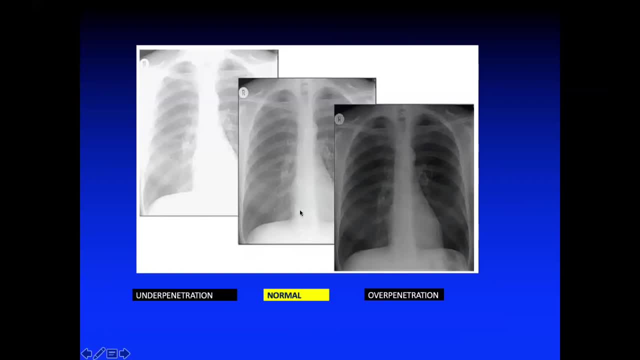 be visible. so here you can see the intervertebral spaces. the discs are just barely visible in the lower end, that is, uh below the bifurcation of the trachea. so after the level of carina, just in the lower part of the cardiac field, these should be barely visible. now, if you are seeing it here, you. 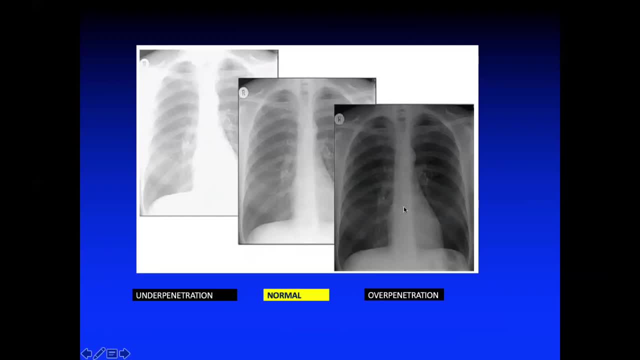 can see the vertebral body. you cannot visualize any intervertebral disc spaces, but here, if you're looking, there are too many vertebral bodies. you can see all the vertebral bodies from starting from up to bottom. so this is again. an over penetrated. x-ray is looking too dark these. 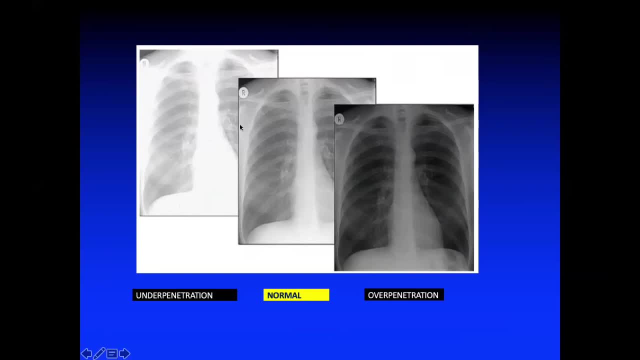 are all the excess of same individual. this is a normal penetration and this is what is called as an under penetrated film. so under penetration, normal penetration, and over penetration, so the same x-ray. so this is very important why? because whenever you have an under penetrated film, you 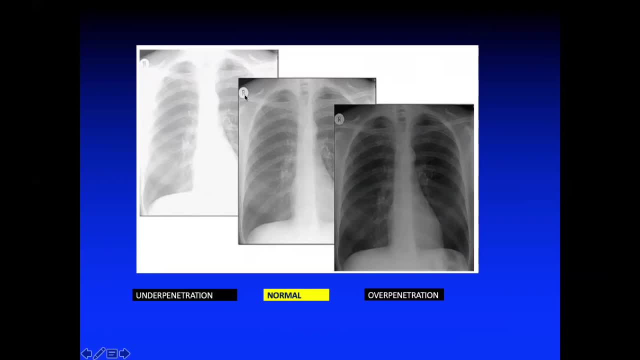 can apparently make out that there can be some opacities and you can force the label those normal, and whether you have sometimes over penetration. you can falsely mix up consolidation. you can falsely miss up, uh, you know, pulmonary edema. these things can be mixed up, or even the 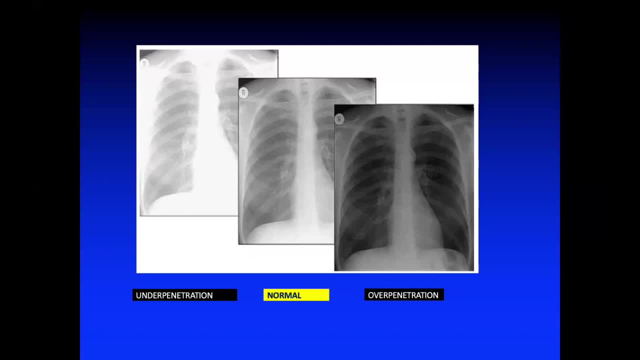 vascularity would be very difficult to comment that you can surely label that the load decrease vascularity. so whenever you are evaluating a suppose a congenital x-ray, and you are given a film and it's an open, integrated film- and you say that the vascularity is very poor or under, 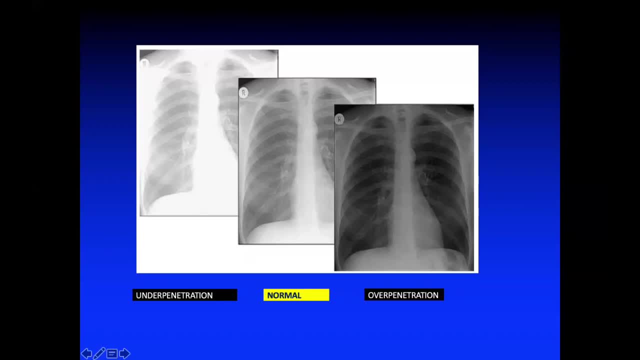 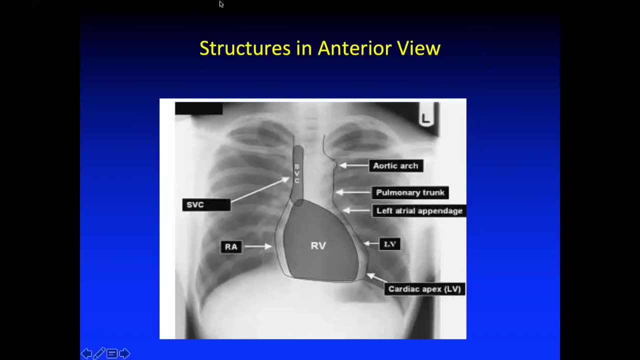 penetrated film you can see that's a abundant vascularity is there. this is again very important whenever you're doing a technical. so after you've done a technical evaluation, let's see very important- that what are the structures in a normal x-ray which are given to you a pa view? this is again the second important question is asked in the exam. 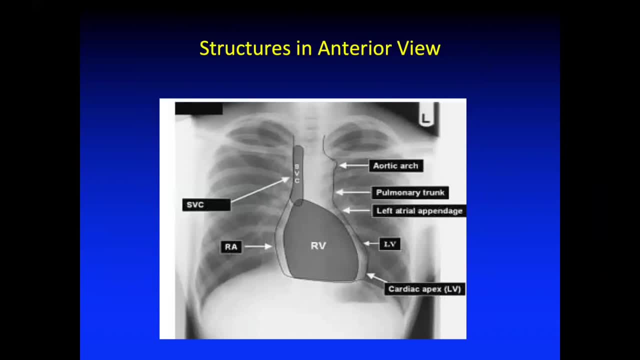 that, uh, an examiner might give you a normal x-ray and you would ask to describe what are the margins or what are the structures forming the cardiac margin. that is the right cardiac margin, the left cardiac margin. so this is very important. so this is what a normal uh one. 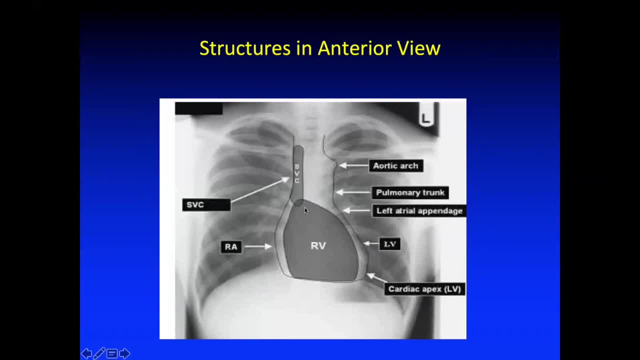 should have this image in mind. svc is on the uppermost aspect. then you have the border formed right border generally formed by the svc ra and some amount of ivc. if it appears or not, right ventricle is never a part of a cardiac margin. that is right cardiac margin or left. 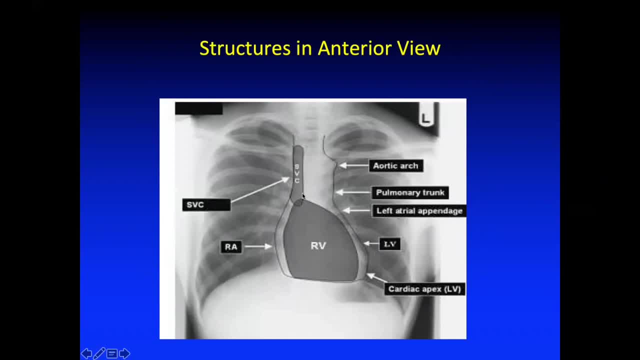 cardiac margin. right ventricle never forms, so right ventricle is in the center part of the x-ray film, so it's forming a central portion x-ray film and so is the left atrium. so left atrium sitting right here. right ventricle is sitting right here, so right ventricle will generally 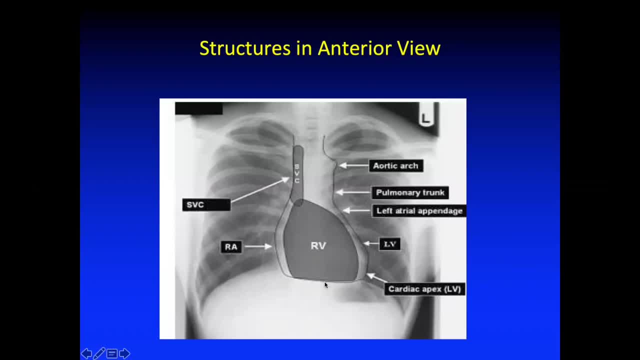 form, the inferior aspect which is sitting on a diaphragm. so this is what you're not going to describe. you're just being describing the right cardiac margin. so the right ventricle is generally the right cardiac margin, the left cardiac margin. on the left cardiac margin, generally you will have. 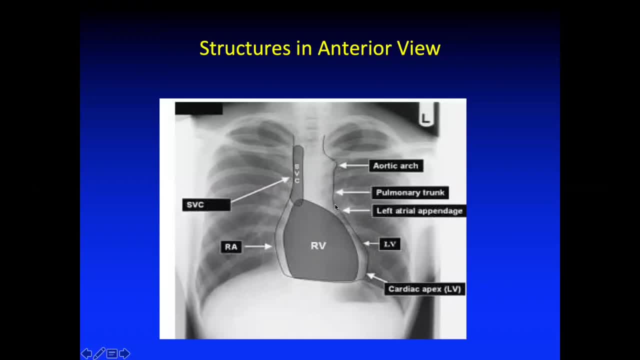 an aortic arch, the pulmonary trunk uh left atrial appendage is a part of it. so left atrium is never a part. the left auricle or the left atrial appendage is a part of the? uh left cardiac margin and then you will have the left ventricle and the cardiac effect. so this is the simplest. 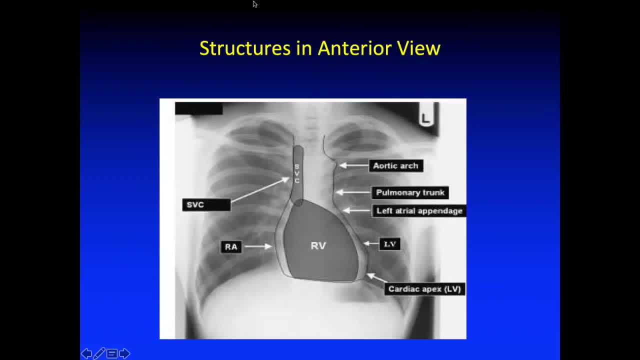 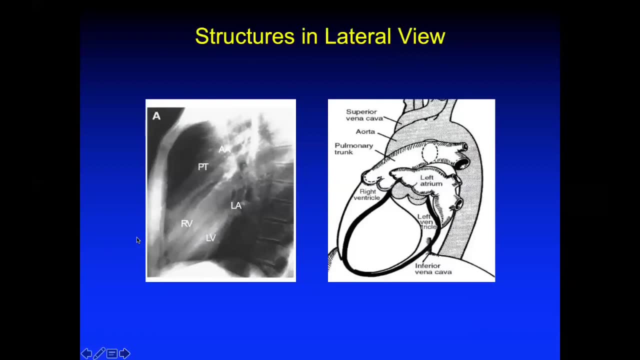 explanation or you know a basic uh what you can give in the exam for uh structures which are appearing in the anterior view, same. sometimes rarely. nowadays you are giving lateral view, but if there are some examiners, uh, they might give you a lateral view of the x-ray also. so that is. 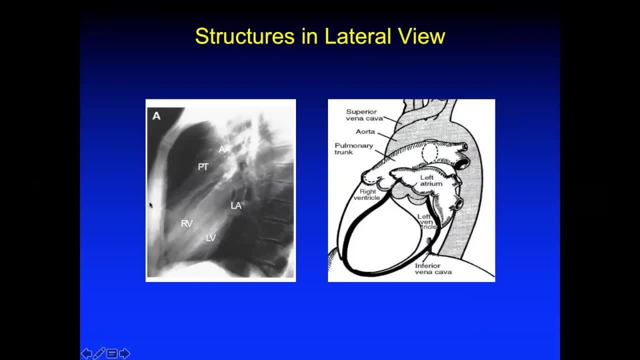 you should know that how do you approach a lateral view? in a lateral view anteriorly, this aspect is the sternum and these are the thoracic vertebrae. so this is thoracic vertebrae and this is the sternum as we move from upper end of the film to the lower end of the film. uh, the radiolucency. 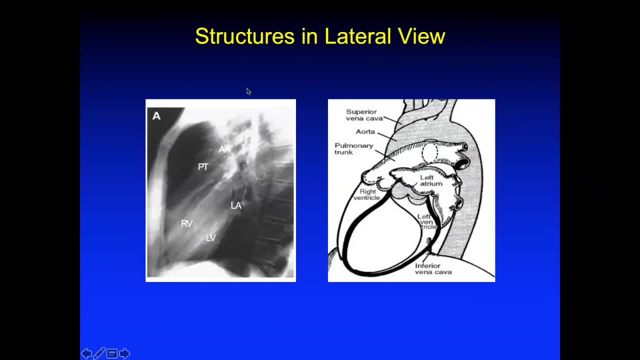 increases, that is, the lung field becomes more darker. this is because there are more air spaces in the lower lung fields. first you- this is how do you actually the anterior aspect in the posterior aspect. then you can see visualize the air column which is running in the center. this is basically the trachea and this is the 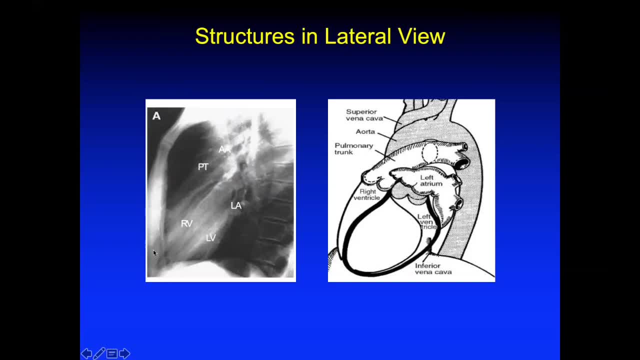 bifurcation in the main bronchi. then you have the cardiac aspect or the cardiac margin. on a lateral view you will have two ventricles which appear, one ventricle which appears anteriorly- this is basically just beneath the sternum. that is the right ventricle. so anterior aspect of a lateral 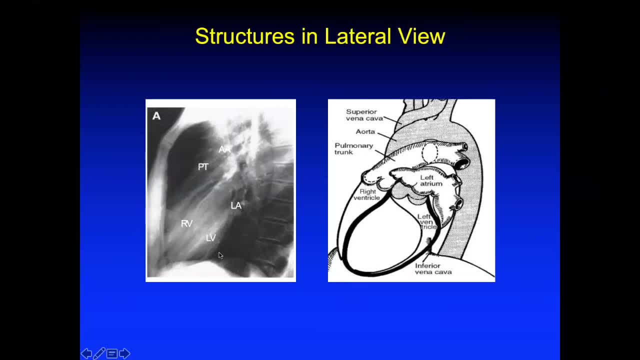 view is formed by the right ventricle. posterior aspect is formed by the left ventricle and over the top of it shapes the left atrium and then the pulmonary. just go on later in also visualization by few animations and how you do. uh see which structures for me, which view. 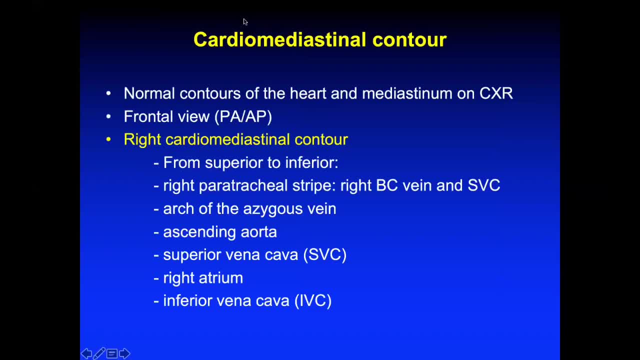 so let's see the cardiomyodastral contour. so an exam- someone will ask you to describe the technical term- is a cardiomyodastral contour. never write as right cardiac margin or left cardiac margin. just mention the right cardiomyodastral contour and the left cardiomyodastral. 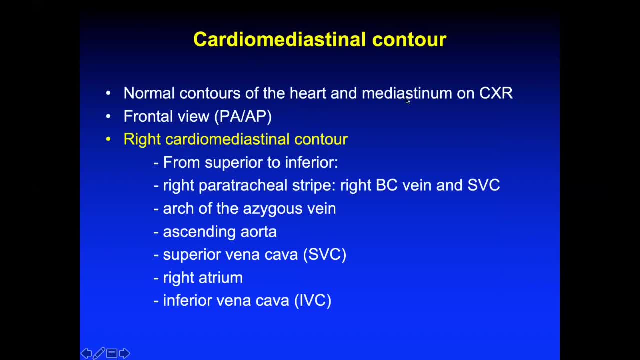 contour. so you'll have normal contours of the heart in the mediastrum, the chest x-ray frontal view. that is pure ap. that is the right cardiomyodastral contour from superior to inferior aspect. you will have a right paratracheal stripe. you have arch of azygos vein. you have ascending. 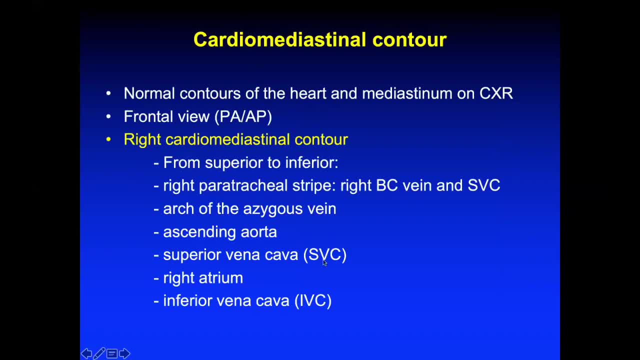 aorta, superior vena cava, right atrium and inferior vena cava. most of the x's you will always be visualizing: svc, right atrium and ivc. these might or might not be visualized, especially ascending aorta and azygos, where arch of the zygus vein, right paratracheal stripe, is always visualized. so 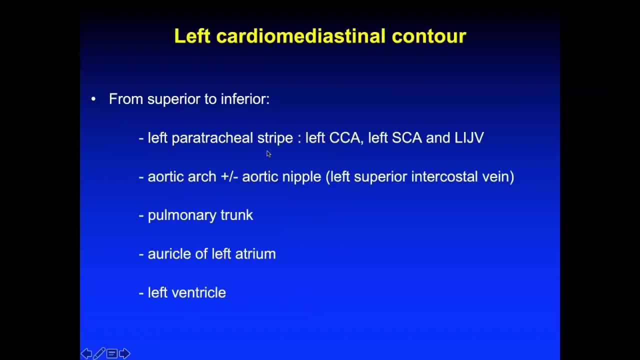 left cardiomyodastral contour from superior to inferior aspect. there is a left paratracheal stripe, then the left paratracheal stripe will include the great vessels, that is, the left common cavity artery, the left subclavian artery and the left internal jugular vein. 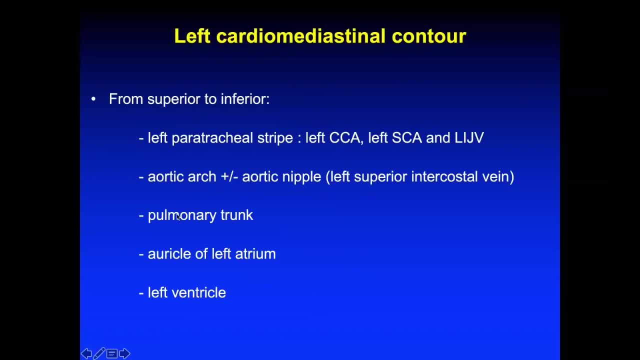 then there is the aortic arch plus minus the aortic nipple. there will be a permanent trunk. there is oracle of left ventricle, left lateral appendage as we call it, and the left ventricle which always form the apex. so this is the normal x-ray here, what you can see, the right paratracheal. 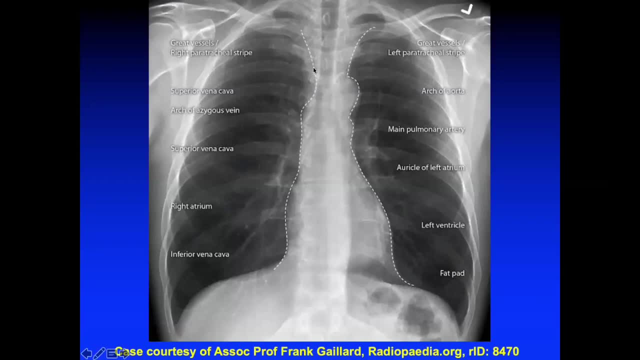 stripe that is the soft tissue around the trachea on the right side and on the left side. so the right right paratracheal stripe. on the left side it is called a left paratracheal stripe, so both of them will have great vessels. then you will have the svc, the margin of the svc. the svc will cover a. 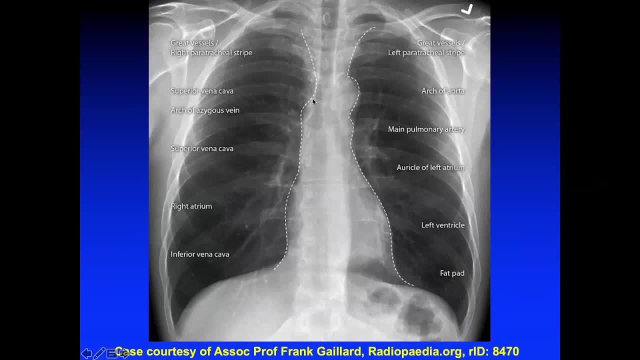 broad aspect right from the bifurcate just up to the bifurcation of the trachea. then you have the right atrium. sometimes ivc may or may not be visualized in the left lower, in the right lower aspect, but mostly it's svc and the inferior vena cava. on the left side again it's. 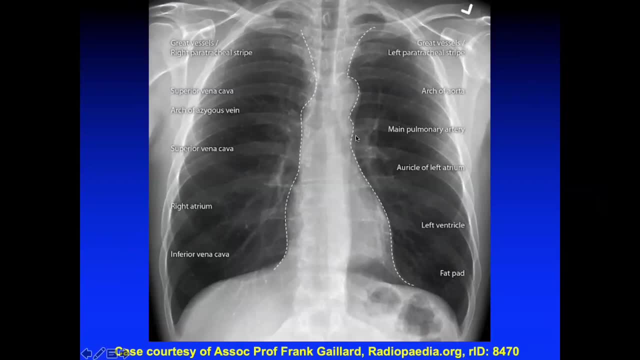 the left paratracheal stripe. this is the arch of the aorta, this is the main pulmonary artery, or we call it. then you have the auricle of the left atrium and then you will have the left ventricle. sometimes you can also have an epicidal fat of pad on a lateral view, if sometimes you are asked to. 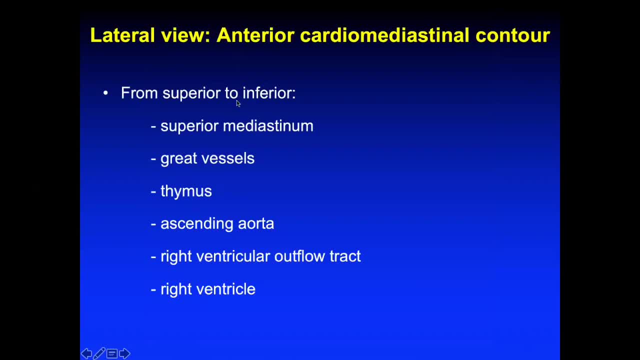 describe the anterior cardiometastatic contours. so anteriorly, as we have talked about right ventricle and right ventricle outflow track, that is, pulmonary artery, pulmonary trunk is anteriorly, on the lateral view. so superior mediastinum, great vessels, thymus, ascending aorta, right ventricular outflow tract and 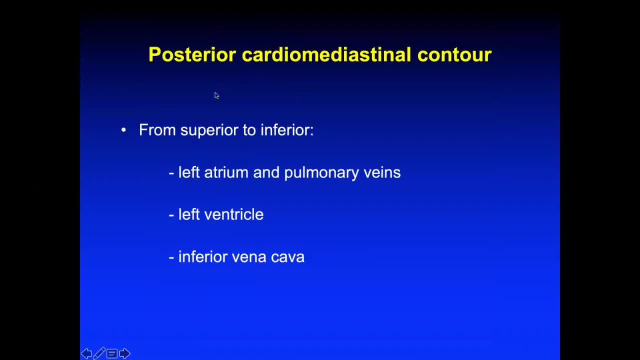 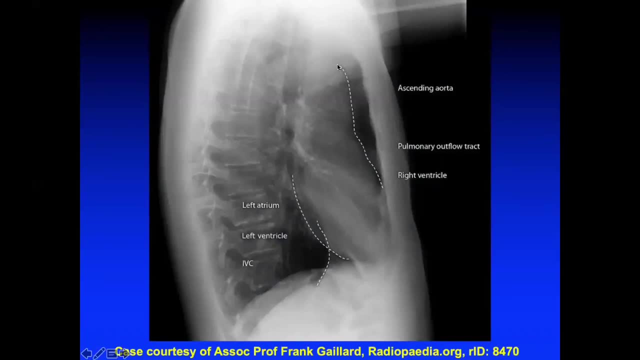 right ventricle is on the anterior aspect and on the posterior aspect you will have left atrium, left lateral view. so this is just the left uh cardiometast, the left uh lateral lateral views and the anterior cardiometastral contours. so you will have a right ventricle. this is the aspect of the right. 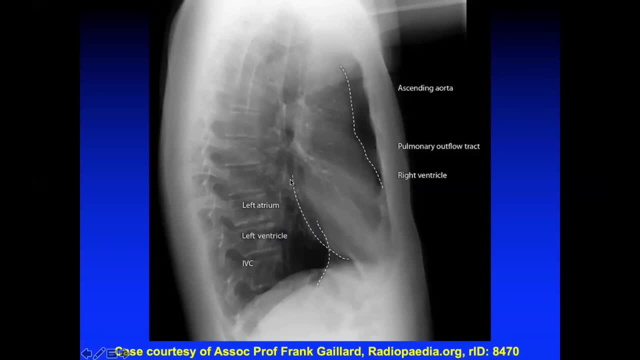 ventricle, there is a right ventricle outflow tract and pulmonary outflow tract, then you will have the left atrium. the left ventricle forms the posterior aspect and sometimes you also have an ivc which is draining. so this is the ivc which drains into the- uh, you know- right ventricle. so this is the. 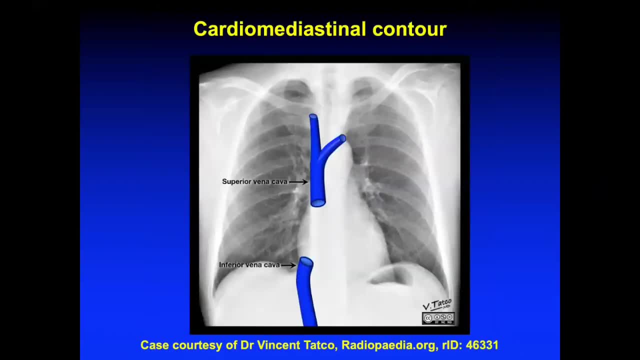 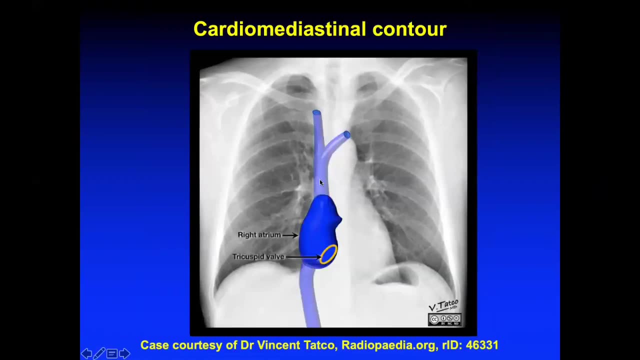 appearance on a lateral view. just see the animation. so here you can see the svc and the ivc. then you have the right atrium. so svc, right atrium, ivc will form with the right cardiometastinal contour. always remember: tricuspid valve is obliquely placed. the tricuspid valve is always oblique. 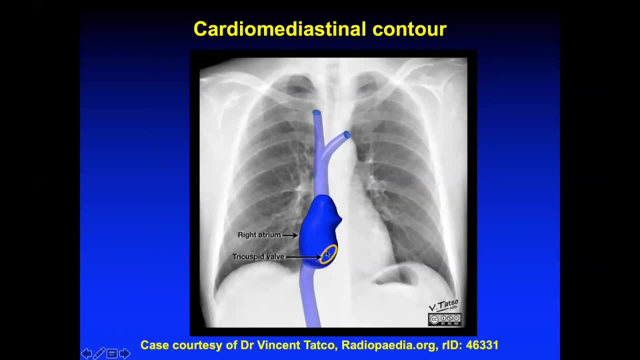 in nature. so this is a tricuspid wall which appears again. it will not appear on an x-ray view. then you have the right ventricles. the right ventricle is always in the center and this will be the tricuspid wall again, for the wall and right ventricle are not visualized normally, except when 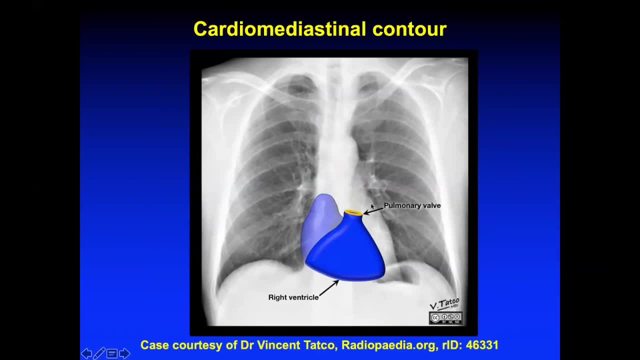 the wall is not being replaced, so the permeable has been replaced by a prosthetic ball, so you can have this permeable which also is being visualized. so this is the normal position on the probably valve. so from here the primary trunk arises. so this is the main pulmonary artery. so 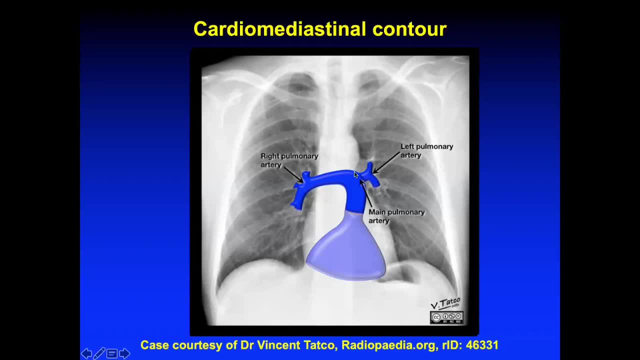 this is what it visible. this is only one. so this is the pulmonary trunk or the main primary artery. this is being visualized. then it bifurcates into left and right, so whatever is seen on the right side, this is what is called as a right atrium pulmonary artery. 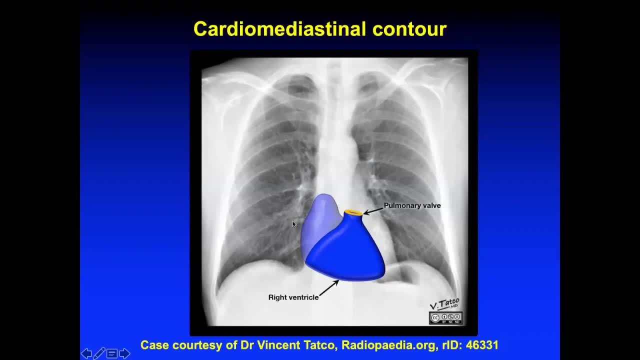 primary descending for my arteries. So this is the RPDF, the right descending for me. So this is the main type for me artery by fun kids and this which goes down. So there's a one best class structure which goes down. This is a right descending for me. Then it 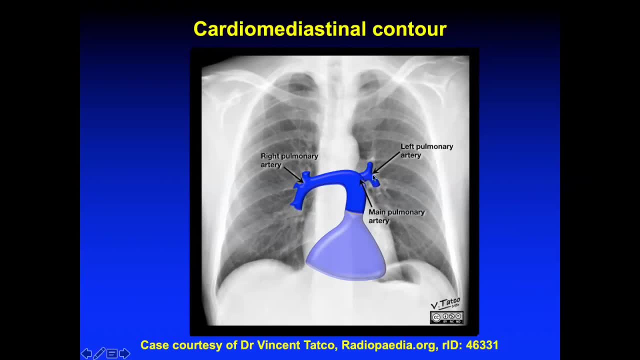 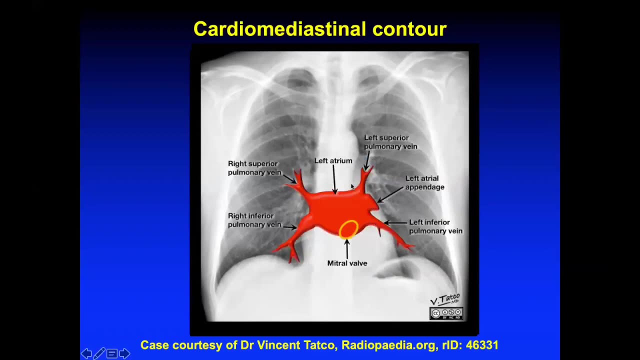 is not the right for me, It's a branch of it. That is the right descending for me. On the left side you have a left one, So this is a left for me, Left atrium. as I said that on a PAV or an APU, left atrium is never visualized because the left atrium rise at the center. 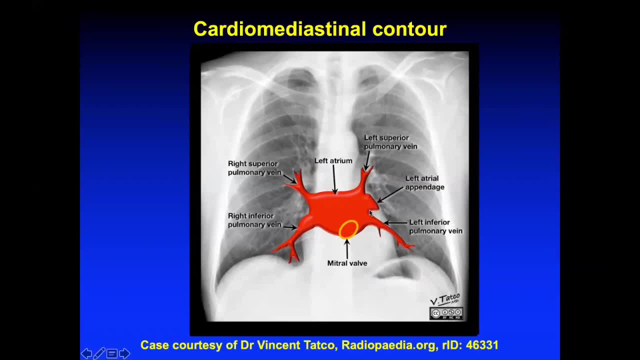 So is the mitral ball. What you are visualizing only is the left atrial appendage which forms the partial, the cardiac margin. So left atrial appendage. So this you can now visualize: that left atrial appendage is the part of the cardiac margin and not left atrium proper. 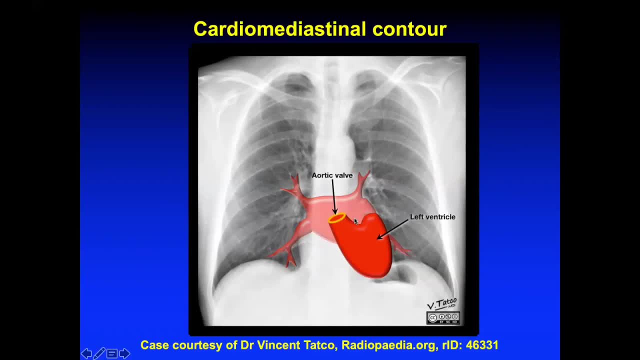 And just below the left atrium will have the aortic ball. This is the left atrium, will have the left ventricle and the aortic ball. So aortic ball, pulmonary ball, left atrium are. these are in the central aspects And later on we'll also describe how do you? 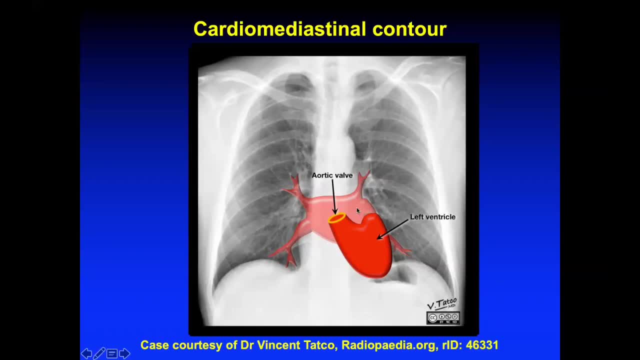 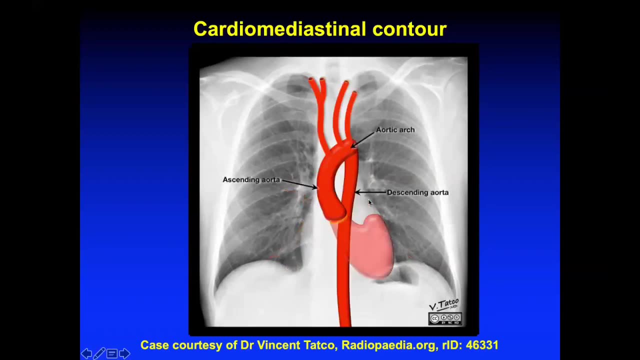 identify these balls, but generally we'll have a left atrium appendage and the left ventricle, which forms the entire left side of the cardiomyocytes, to control the lower aspect. Then you have the ascending aorta. Sometimes ascending aorta can be seen on the 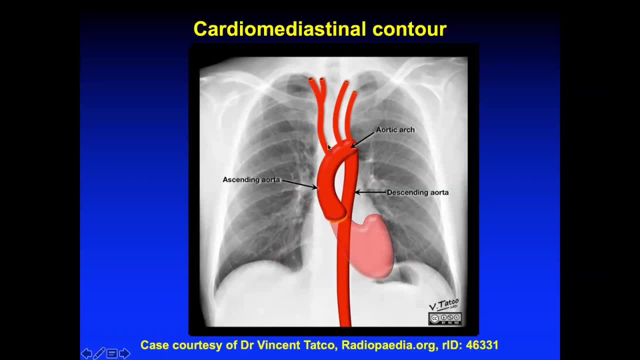 right side. So here you can see, the ascending aorta can be seen on the right side. Then you have the aortic arch and the aortic knuckles. So this you can now visualize: that aortic arch and knuckle forms the right left side and the descending aorta, The descending aorta. 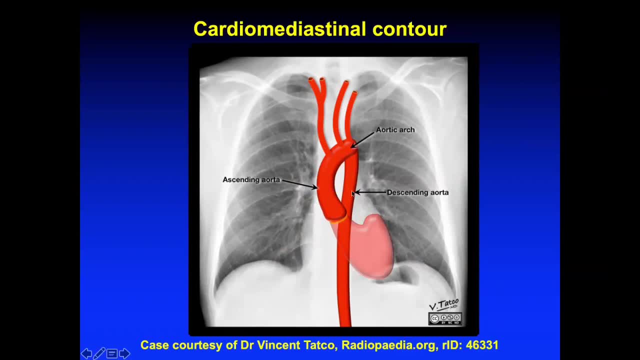 is never visualized as a part of the cardiac margin. It is always seen within the cardiac shadow, Whenever you have aneurysms sometimes, then it can be visualized. So you should know how this, normally appearing- This is a normal anatomy of various cardiac structures on an. 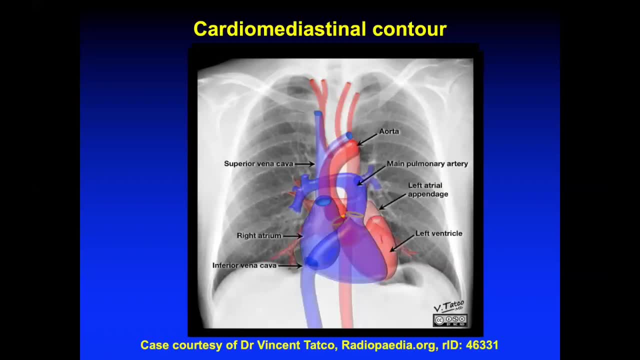 x-ray. So when you over, when you superimpose everything, this is how it appears. So you have the SVC. some types of the ascending aorta might be visualizable. You have right atrium, you have IVC. then you will have the arch of the aorta. This is the aortic knuckle. 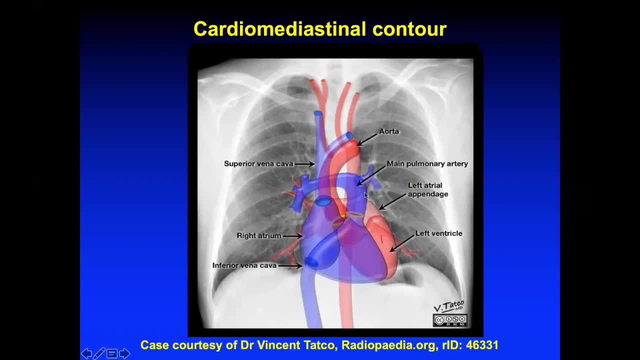 Then you will have the main pulmonary artery. So this is the main pulmonary artery, It forms a part of it. You have left atrial, atrial appendage and the left ventricle. This is the simplest way how you describe a normal x-ray, or normal x-ray which is given to you: Lateral, mediastinal. 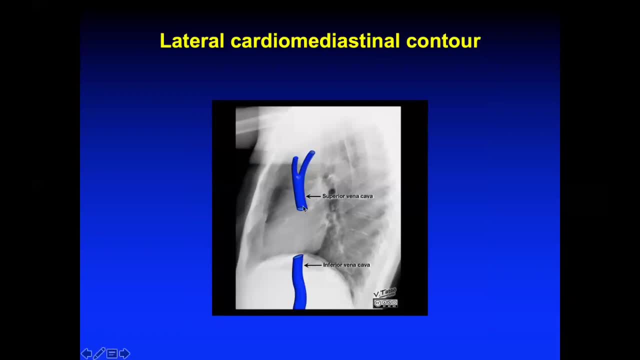 cardiomediastinal contours And you can see the superior vena cava, You can see the inferior vena cava and the right atrium. Then the tricuspid was the right ventricle. So, as I said, the 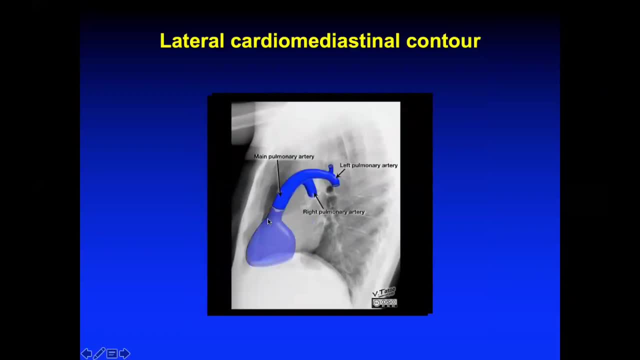 right ventricle is an anterior most structure here. From the right ventricle the pulmonary artery arises. So posteriorly, if you see on a lateral view, this is the sternum, Then you have a right ventricle and the main pulmonary artery. Posteriorly what you have is the left atrium. It aspires. 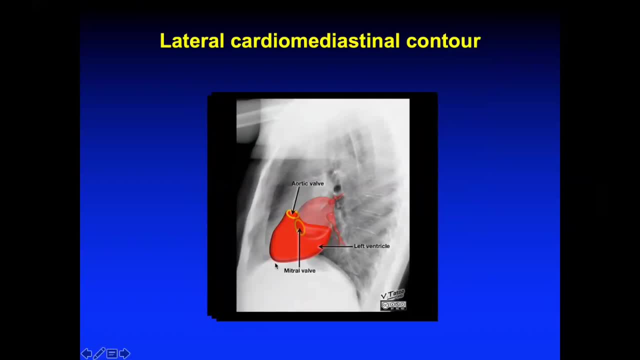 the posterior aspect and you will have the left ventricle. So left atrium and left ventricle are appearing in the posterior aspect. Right ventricle and pulmonary outflow tract are appearing on the anterior aspect And then you can see the ascending aorta. So this is. 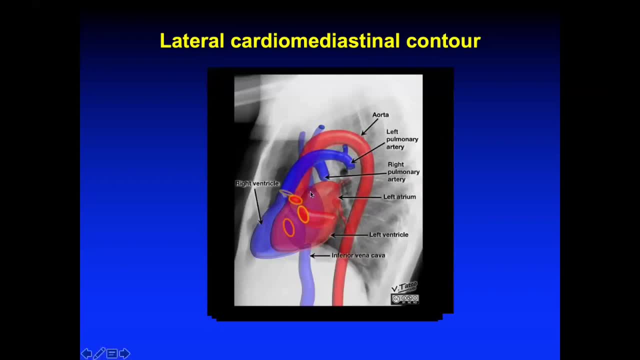 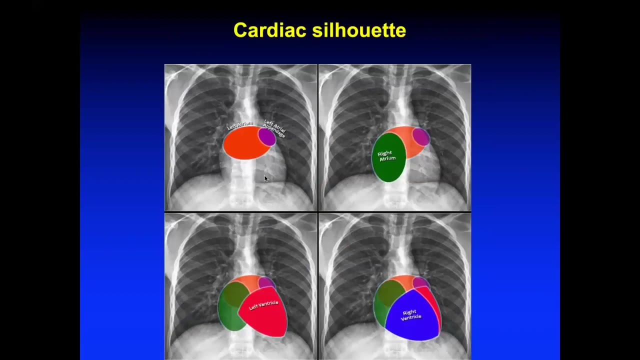 the simplified way. So right atrium generally never forms a part of the lateral cardiac margin, The posterior Spieler caudeic margin, And it's the left atrium, the left ventricle and the right ventricle and right pulmonary output tract. 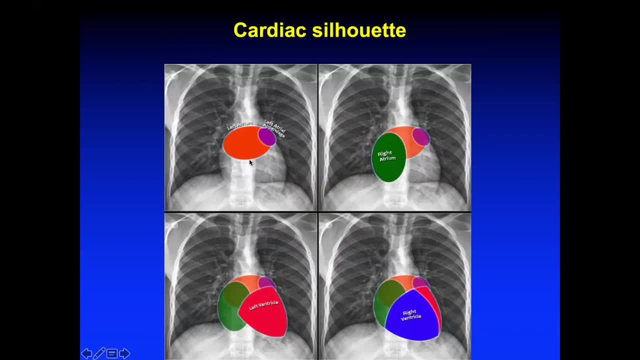 This is what is called cardiac silhouette. So at the left ependage the right atrium, left ventricle. So here you can see the right ventricle and the left atrium are never a part of the cardiac margin. So in the exam never, ever say that left atrium is a part. 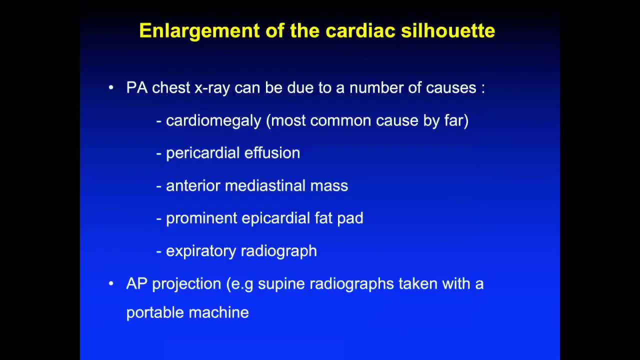 of the cardiac margin, the right ventricle and right cardiac margin. The left atrium is rare, is to the così is a mistake. So here you can see the Posterior Cardiac Vibrato and to the posterior Cardiac Ventricle. 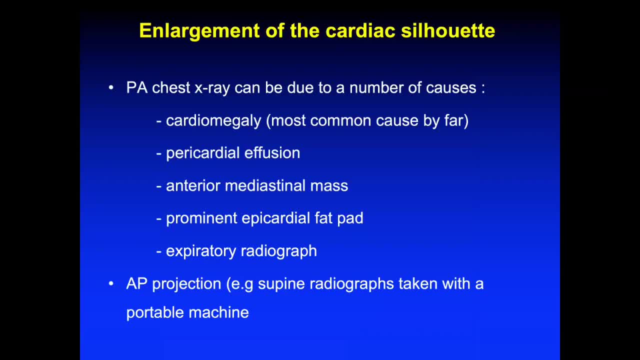 that first abnormality is an enlargement of the cardiac silhouette. that is basically called as cardiomegaly, and this is the first and foremost thing which is given in the exam is to determine what is the cardiothoracic ratio and what is the cardiac size. so pa on a phs x-ray, obviously in. 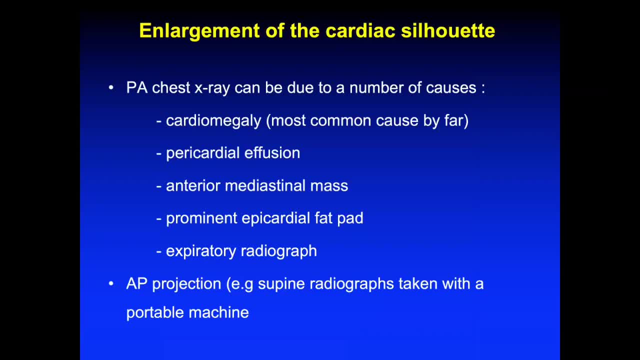 the ap view it's an apparent cardiomegaly. so most of the cardiomegalies are being reported only in a pa view. so pa view, a number of causes can be there for enlargement of cardiac silhouette. so cardiomegaly the most common cause. then there can be pericardial effusion. there can be an anti-embosomal. 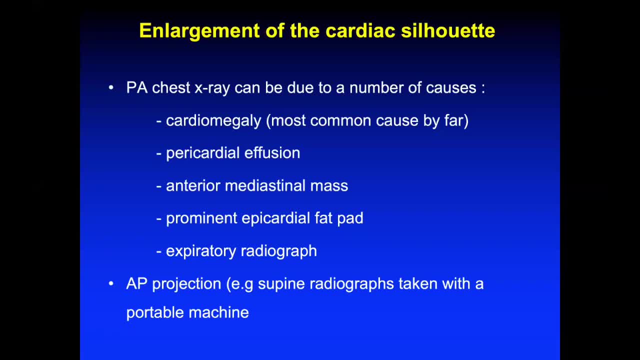 mass, there can be pericardial fat and there can be an expiratory radiograph. so if you have excluded- there is no expiratory radiograph- the four causes of a enlarged cardiac silhouette on an ap view, obviously it is an always an enlarged cardiac silhouette. so first and foremost is cardiothoracic. 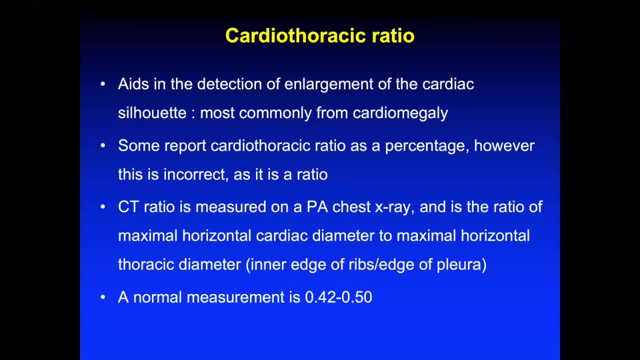 ratio, so cardiothoracic ratio, also called ctr. it aids in detection of enlargement of cardiac silhouette. that is most commonly from the cardiomegaly. so whenever there is cardiomegaly your cardiothoracic ratio increases. so how do you differentiate cardiomegaly from other causes? that is basically on the basis of cardiothoracic ratio. 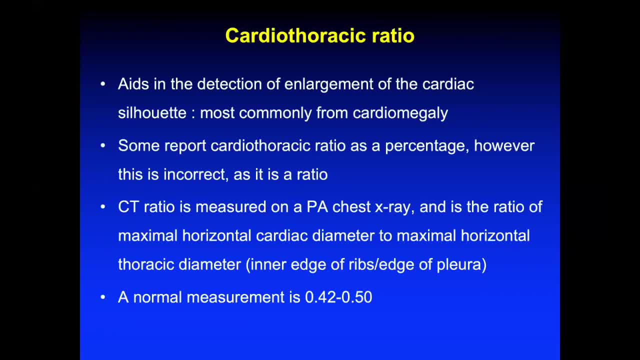 some say cardiothoracic ratio is a percentage. it's incorrect. it's always mentioned as a ratio because in the technical term it's a ratio mentioned ratio and not a percentage. so on a pa view, it is measured as the ratio of the maximum horizontal cardiac diameter to the 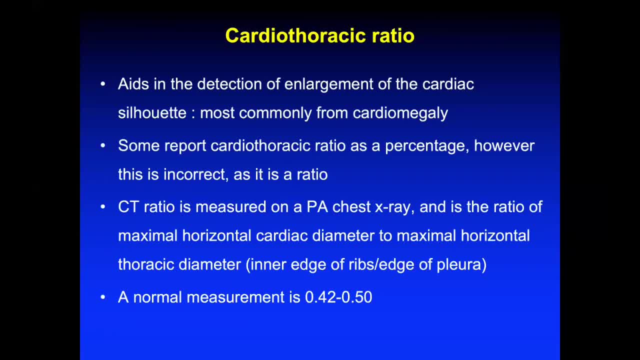 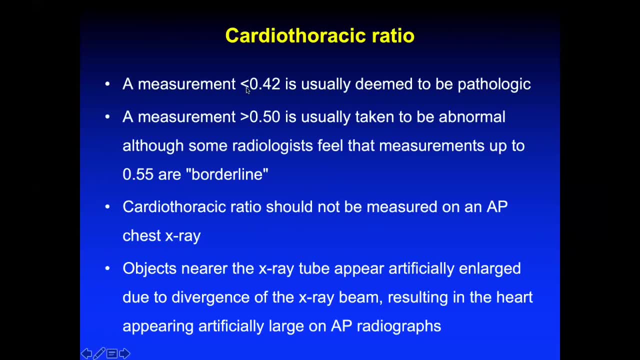 maximum thoracic diameter, inner edge of the rib or edge of the pleura. a measurement called cardiomagnetic ratio is usually deemed to be pathological. a measurement 0.50 is taken out to be abnormal somewhere you know you can see as 0.55 or 50% also should. 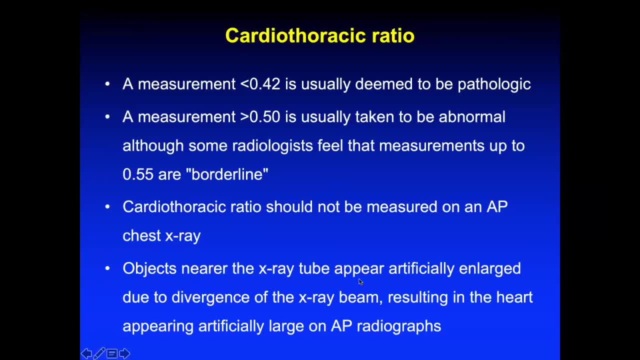 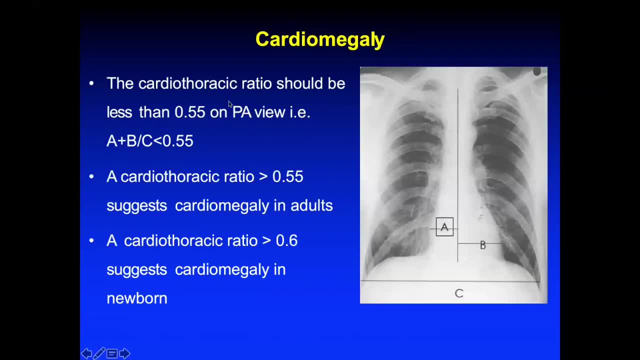 not be measured. on an ap view, so an apr view. obviously it appears as apparent cardiomegaly, so cardiothoracic ratio should be less than 0.5. on a pa view, so for our exams and all the things, the cardiothoracic ratio is usually deemed to be pathological. so for an alpha. 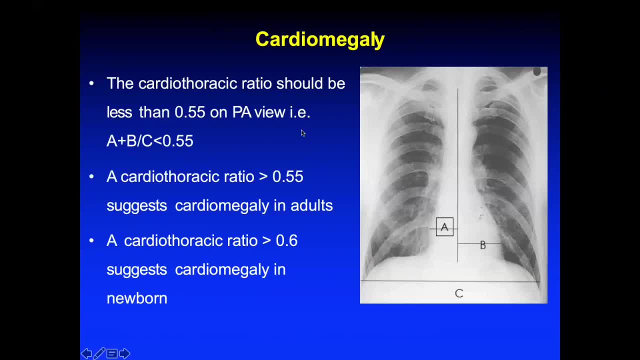 call it the therian, than you can measure it if it is a therian. so in the context of the So, a cutoff value is taken as 0.55 and this is the standard one. So all we mention is 0.55, should be less than 0.55.. 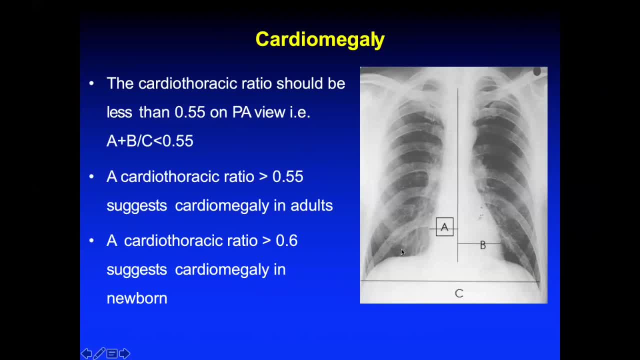 In newborns. you know 0.6 is taken as a cutoff. So how do you measure the cardiothoracic ratio? This is the most common thing which is given to an exam. So first thing would be the maximum horizontal cardiac diameter and the maximum horizontal thoracic diameter. 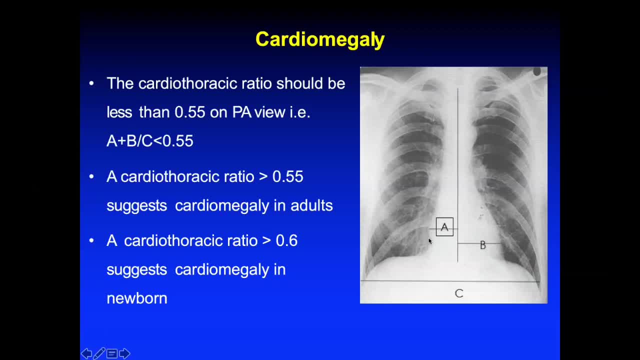 Now, mind you, the maximum horizontal cardiac diameter is not measured in the same plane. So first of all you draw a vertical line from the spinous process of all the vertebra, Then you see the right cardiac margin and the left cardiac margin. 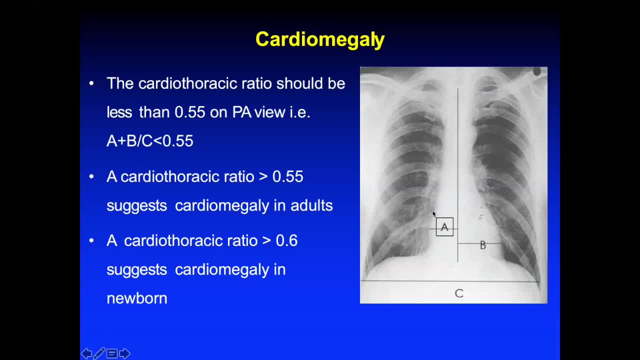 So the right cardiac margin, the maximum prominence is here. So maximum outward curvature or prominence is here. From here draw a perpendicular to the central line from the spinous process. On the left cardiac margin, the maximum prominence is here. 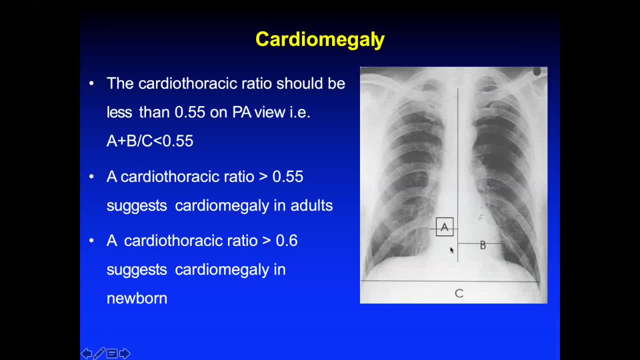 So from here you draw a perpendicular To the central margin, So that A plus B would be the maximum cardiac diameter, That is, the transverse diameter of the cardiac X-ray. Now how do you measure the thoracic diameter? maximum thoracic diameter? 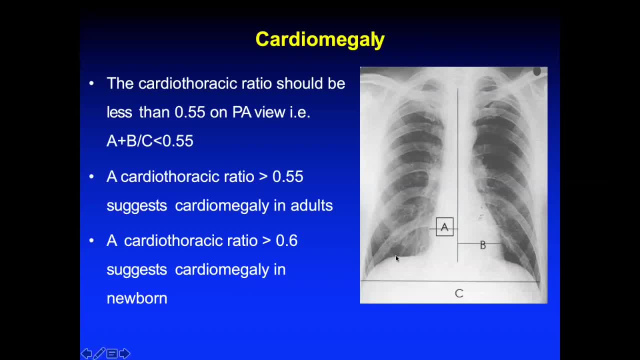 From the edge of the ribs. So you see, wherever the maximum curvature of the ribs is there, from there draw a horizontal line Edge to edge, From inner edge to inner edge, Not outer edge. So never include this outer edge of the ribs. 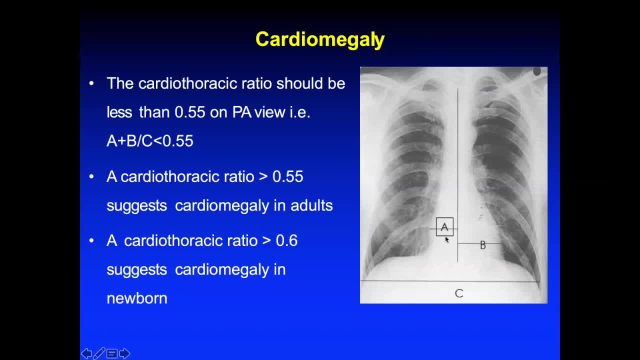 Always go for the inner edge of the ribs or the edge of the pleura. So this would be A plus B divided by C. Draw a cardiac thoracic ratio. So A plus B upon C would be. This is where you should measure a cardiac thoracic ratio. 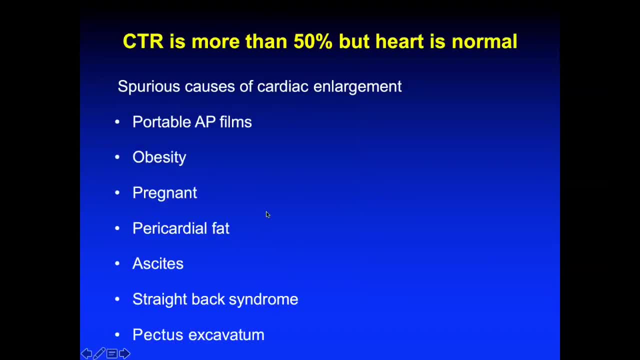 And that is what is being exercised in exams also. So sometimes your cardiac thoracic ratio is more than 50%, But heart is normal. Spurious causes can be there because of portable epiphyllum- Okay, Obesity, Pregnancy, Pericardial fat. 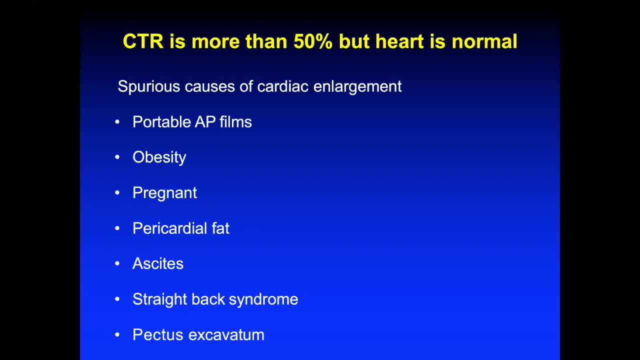 Ascites, Straight back syndrome And pectus excavatum. So again, this is a very common question asked in exams. So X-ray heart is normal, So you have a normal heart, But then the CT ratio is more than 50%. 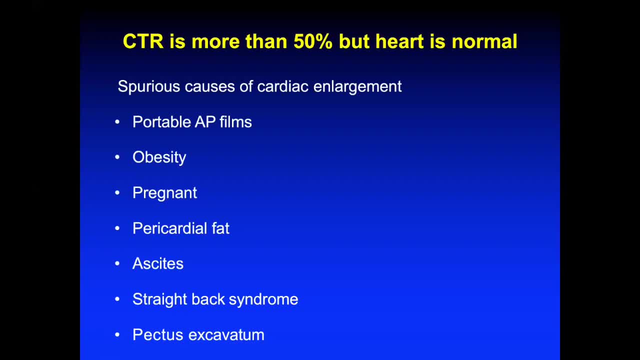 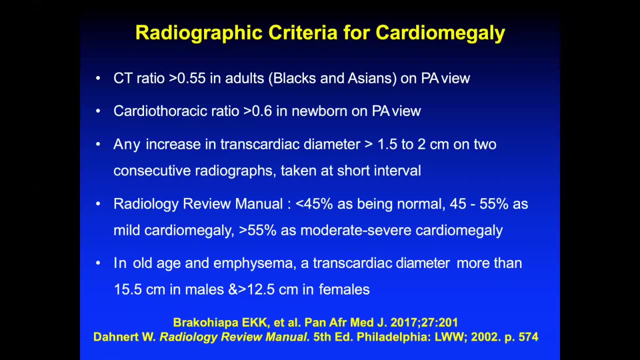 What are the references? A lot of the causes. So these are the causes of that. So, radiographic criteria for cardiomegaly. So for blacks and Asians the CT ratio should be more than 0.55.. The CT ratio more than 0.6 in newborn. 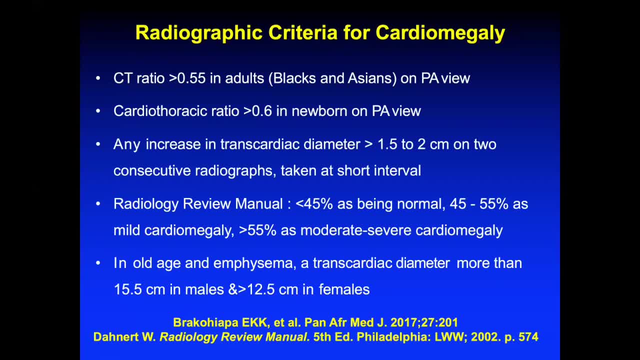 Again, this is very important. So another quite common question examiners will ask, especially, you know, the senior examiners- is that any role of a serial X-ray like? suppose you are seeing an individual today coming with a cardiac thoracic ratio of 0.44.. 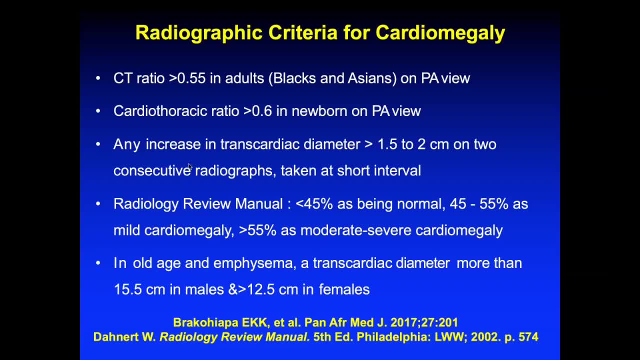 And if it is increasing over a period of time. So yes, So in any increase in transcardiac diameter of more than 1.5 to 2 cm on two consecutive radiographs taken on a short interval. this is basically, says us, abnormal. 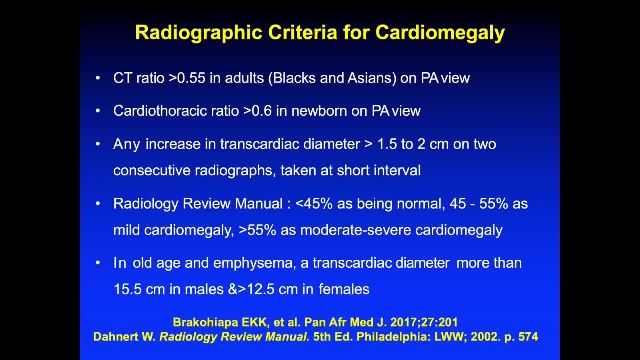 So this is what a serial X-ray also has. The CTR plays an important role. This was a study where you know they have classified as severity of cardiomegaly, But again it was for a population where they said that cardiothoracic ratio 0.44, below it is normal 0.45 to 0.55 mile and 0.55 to 0.6.. 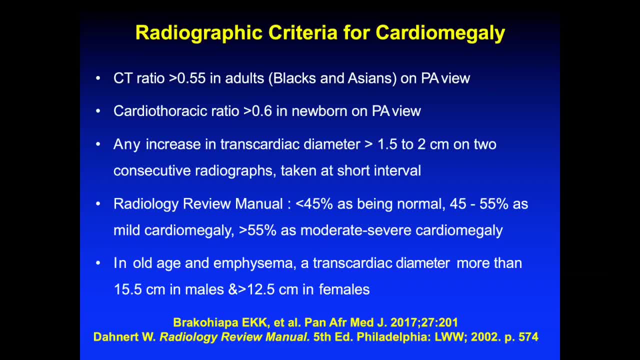 Again, for Asians this is not applicable, And only in emphysema, obviously. in an emphysema, at the slant the heart becomes tubular And a transcardiac diameter of more than 15 cm in males and 2.5 cm in females can be taken abnormally. 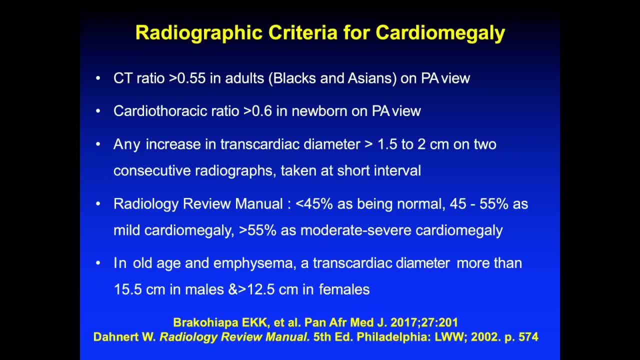 But again, these are rare things. Only thing you need to remember is 0.55 ratio more than in adults and 0.6 in newborns. This is about Asians. This is what? Another cut-off. If someone asks you that, okay, what is the severity? 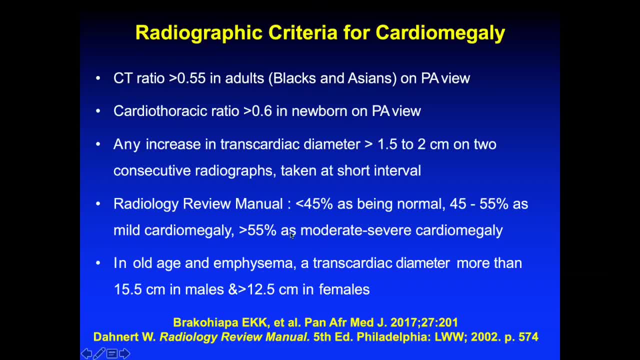 So this is the only classification I got in the literature that what is the severity? on the basis of cardiothoracic ratio can you classify the severity as being mild or moderate or severe cardiomegaly. So again a very simple example. 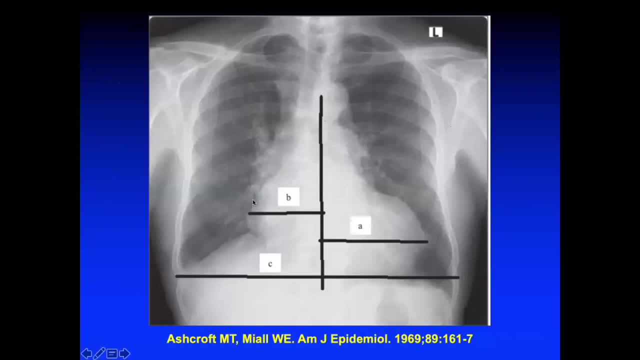 Draw a vertical line. maximum cardiac diameter from the left side, on the right side, on the left side, A plus B and the maximum thoracic diameter. So here they have just R to make the outer rim. It should always be the inner rim. 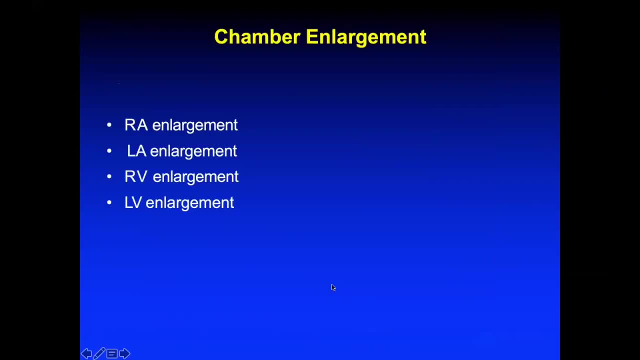 So that's it, Thank you. So once you have done a cardiomegaly, that, once you say that, okay the exam, you have found out that the CT ratio is there and you have a cardiomegaly. 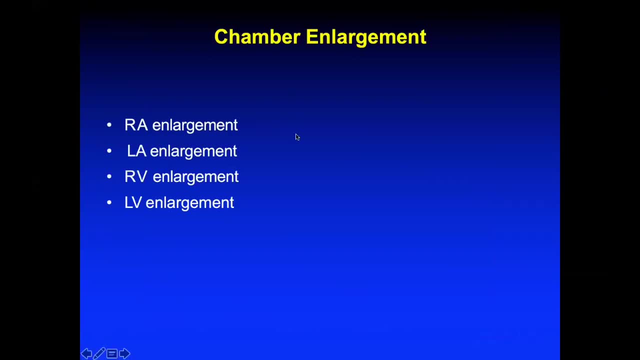 Now next thing the examiner wants: is that okay, which is the chamber being enlarged, So that what you are saying, that how you can say that it is the right atrial enlargement, or you can say it's the right ventricular enlargement or left atrial enlargement, left ventricular enlargement. 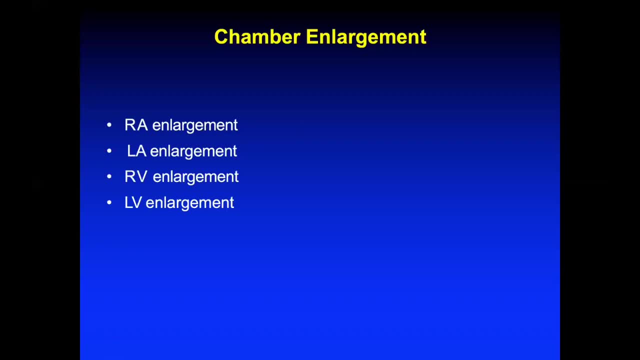 So this is again second most common question being asked in exams: How do you determine the chamber enlargement, So all the four chambers? there are some, you know, hard points. There are some criteria, So one should remember all these. 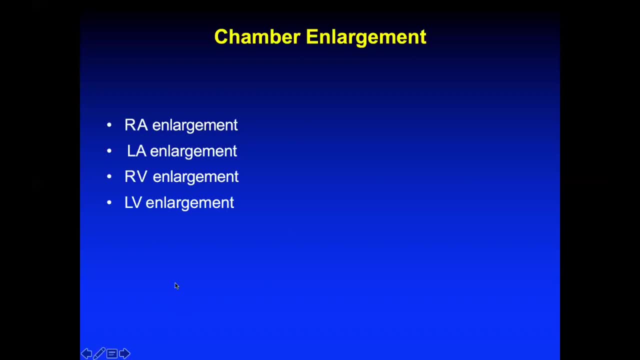 All the criteria for enlargement, Because you know why we are going on a stepwise approach is because when you are dealing with systemic disease, like suppose you have a case of mitral stenosis, you always have a left atrial enlargement. 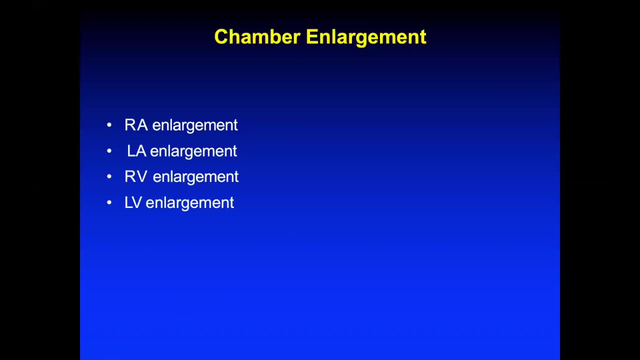 Then you will have later on, as an RA, enlargement or a case of atrial septal defect, ASD. you will be given a case of ASD. Then you will have a simple X-ray where you have a right atrial enlargement or right ventricular enlargement, or you suppose you have a case of, you know, hypertension or aortic stenosis and you will have a left ventricular enlargement. 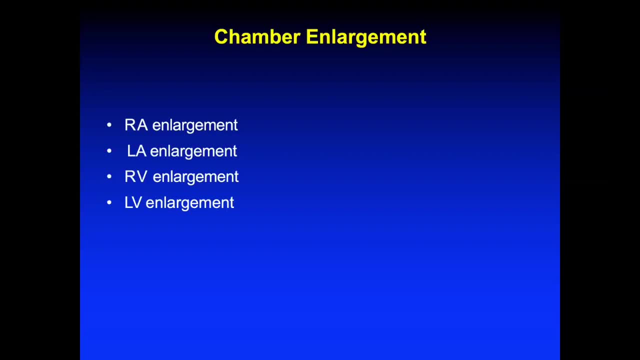 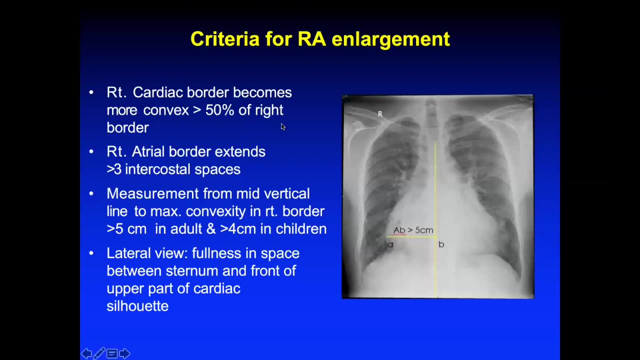 So this is basically. you should know That. how do you identify in an X-ray, What are the criteria? So let's see first criteria for right atrial enlargement. You know, when there are multiple criteria, for one thing, always remember that this is not a very hard point for a criteria. 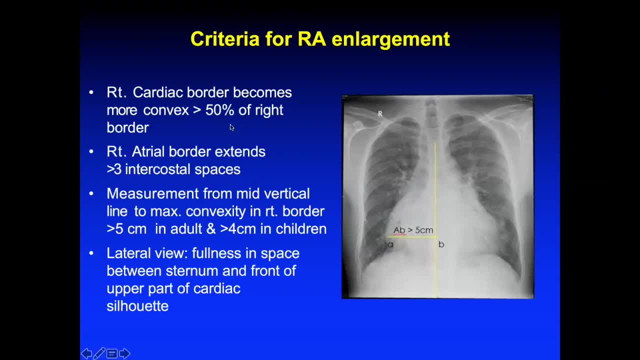 But the easiest criteria for a right atrial enlargement is right atrial border extending more than three intercostal spaces. So if your right atrial border, So this is the right atrial border If it extends for more than three intercostal one, two and three. 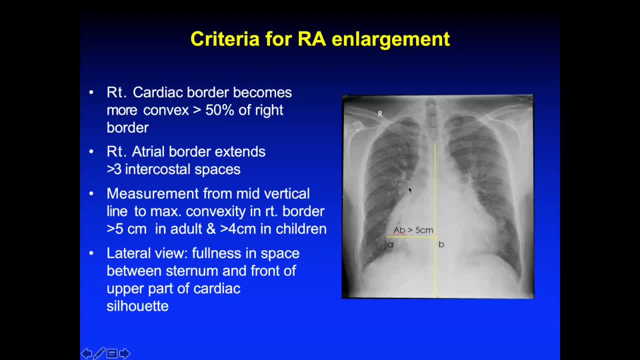 So beyond three intercostal spaces, Any right cardiac border if it extends. this is basically enlargement of right end layer enlargement. So first criteria and the easiest way out is right atrial border extending more than three intercostal spaces. Second is measurement from the mid vertical line to the maximum convexity in right, more than five centimeter adult and more than four. 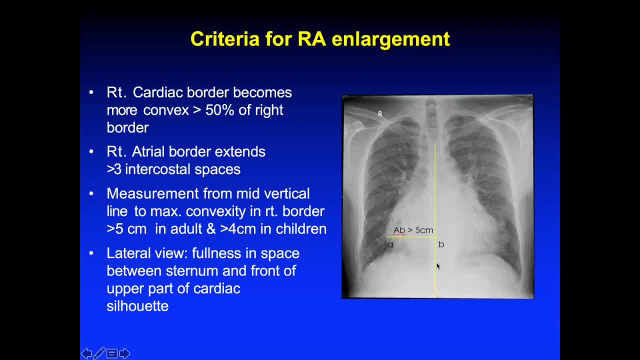 So second criteria is you again draw a vertical line from the spinous process and then a transverse line to the maximum convexity of right atrium, And if the distance is more than five centimeters In adults, of more than four centimeters in children, 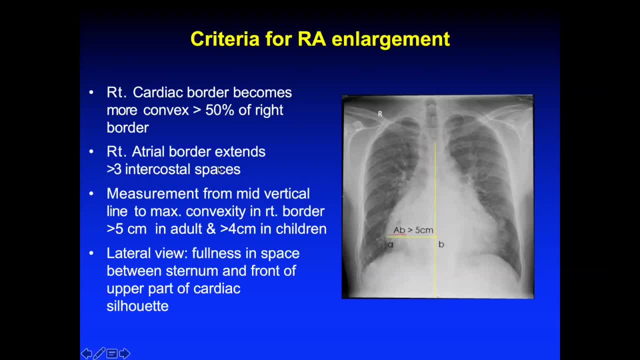 So this is again a second criteria. Third thing is that right cardiac border become more convex, more than 50% of the right border. So again, this is a very soft criteria. So the two main consistent criteria are: right atrial border more than three intercostal spaces and the distance is more than five centimeters. 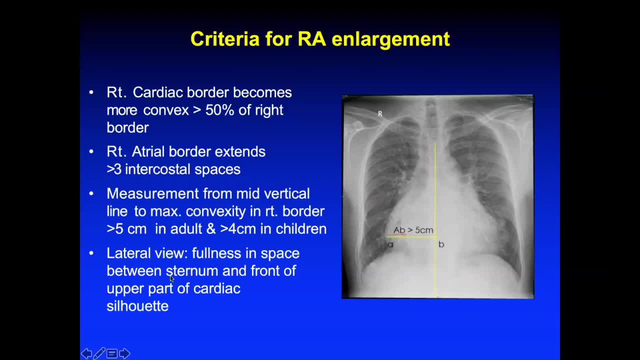 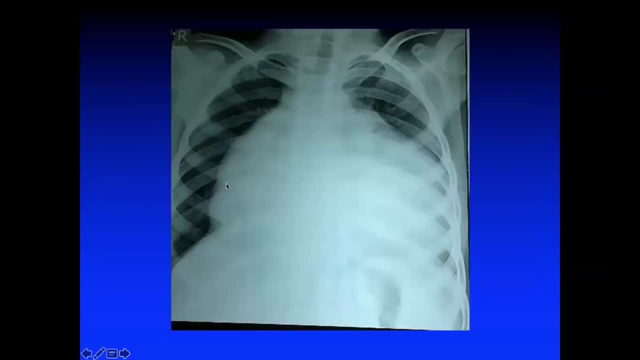 On a lateral view. fullness in the right space between sternum and upper part of the cardiac silhouette is again a criteria for a lateral view. Some might, some examiners might ask you this. So here you can see A case. first of all, once you identify that, okay, there is cardiomegaly, the CTR ratio in any case is obviously more than 0.55. 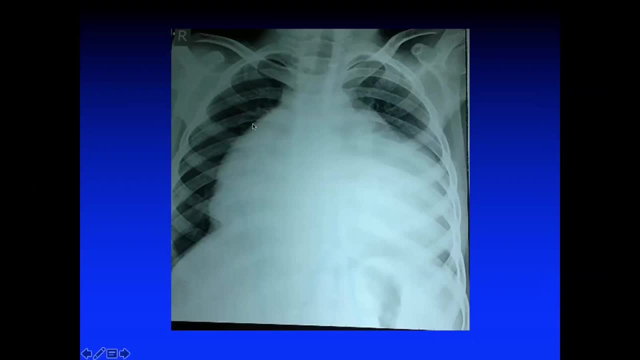 Here you can see, there is this right cardiac border. So the right cardiac border, if you can see it, extends from more than one, two, three, four, five intercostal spaces, So it's massively enlarged. Again you can draw a vertical line. 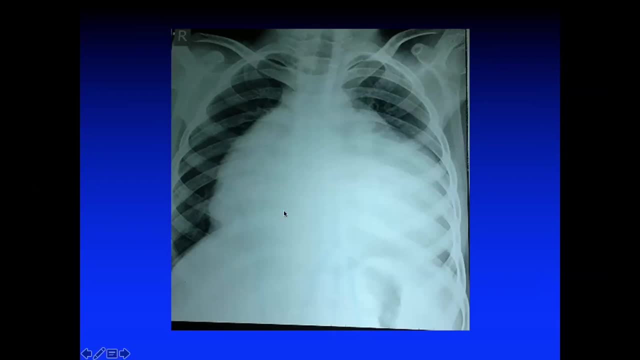 And obviously it appears more than five centimeters, more than 10 centimeters. This is why you can make a diagnosis. So this is the case of Epstein's, And you know this right atrial border was massively enlarged. 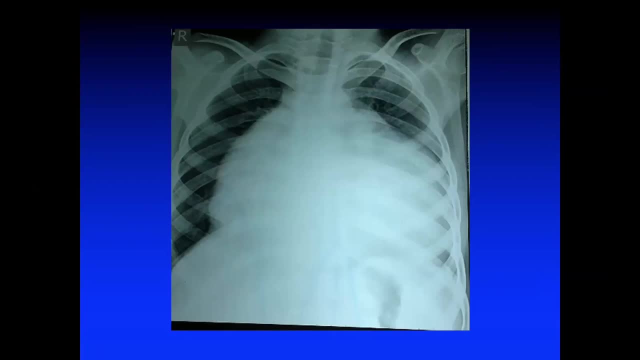 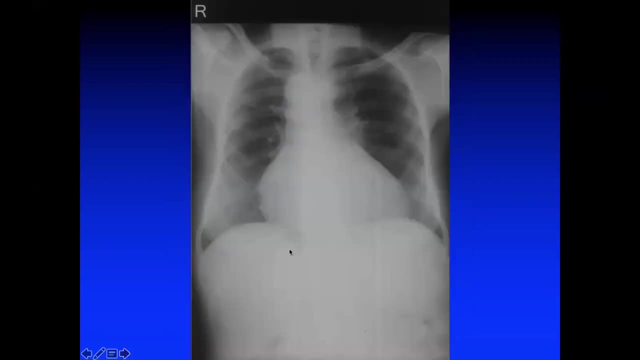 This is what you are given in exams And you are given sometimes a spotter, sometimes you know. so you are asked to identify the criteria And then you should be very clear about the criteria for right atrial enlargement. This is another X-ray. 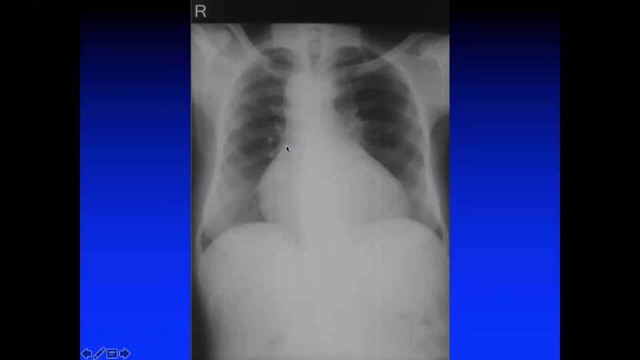 So one, two, three, you know, up to four. So this is the right atrial border, Or again you can draw from here. It obviously appears more than five centimeters, So this criteria should always be fulfilled. 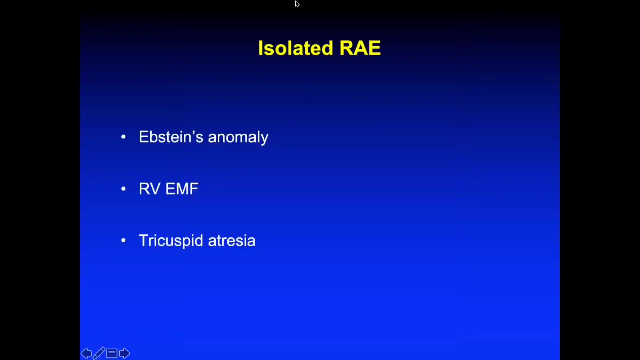 This is the right atrial enlargement. So if someone asks you that, what are the causes of right atrial enlargement Isolated? Obviously there are other causes of right atrial enlargement, be it atrial cervical defect, pulmonary hypertension. So isolated, like a person, only has a right atrial enlargement. 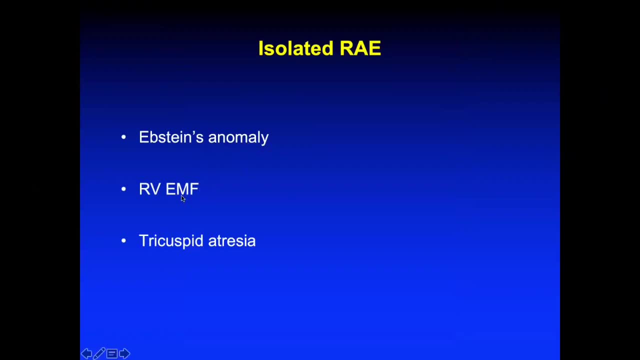 There are three causes: Epstein's anomaly, right ventricular endomyocardial fibroelastosis and tricuspid atresia. These are three important causes of isolated right atrial enlargement. Then second and the most important criteria: criteria for left atrial enlargement. 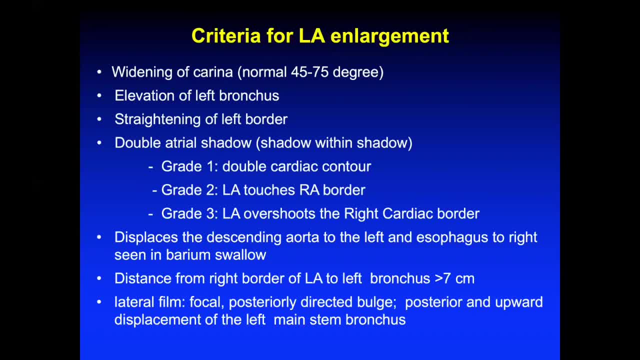 And this is what is being commonly exercised in exams, be it postgraduate or even post-graduate exams. So what are the criteria for a left atrial enlargement? First and foremost criteria is widening of the carina. The carinal angle normally is 45 to 75 degrees. 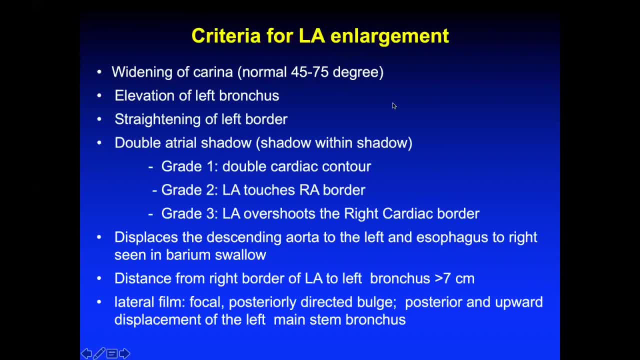 So if it appears more than that, then this is the first criteria being fulfilled and widening of carinal angle. Second will be the elevation of the left bronchus. So the left main bronchus is being elevated, There is straightening of the left heart border. 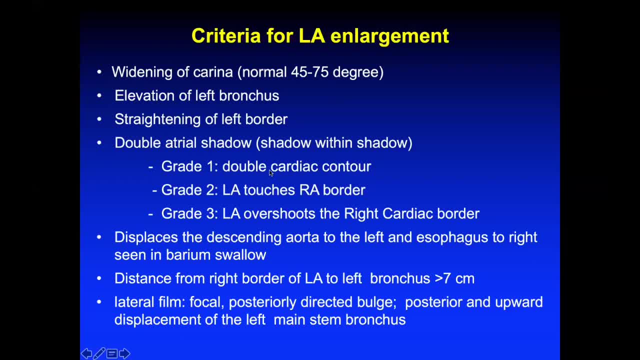 Then there is a double atrial shadow, That is the shadow within the shadow. There is also a classification system. Sometimes someone asks you that what is the severity of the atrial enlargement? So there is grade 1,, grade 2, and grade 3.. 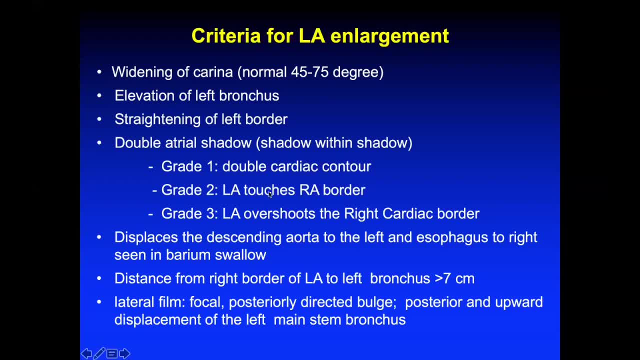 Grade 1 would be double atrial, double cardiac contour. Grade 2 is when the left atrial border touches the right atrial border And grade 3 is when the left atrial overshoot the right cardiac border. Then another criteria for left atrial enlargement is displacing the descending aorta to the left and esophagus to the right is seen in William Swallow. 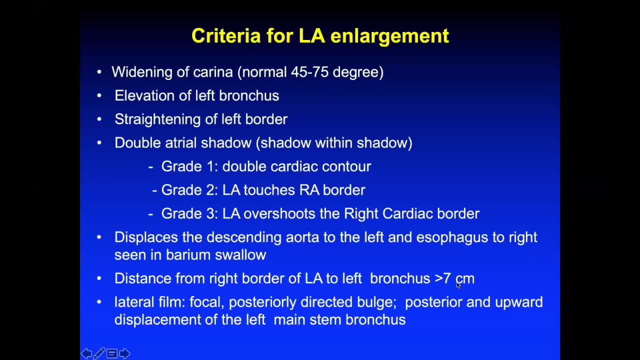 Distance from the right border of LA to the left bronchus being more than 7 centimeters on a lateral fill. It is focal, posterior directed bulge, posterior upward displacement of the left main bronchus. So we will see one by one, what are the criteria. 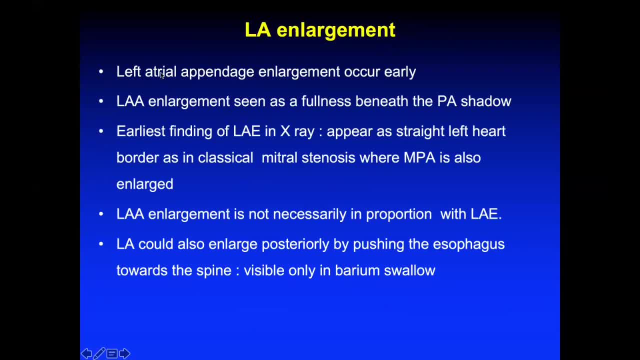 Now in an LA enlargement, normally first would be the left atrial appendage which enlarges. LA enlargement appears as a fullness beneath the PA shadow. The earliest finding of left atrial enlargement is a straight left heart border ascending practical mitral stenosis where MPA is also enlarged. 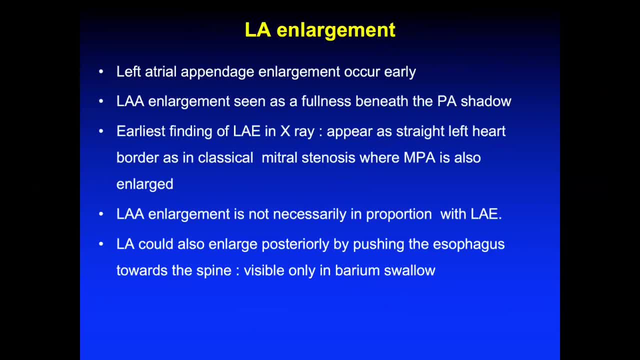 So first thing would be a left atrial appendage which gets enlarged, will become more prominent And the thing is, the thing you see on an x-ray would be a straight heart border. So a straightening of the cardiac border is the first sign of a left atrial enlargement in form of left atrial appendage which enlarges. 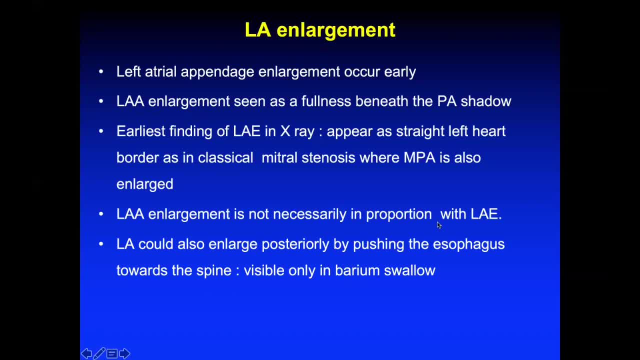 Now, LA enlargement is not necessarily proportioned with left atrial enlargement, So it can be, depending on what stage the presentation is there. So mostly the left atrium enlarges posteriorly, superiorly, in upward direction. So if it enlarges in upward direction, superiorly and posteriorly, 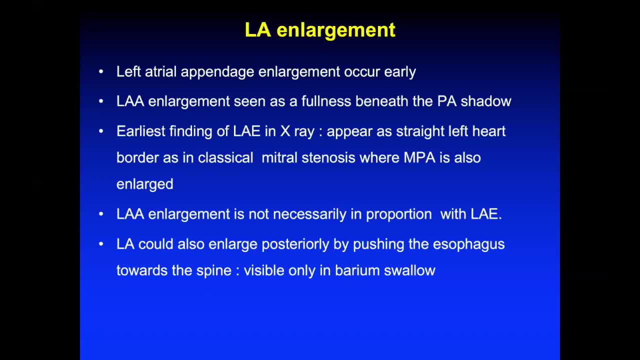 So the only space it can have is upper, So it can push the main bronchus above, So you will have a displacement of the left main bronchus. Whenever the left main bronchus is displaced, you will have the enlargement of the carinal angle. 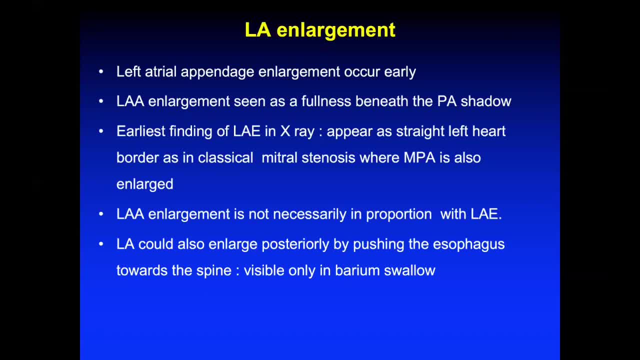 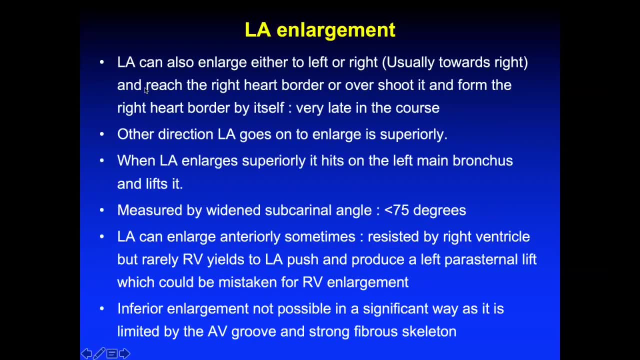 So the left main stem bronchi appears widened and then you will have the double cardiac contour. So LA can also enlarge either on the left and the right and reach the right heart border. So first it will enlarge superiorly upwards into the left. 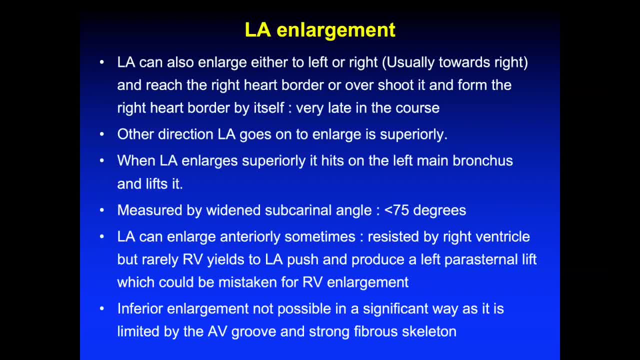 So this will lead to an widening of the carinal angle and you know this, elevation of the left main bronchus. So first earliest sign of left atrial enlargement is straightening of the left heart border. The second sign would be elevation of the left main bronchus and widening of carinal angle. 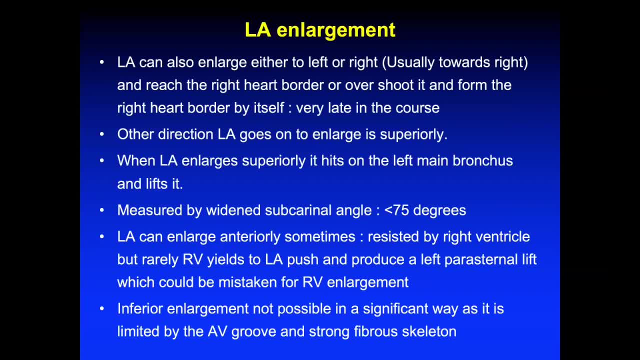 The third sign would be: now LA doesn't have a space to enlarge on the upper side. So now it will start enlarging towards the lower side. So it will come towards the right side and it will reach the right heart border. It can overshoot it. 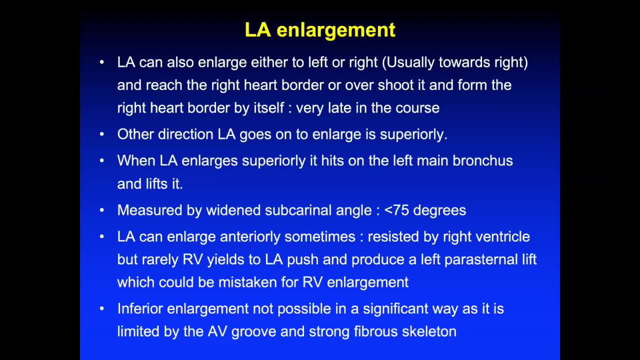 So it will form a double atrial contour or a double cardiac shadow. So double cardiac shadow is the third in the course: Straightening of the left heart border, earliest appearance. Then it will be the straightening or elevation of the left main bronchus and widening of carina. 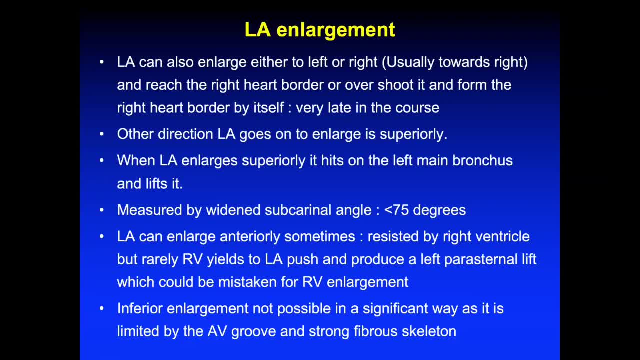 And the third would be, you know, it reaches the right heart border and it forms a double atrial shadow. Now, the subcarinal angle is normally less than 75 degrees. If it becomes more than you know, 75 or sometimes 90 degrees, it becomes very prominent. 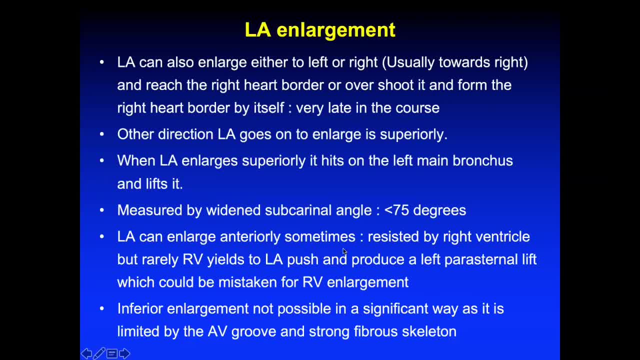 And LA can sometimes enlarge anteriorly. But anteriorly you will have right ventricle age resist. So sometimes You can have an LA enlargement- rarely But you know, whenever LA is seen in mitral regurgitation. the largest left atrial diameters are seen in cases of mitral regurgitation where you have aneurysmal LA. 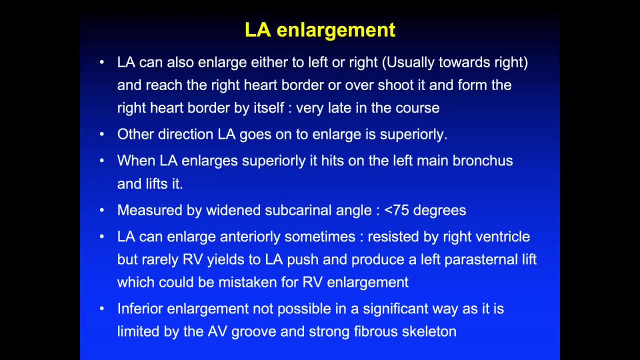 So in that case it can enlarge anteriorly, It can lift the right ventricle and it can also produce a left parasternal lift which is, on a clinical examination, quite prominent. Inferior enlargement is not possible in a significant way. 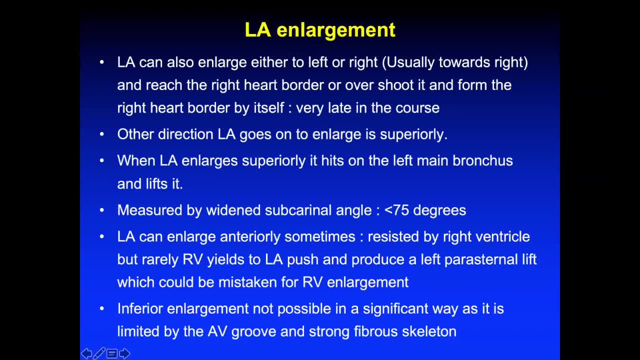 It is limited by the AV groove and the strong fibrous cartilage. It can never enlarge inferiorly. So it can only enlarge superiorly, upwards and left, Or it can enlarge towards the right side, Or rarely as an anterior. No posterior enlargement, no inferior enlargement. 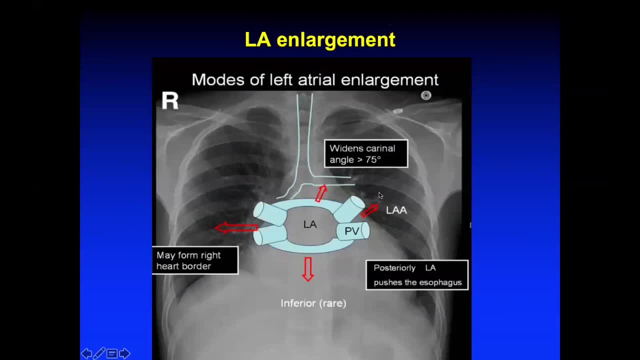 So here the modes of the left atrial enlargement. if it enlarges upwards and to the left and superiorly, it will elevate the left main bronchus, It will widen the carinal angle and it will make it more than 75 degrees. 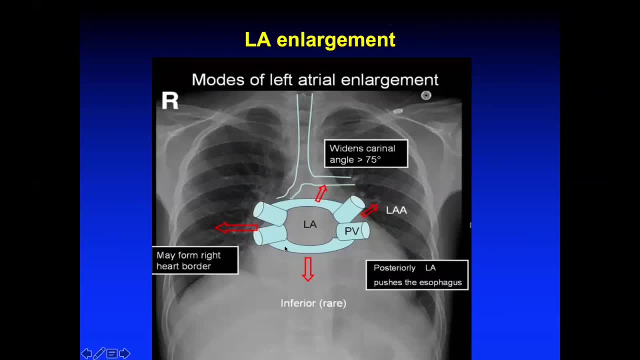 If it basically enlarges towards the right side, it will form the right heart border. Inferiorly it doesn't. If it goes posteriorly, it will push the esophagus, Because behind the LA lies the descending aorta and the esophagus. 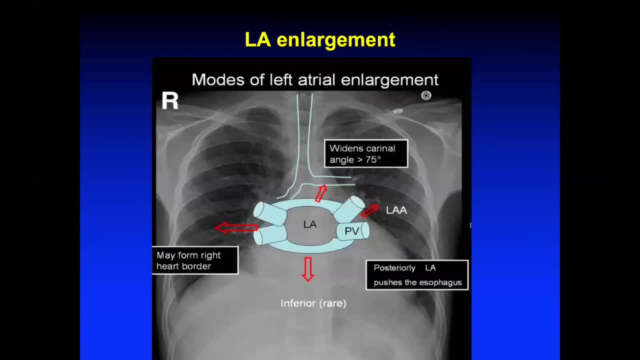 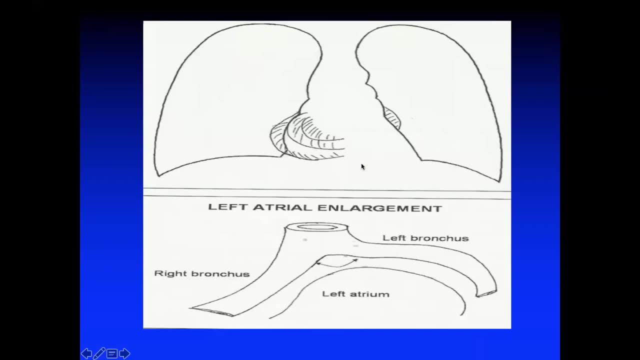 So it will push the esophagus and it will cause compression of the esophagus and patient may report with dysphagia. So here, elevation of the left bronchus, widening of the carinal angle and displacement of this. 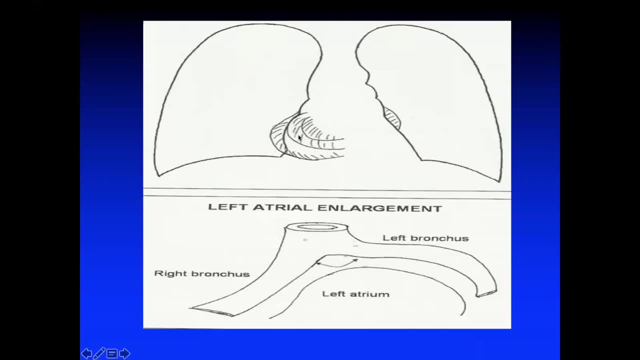 So first thing is the straightening of the left heart border, Then the displacement of the, that is, the double atrial shadow. This is what you. double atrial shadow, This is a grade 1. double atrial shadow- This is grade 2.. 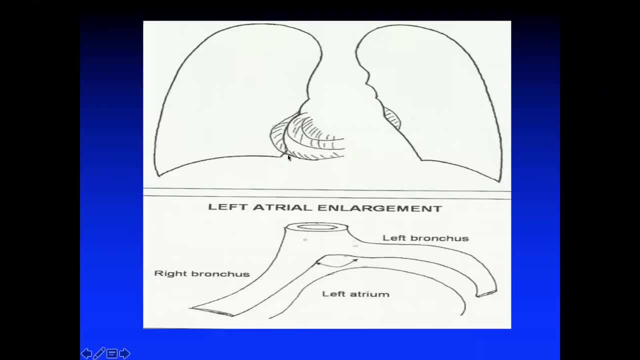 This is the right atrial border And the grade 3 is the left atrial border. It overshoots it. So grade 1, grade 2 and grade 3.. So this is a double cardiac contour, or double atrial shadow. you can see. 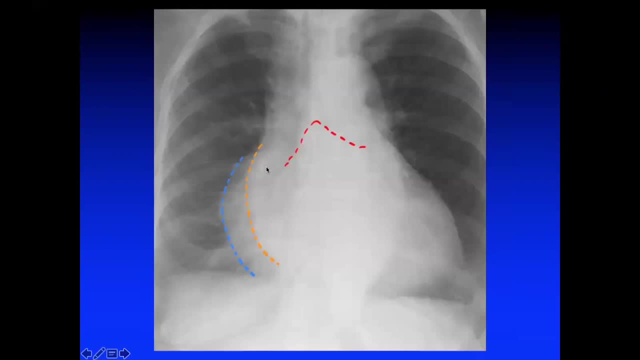 And these are the elevation left main bronchus. So here you can clearly see the two cardiac contours. One cardiac contour is continuous with this. So this is the right cardiac contour, That is the right atrium, And this is another contour beyond it. 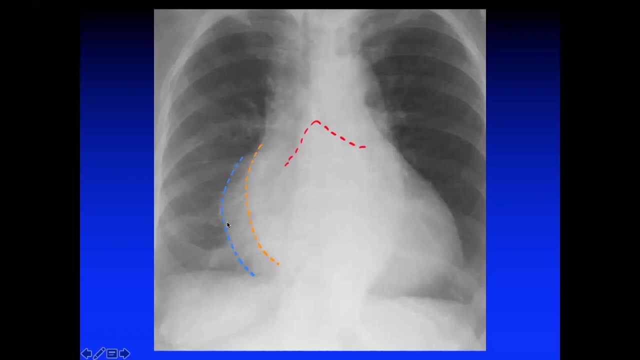 So the left atrium has enlarged and has come here. So this is basically, And there is elevation of the left main bronchus, There is widening of the carina. So this is what you have: a left atrial size. 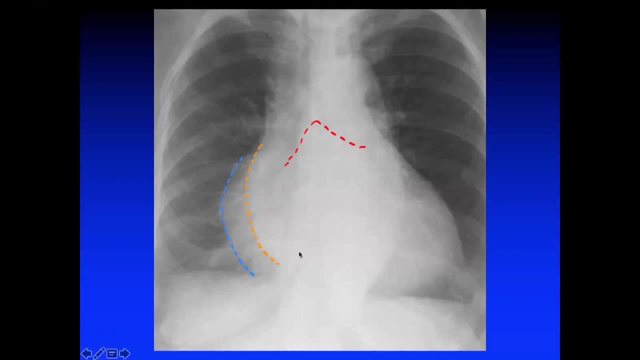 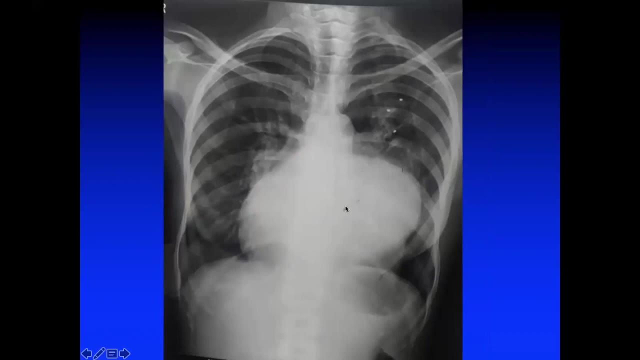 And this is the right atrium. So this is the grade 3 left atrial enlargement. on an X-ray Again, and a very important X-ray, you can see here The left atrium has enlarged towards the left side. It has enlarged towards the right side. 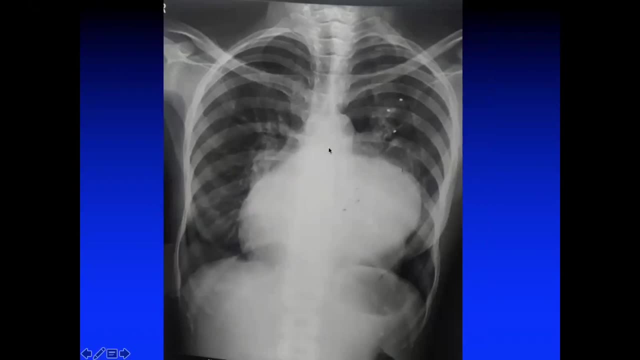 You can see a double atrial shadow. You can see the widening of the carina. You can see a wide spaced carinal angle. You can have a left main bronchus which is elevated. So this is again a case. So I need to use my left atrium in the case of severe mitral disagitation. 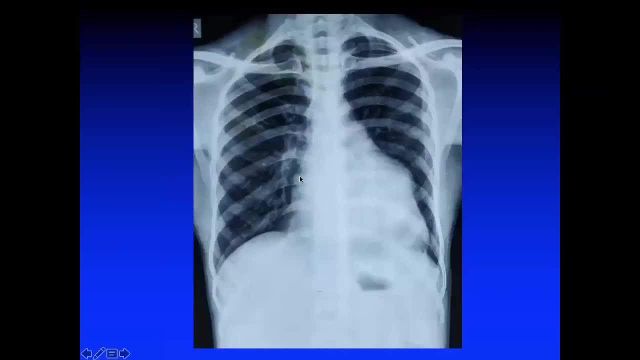 This is again you know, focal atrial enlargement. Here you can see one cardiac contour. This is the second cardiac contour. This is the enlargement of the left atrial appendage, Now straightening beyond the straightening. So this is the earliest signs you can see on an X-ray for left atrial enlargement. 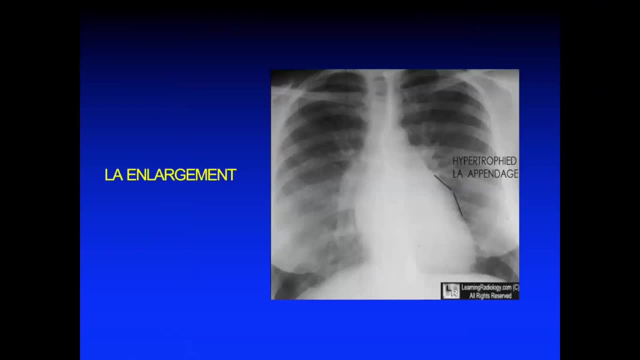 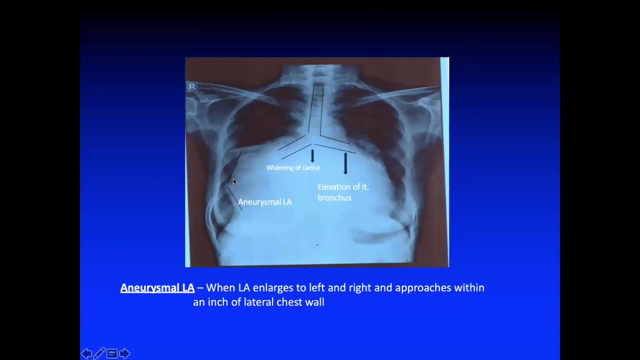 So hypertrophic left atrial appendage again appears as this way: And it is my LA When the LA enlarges to the left And right. So here you can see it has continuously completely reached up to the right cardiac margins. 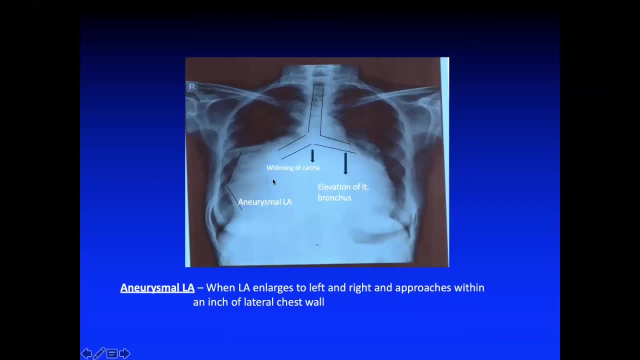 This is what you can see in enlargement. So everything you can see here is left atrium. So case of severe mitral disagitation, There was widening of the carina, There is elevation of left main bronchus And there is aneurysmal LA. 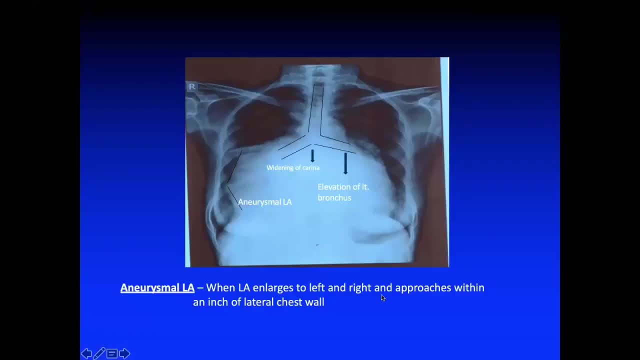 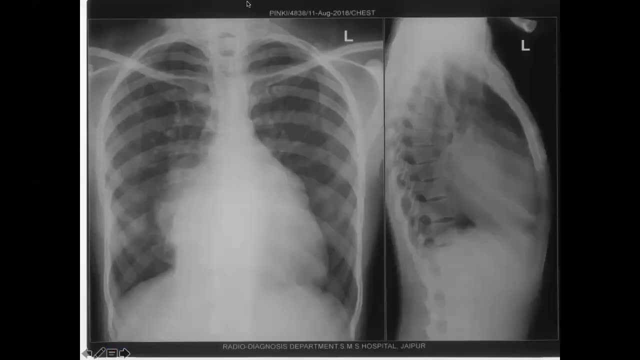 So on a radiologically, when LA enlarges to the left and right and approaches within an inch of the lateral chest wall. So that is basically a criteria for aneurysmal LA on a chest X-ray. So sometimes may I ask you this: 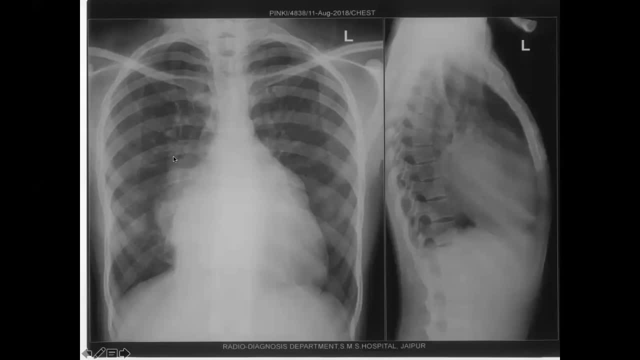 This is another X-ray. what you can see Here. you can have one cardiac border Here, another cardiac border. So this cardiac border, This is continuous with the right side, This cardiac border is appearing beyond this. So this is basically grade 3.. 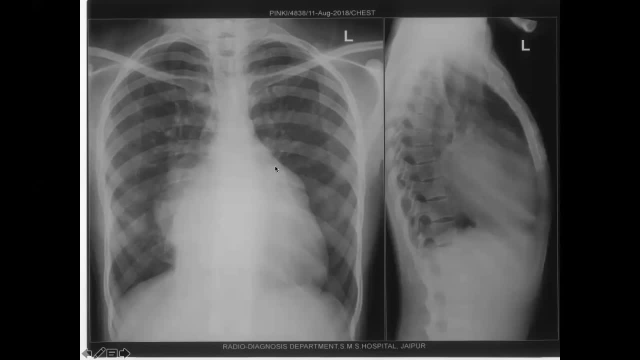 Case of left atrial enlargement. Then again, the left atrial appendage also appears enlarged posteriorly here. So this was basically a young female where she had come to us with dysphagia And somewhat hoarseness of voice And this was the X-ray. 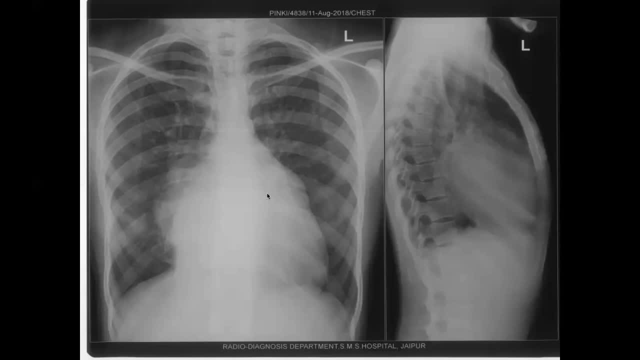 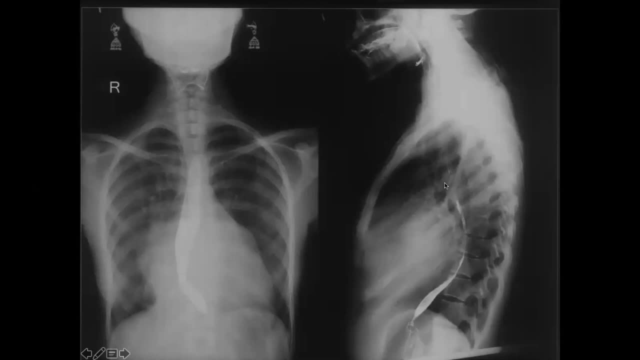 So on the basis of X-ray We made a diagnosis that there was massive left atrial enlargement. Here you can trace the cardiac contours on the left atrium. So then we did a barium swallow And what you can see classically on a barium swallow? 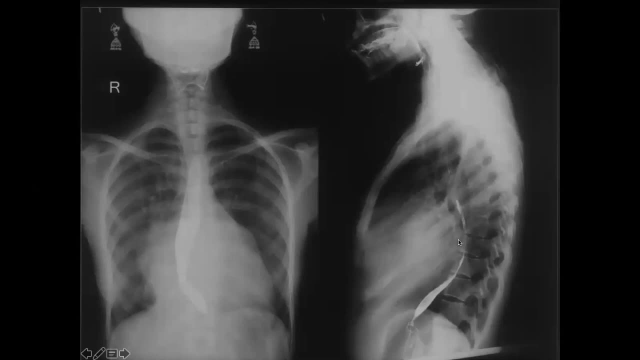 The esophagus is displaced to the right side, But here you can see This is marked narrowing of the stenosis of the esophagus Because of the left atrium which is pushing the esophagus. So this is basically a classical case of patient presenting with dysphagia and autism syndrome. 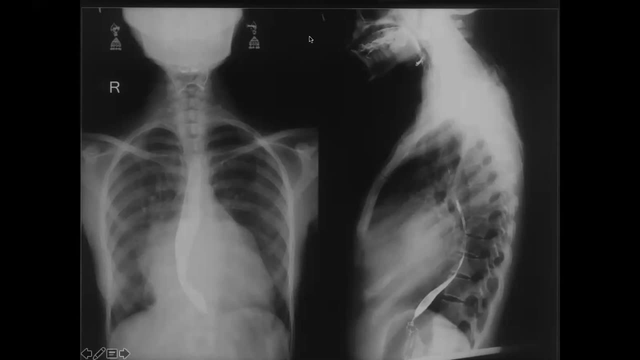 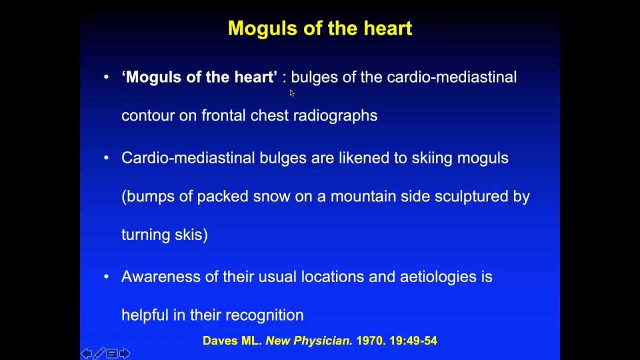 And this is aneurysmal LA. She was diagnosed with a case of rheumatic heart disease With mitral regurgitation, With aneurysmal with large size LA. So another question is being asked: in your exams Could be the moguls of the heart. 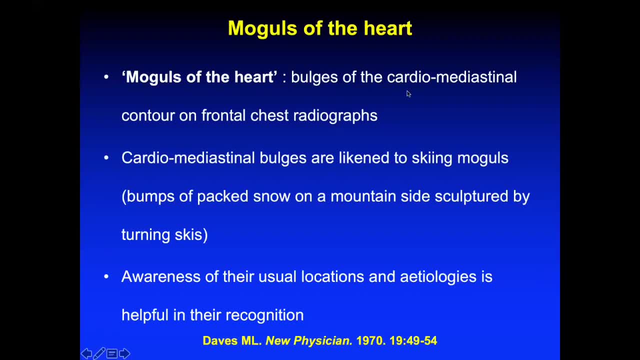 So what are the moguls of the heart? These are basically the bulges of the cardiomediastral contour on frontal chest X-ray On a PA view. Some bulges are seen on the X-ray On the cardiomediastral contour. 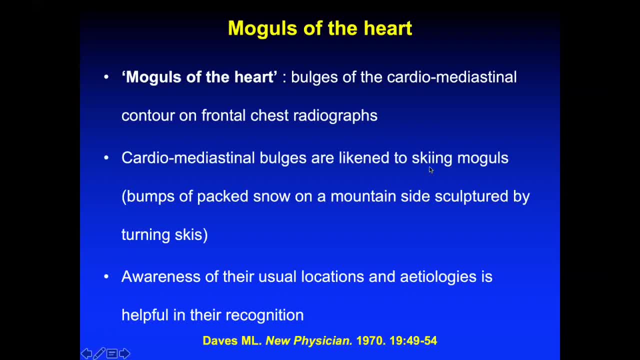 And they are basically called moguls. So the cardiomediastral bulges are likened to a skiing moguls, That is, bumps of packed snow on a mountainside Sculptured by turning skis. Someone asked you that. what is a mogul? 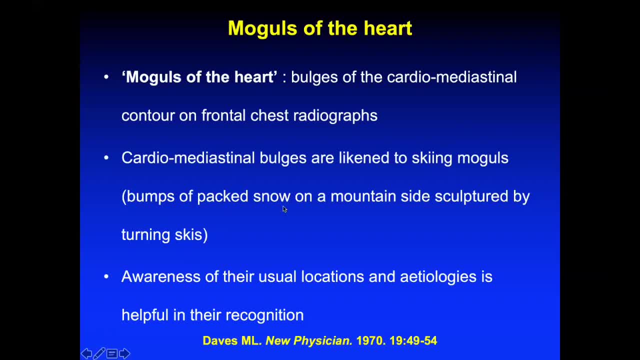 So basically it refers to a skiing mogul. This is basically a packed snow on a mountainside. Someone has gone for skiing, So you can be very clear to them. Awareness of the location and etiology is very important, So you will have various moguls. 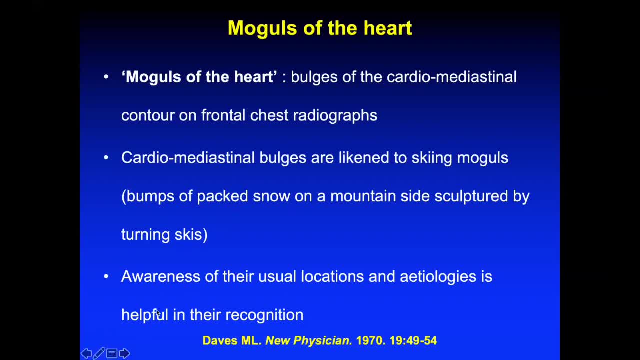 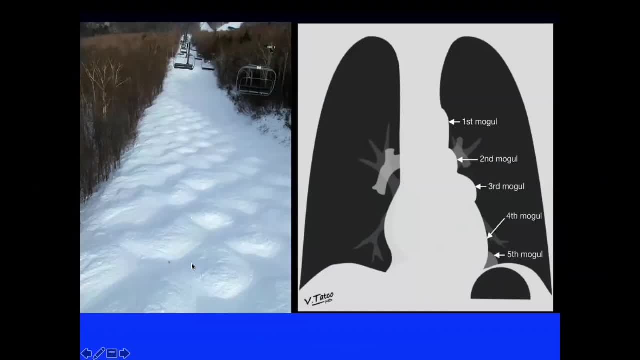 First, second, third, fourth, fifth. So one should know what are the causes and what is the abnormality. So these are basically the moguls, They are bumps of snow, Basically with the skiing tracks, And these, basically, are seen on an X-ray. 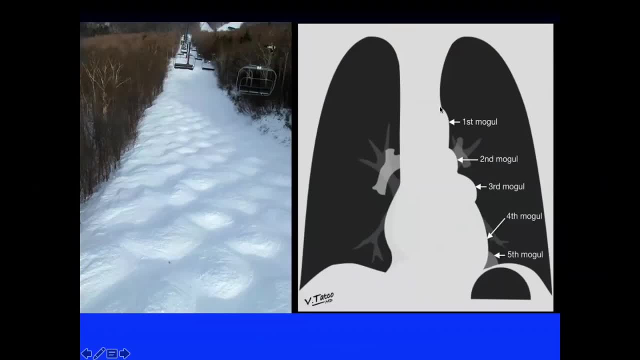 So when they are seen on X-ray We call them moguls. So there are five moguls. There is first mogul, There is second mogul, There is third mogul, There is fourth mogul, There is fifth mogul. So all the moguls are located on the left cardiomediastral contour. 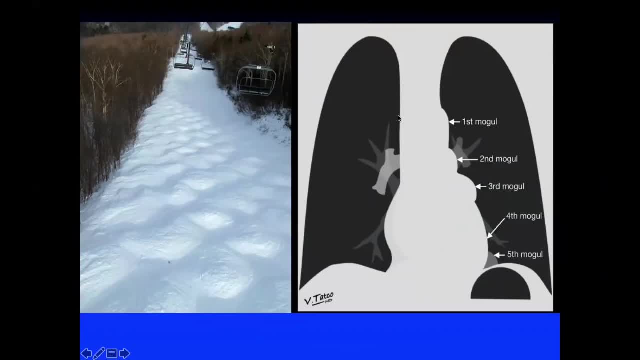 So this is always clear, that one should not try to find out the moguls of the heart on the right side. So in exam we will be asked that: okay, describe the first mogul, the second, third, fourth and fifth. So first mogul. 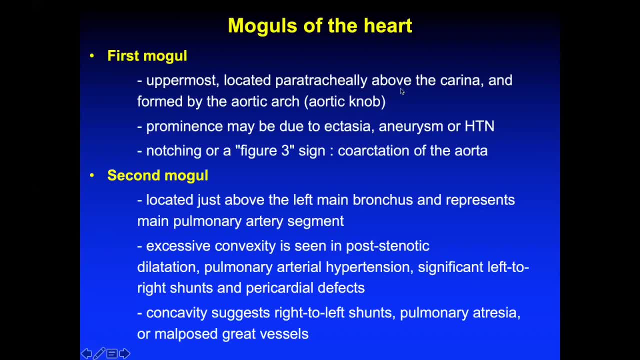 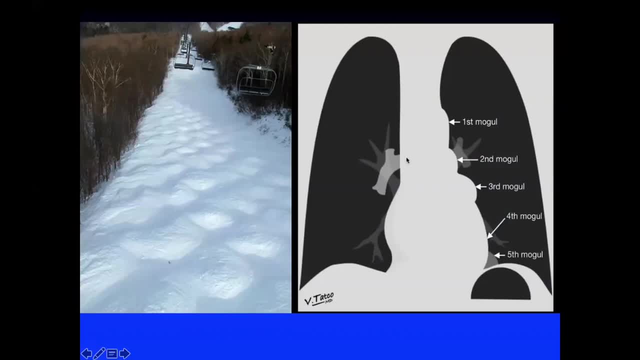 It is the uppermost, located peritracheally above the carina and formed by the aortic arch. So this is the first mogul And this is basically formed by the aortic arch. So normal structure which is present in the first mogul is the aortic arch. 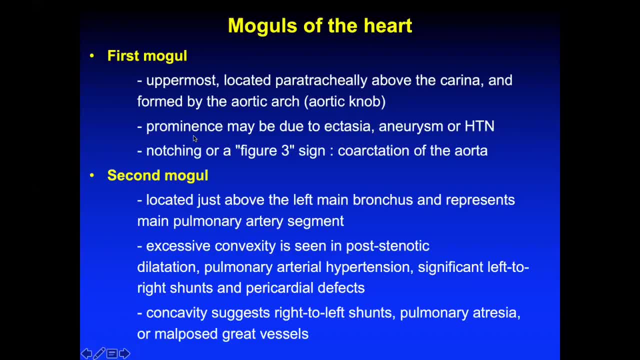 Now aortic arch may get prominent. So in a diseased state your first mogul will appear as because of actasia. So there can be an aortic actasia or aortic aneurysm, Or it can be even in hypertension. 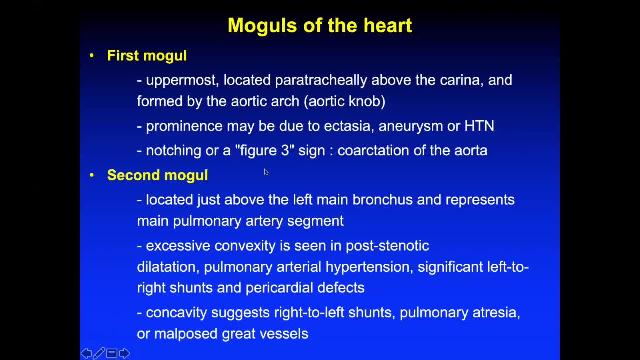 There is also a figure called figure of three, sign or notching of the aorta. We have seen co-operation of aorta, which will come on later on in our presentation. So in co-operation of aorta you will have a notching. 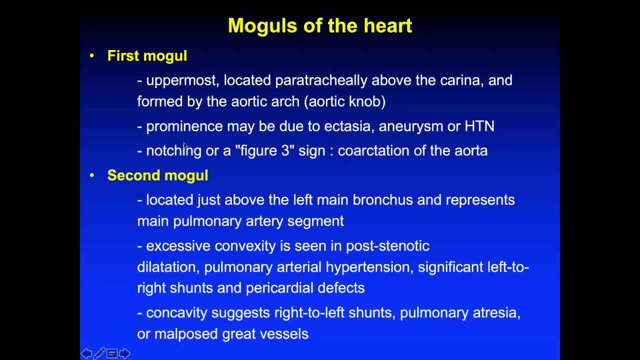 Which is seen in the first mogul. So there are two abnormalities in first mogul. First is aneurysm and hypertension And second is the figure of three sign or notching. There is a second mogul. It is located just above the left main bronchus and represents the main permeatory segment. 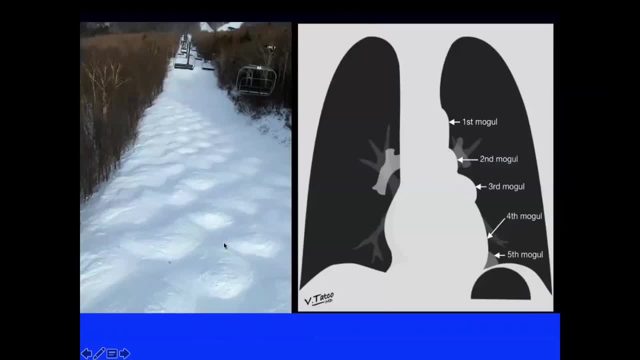 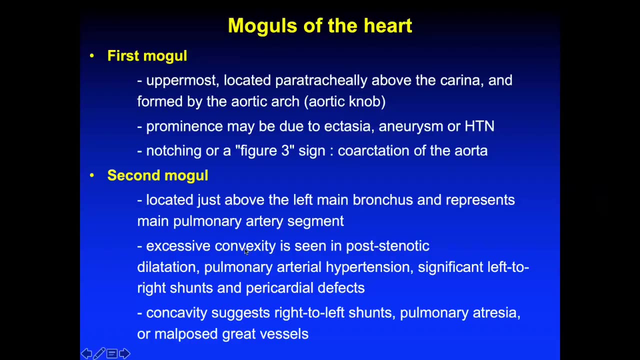 So here this is the second mogul Where you will have main permeatory segment just above the bifurcation of the trachea And it is excessive convexity is seen in post-tenotic perme dilatation. So if you have a case of permeous stenosis, 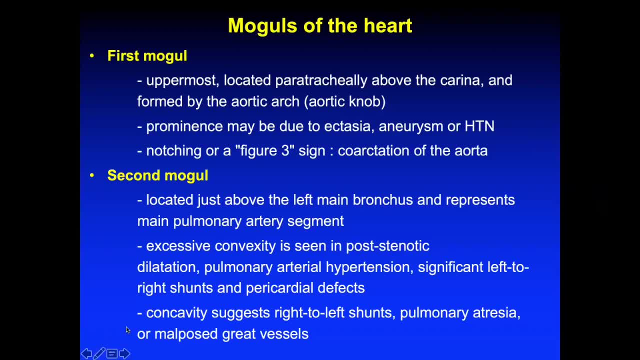 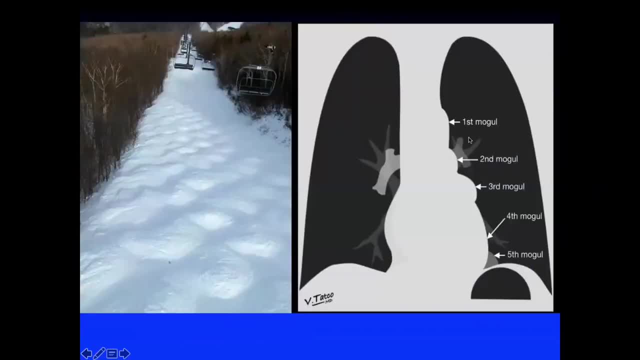 It can be mildly enlarged pulmonary artery, Pulmonary arterial hypertension Or significant left to right shunts and pericardial disease. So if you have a very prominent second mogul, So if it appears very convex, So these are the causes of it. 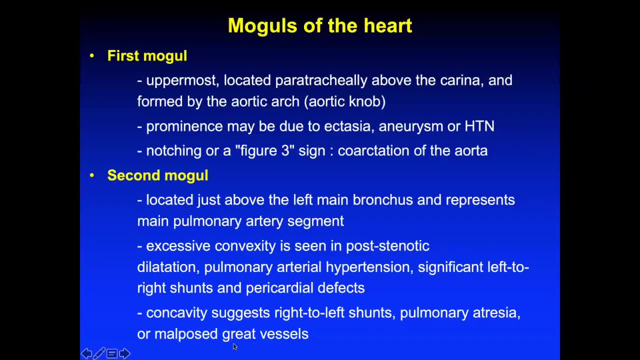 Concavity suggests that right to left shunt pulmonary atresia or malport. So if you have a mildly enlarged pulmonary artery So there will be a mild convexity in the second mogul And these are the causes of that. 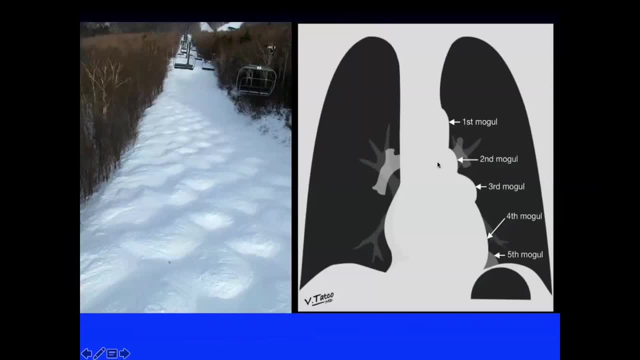 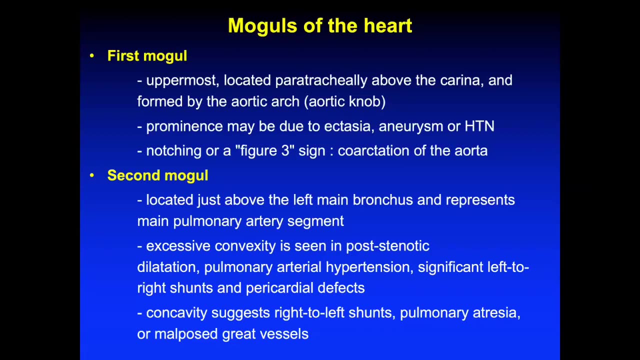 If there is concavity, that instead of appearing convex it appears as concave, This means the pulmonary artery is absent. So either there is a pulmonary atresia Or right to left shunt where the pulmonary blood flow is. you know less. 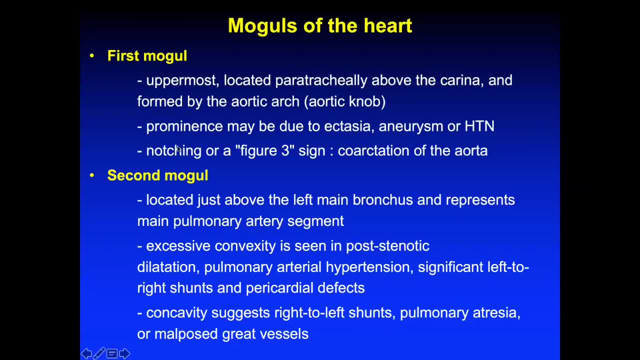 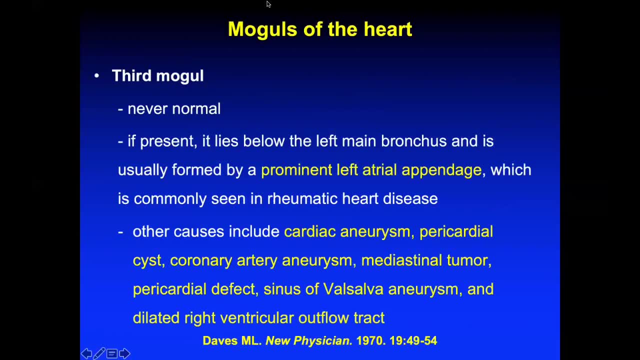 And you will have malport grade vessels. The vessels are not properly positioned, So they are interior and posterior. So this is again second mogul. Third mogul is never normal, So in all cases of heart. So if someone asks you, the third mogul. 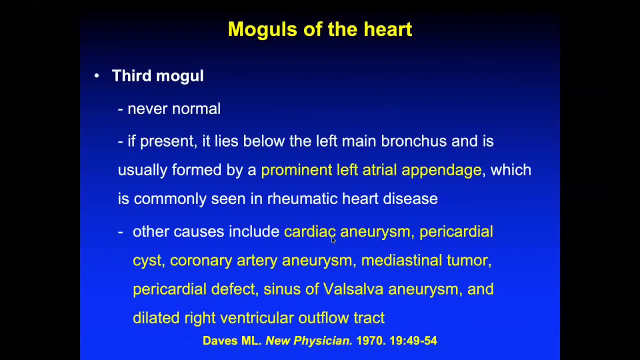 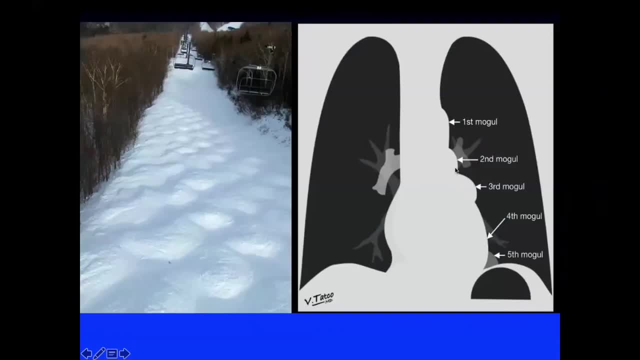 So this is always abnormal And if it is present, It lies below the left main bronchus And usually formed by prominent left rectal leprosy And there is no normal structure located. So if you have a third bump on an x-ray, 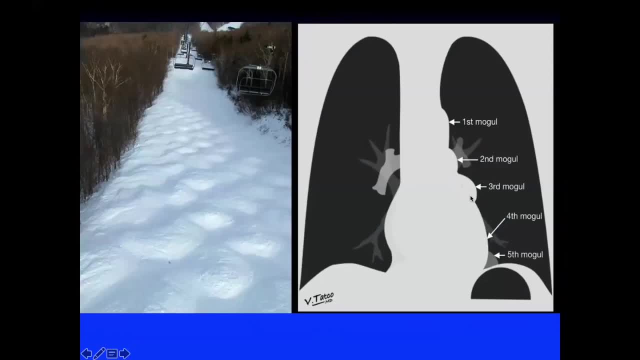 There is always, most common causes, enlarged left atrial appendage. So in an exam you generally be given an x-ray of mitral stenosis And they will ask you that, okay, this is what this appears. So this is basically the third mogul. 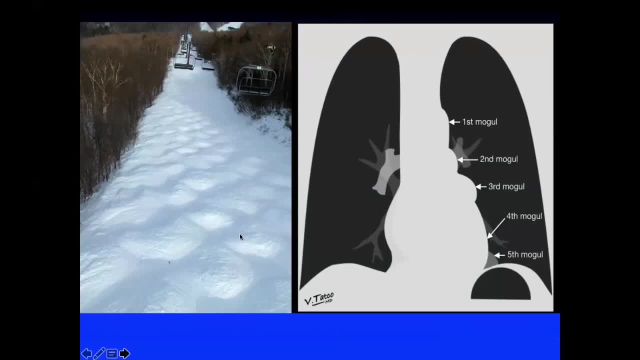 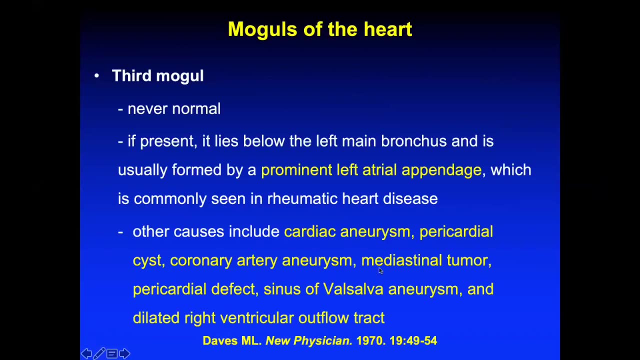 And that is basically. it is the enlarged left atrial appendage Which is commonly seen in rheumatic heart disease. Other causes include cardiac aneurysm. There is pericardial cyst. Coronary artery aneurysms can be there. 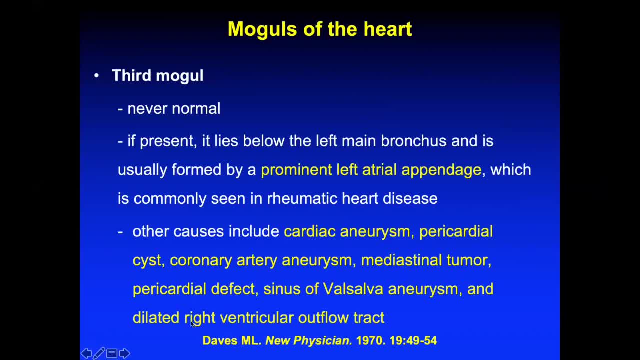 There is pericardial defect, Sinus of valsalva, aneurysm And dilated right ventricular outflow tract. So these are again the causes. So in exam they will always ask you: what are the causes of a third mogul? 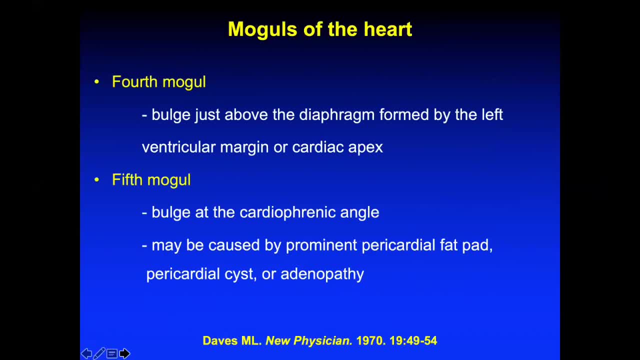 Which is very prominent. And these are the differentials. Then the fourth mogul is the bulge over the diaphragm And it is formed by the cardiac apex. That is very simple. Fifth mogul is again, the bulge of the cardiophrenic angle. 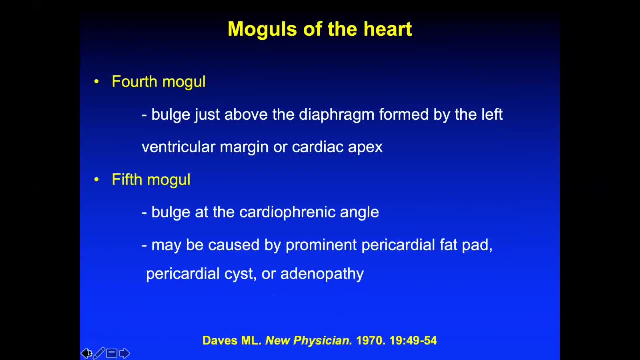 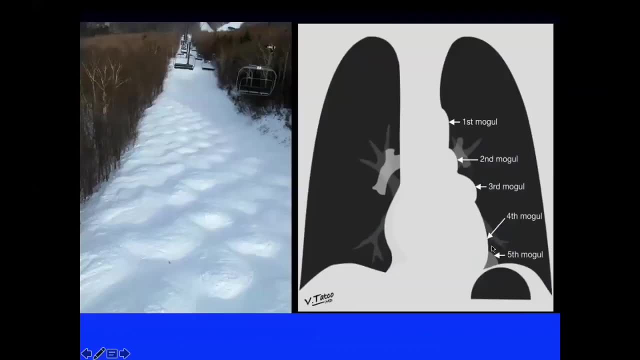 And the causing very prominent pericardial fat, Pericardial cyst or adenopathic Some lymph nodes, Pericardial cyst. The fourth mogul is formed by the left ventricular apex. It is always normal. Fifth mogul can be formed by the pericardial fat. 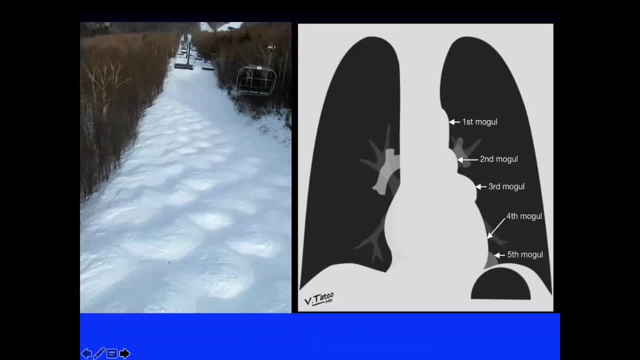 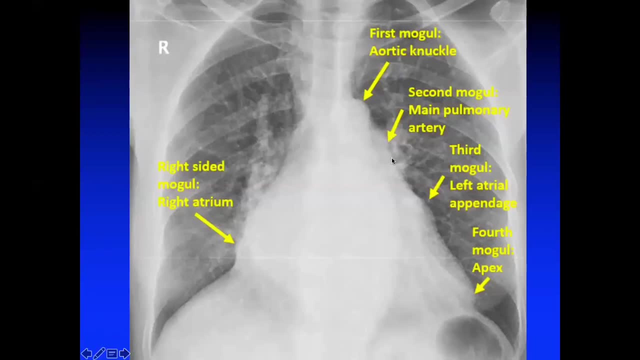 Pericardial, you know, Or there can be some tumour Or sometimes even lymph nodes. So here, just on an x-ray, you can see the first mogul, That is the aortic knuckle. Second mogul is the pulmonary artery segment. 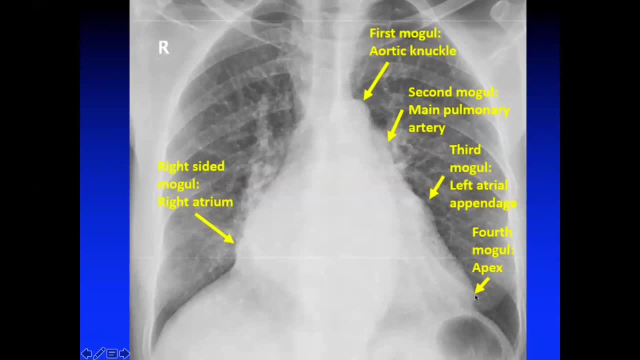 Then you will have a third mogul, Left ventricular appendage. Then you have fourth mogul, The apex, And here sometimes you can have the fourth mogul. Sometimes even examiners will ask you: what is the right sided mogul? So right atrium is the right sided mogul. 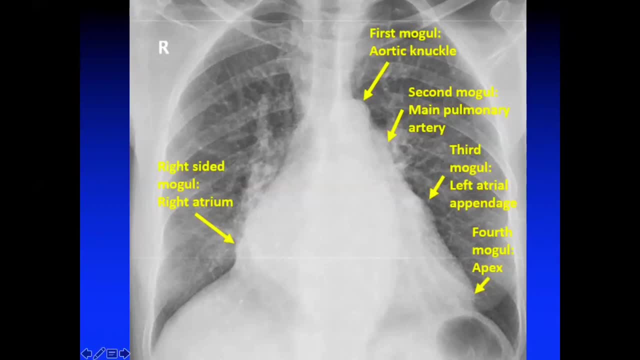 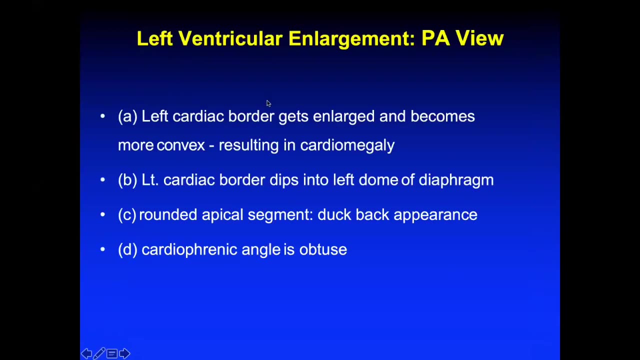 That is because if you enlarge right atrium, It will always form a convexity. So after doing left atrial enlargement criteria and right atrial enlargement criteria, Let's go on to the criteria for left ventricular enlargement. So left ventricular enlargement. 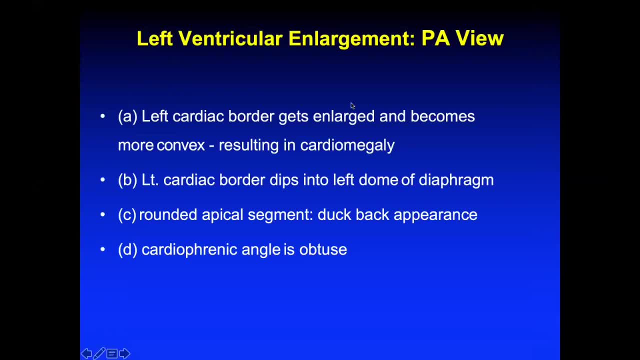 The criteria is very easy: Left cardiac border gets enlarged And normally the left atrial enlargement is always, as we have been treated, in the form of MBBS times. It is always down and out, So down and below Left cardiac border gets enlarged and becomes more convex. 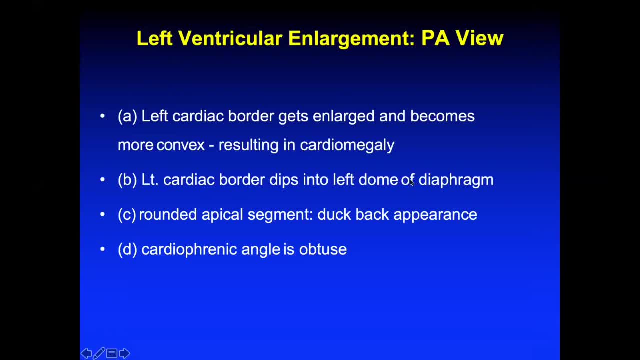 It results in cardiomegaly. Left cardiac border dips into the left dormant diaphragm. So it goes below. It appears as a rounded segment, Duck back segment, Duck back appearance. But the most important and most confusing thing is the cardiophrenic angle. 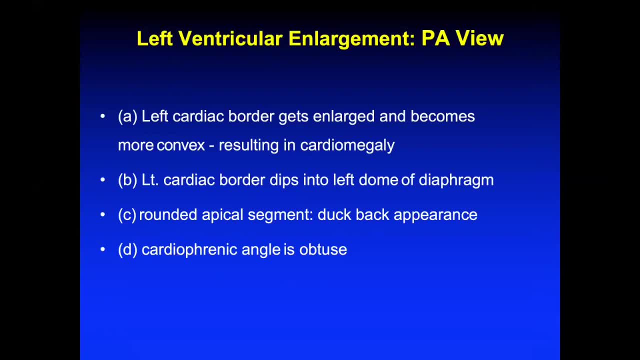 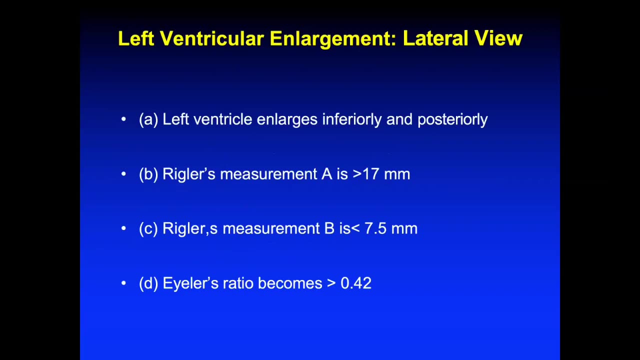 The cardiophrenic angle is always obtuse in the case of left ventricular enlargement. So the lateral view. It always enlarges inferiorly and posteriorly. There are some measurements. Again, these are all exam based. You just need to remember if someone asks you in the exam. 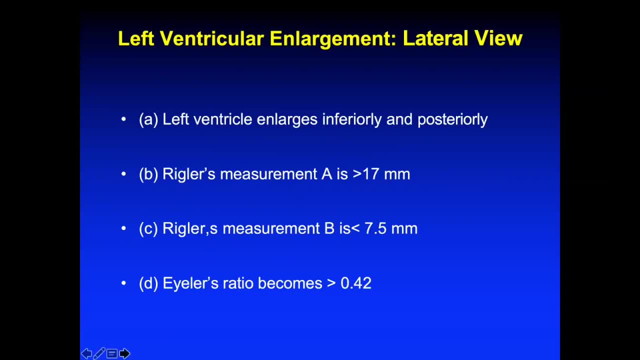 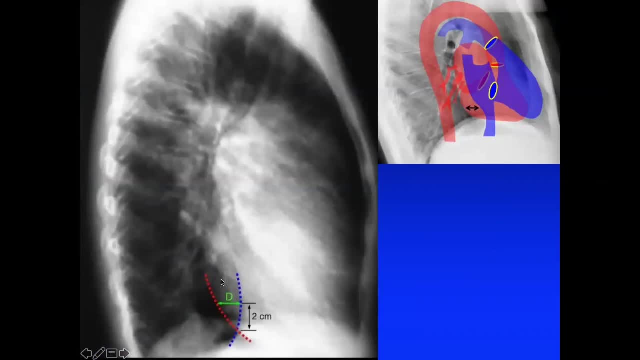 Then what are the criteria? These are not being applied practically as of now. So this is how the left ventricular enlargement is. posteriorly, This is the IVC, And the IVC becomes incorporated into the cardiac margin and goes beyond it. 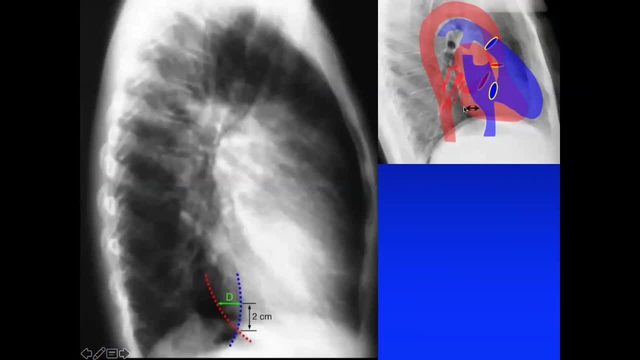 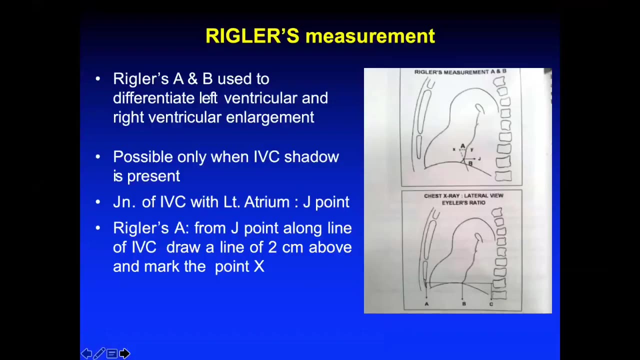 So normally the IVC is lying here. But if the left ventricular enlargement is, if you go posteriorly, So it enlarges posteriorly in a lateral view. Regulars measurement: These all can be skipped up. Eyelers ratio can be skipped because these are not important. 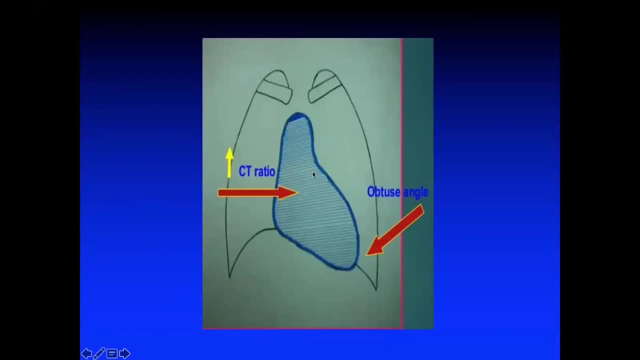 What is more important, at last, to ask you, is that Just focus on this diagram. A left ventricular always enlarges in this way Towards the diaphragm, It becomes more rounded in appearance And the angle that is the cardiophrenic angle. 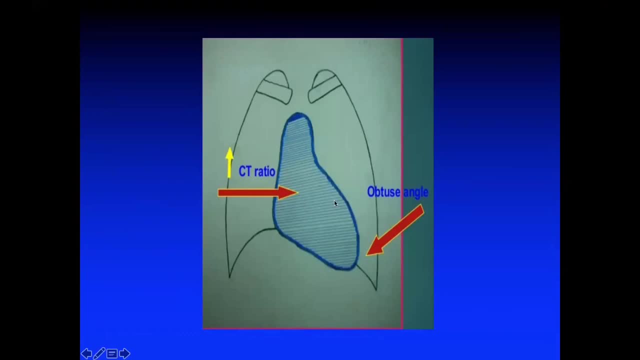 The angle it makes with the diaphragm is always obtuse, So a cardiac thoracic ratio is increased And obtuse angle is made. So these are just two ways you can just differentiate: a left side cardiac apex or a left LV enlargement. 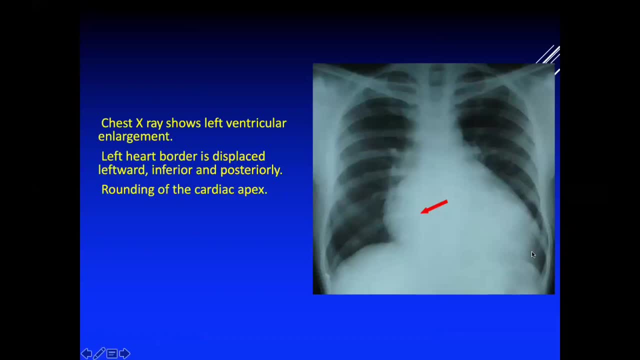 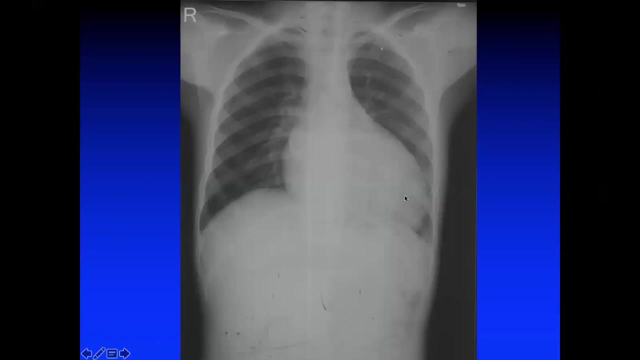 So here you can see This is the LV enlargement And there is a rounding of the cardiac apex. It goes more inferiorly And the angle you can see with the diaphragm is more an obtuse angle. Again you can see the aspect is displaced inferiorly towards the left ventricle. 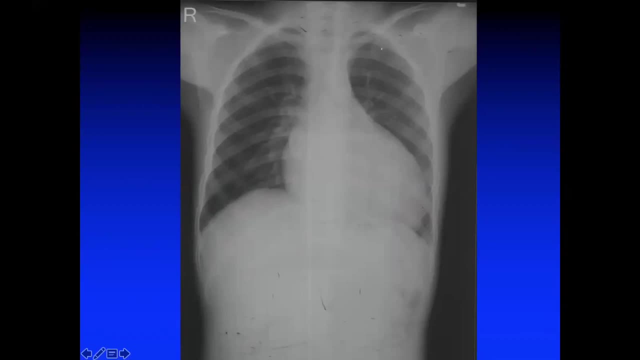 And the angle it makes This angle is more obtuse And also you can note a double lateral shadow And this is grade 2.. This is the right atrium, So grade 2, left ventricular, And then this straightening of the left heart border. 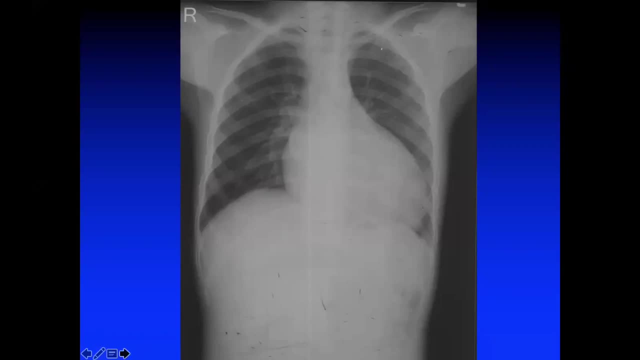 Other points. This is the case of mitral stenosis with MS with MR. So generally you can sometimes get a combined lesion. So if you have an MS with MR, One of the X-rays- Classical X-rays- would be this. 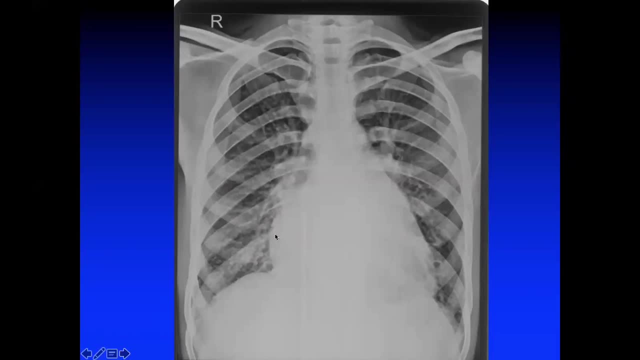 Then this is again a very simple X-ray. You will have double cardiac shadow. This is the two cardiac margins. This is straightening of left heart border. This is the third moment, which is very prominent, And then the left apex, which is the last. 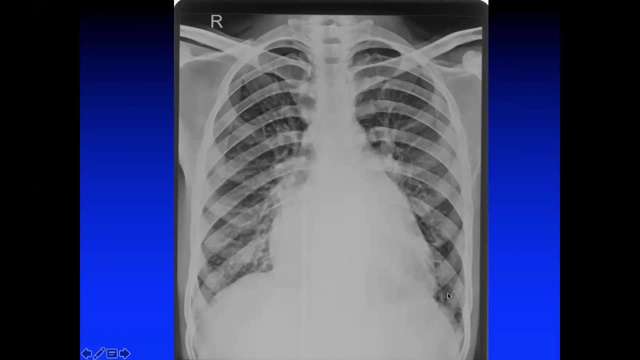 And here you can see the angle. So this angle is obtuse And this is the most important confusing thing. in exams You tend to confuse. You are given a case presentation And then, when you are going to ask to present an X-ray, 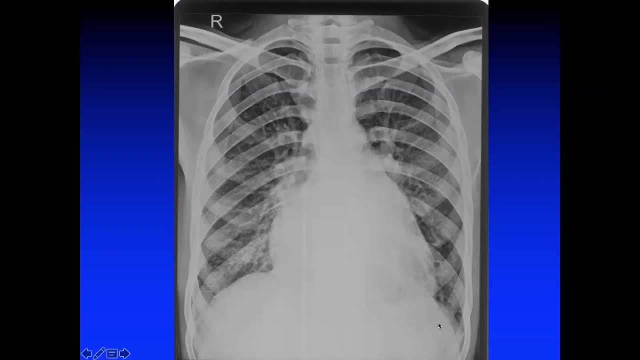 And then you get confused whether it is an LV apex or an RV apex on an X-ray. So an LV apex always appears as an obtuse cardiofrenic angle, And this is a very hard point. So this is not a very subjective thing. 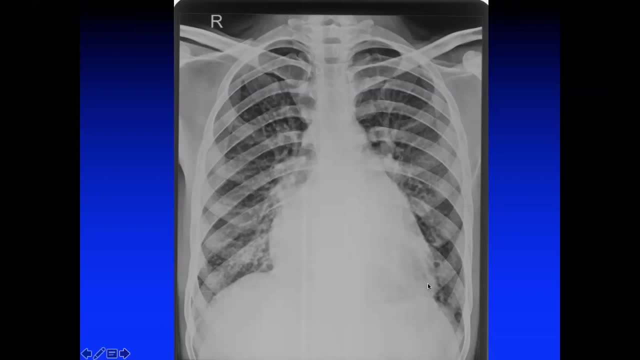 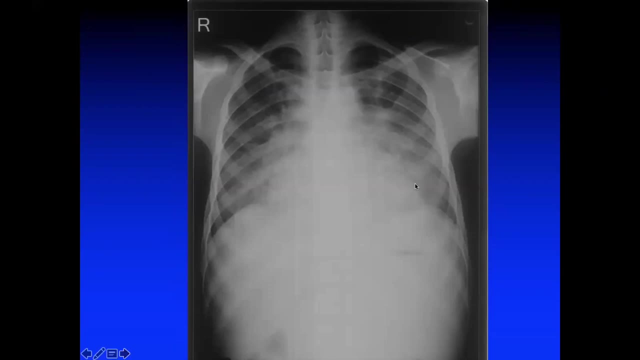 This is a very objective thing. Sometimes a subjective appearance would be that downward displacement might look hard, But if an angle is always obtuse, it is always an LV type apex. Again, you can see the angle very clearly. The angle is obtuse. 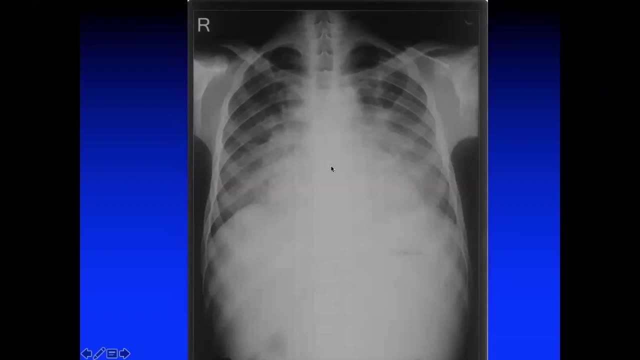 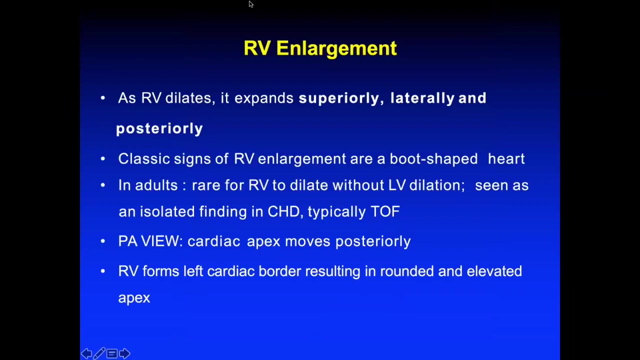 So this is again a classical example of cardiomegaly. CT has more than 0.5. And you will have a LV apex. Now right ventricle. Right ventricle: as it dilates, it expands superiorly, laterally and posteriorly. 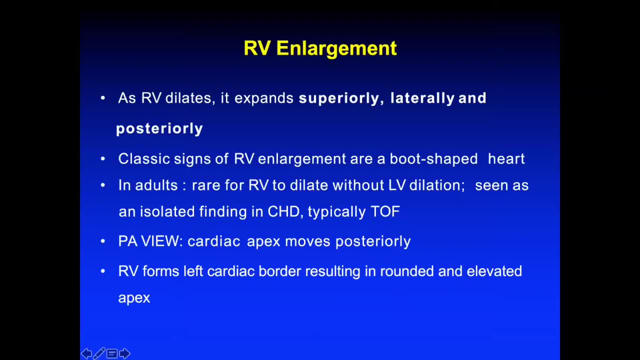 So right ventricle is always an anterior structure, So it can never go anteriorly. So either it will go superiorly, ever It will go laterally, Or it will go posteriorly. So the only way a right ventricle to go is to displace the left ventricle. 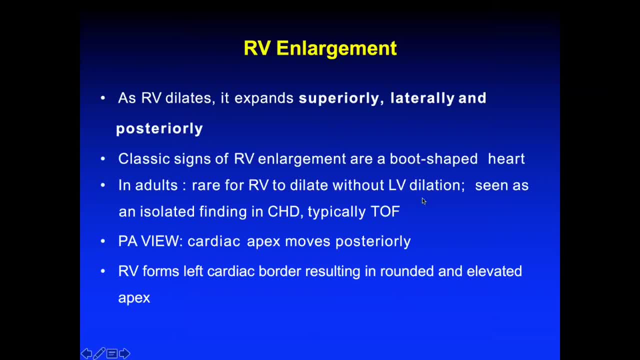 So classical science of right ventricle or boot-shaped heart, Classical is seen in Tetralogy of Fallot. In RV, PA view the apex moves posteriorly. So that is there. So RV, the cardiac apex moves posteriorly. 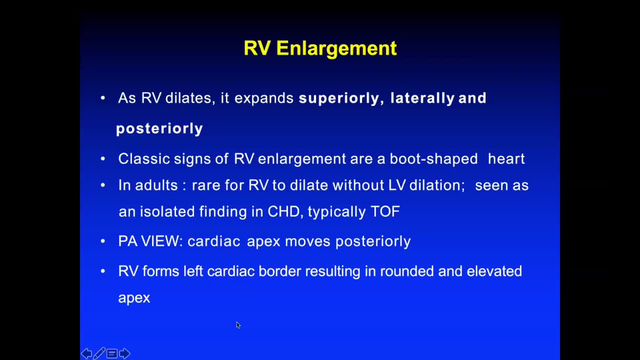 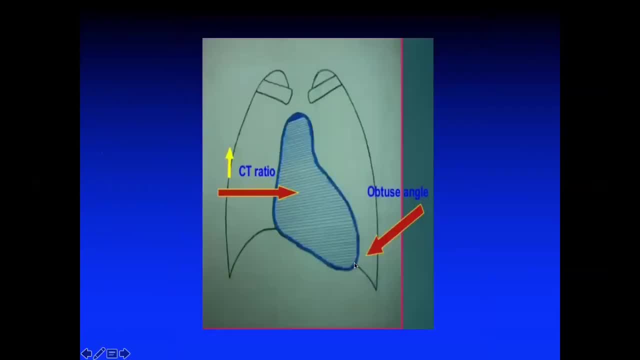 And the right ventricle forms the left cardiac border, resulting in rounded, elevated apex. Now this is a very common problem, Because someone had a doubt that how does this form? the obtuse angle? See the angle- is the cardioprenic angle. 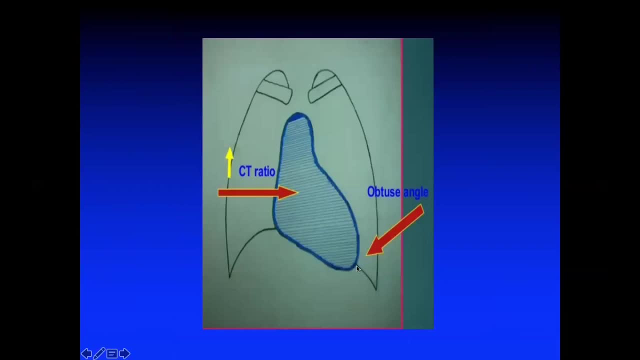 The angle which The heart shadow, which makes the diaphragm. This is the angle And that angle is the obtuse. So anything which is more than 90 degrees is the obtuse angle. So from the apex where it cuts the diaphragm, just measure this angle. 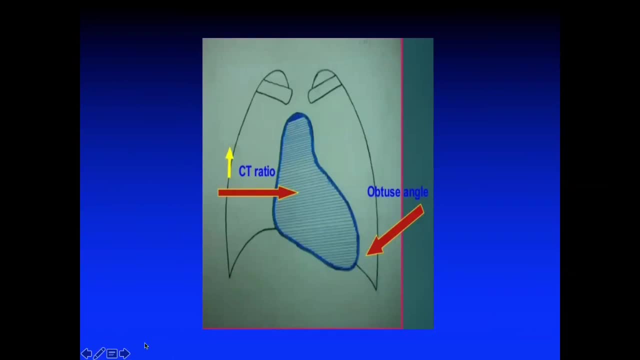 So this angle? it appears more than 90 degrees, So it is basically an obtuse angle If you try to be an acute angle. So whenever you are using an RV apex, I just that how an acute and obtuse is different. so just see this diagram here. the angle: this is the angle. 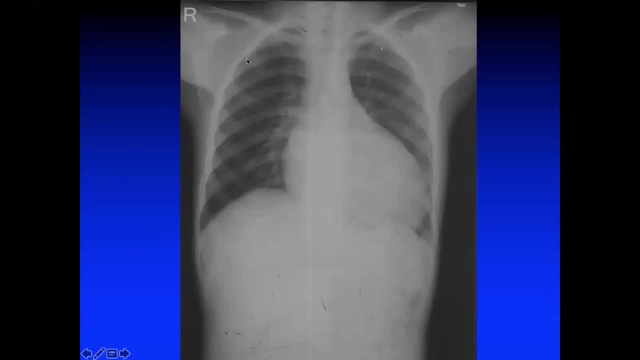 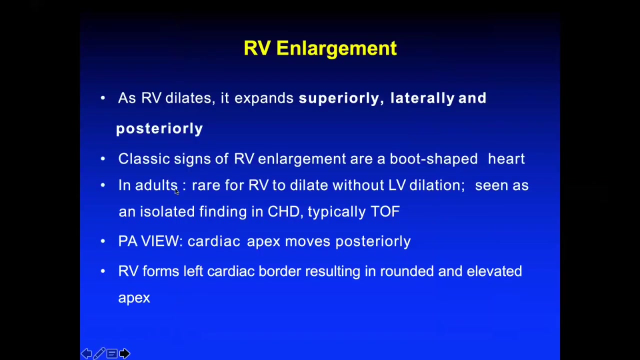 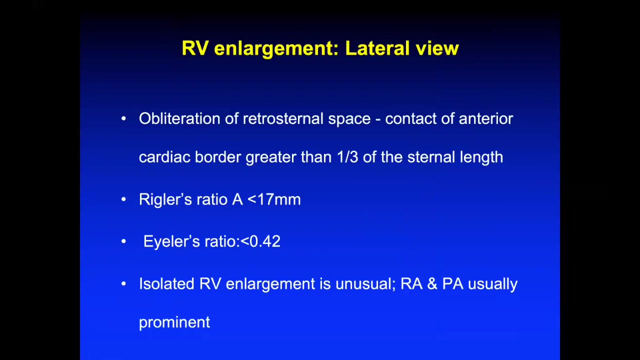 so if it is more than 90 degree. so, uh, that is an obtuse angle. when you see an rv apex xl, you will be clearly be sure that what is, uh, the difference? so rv apex, the angle is acute as compared to lv apex. so rv apex always goes horizontally and lv apex goes inferiorly, so there. 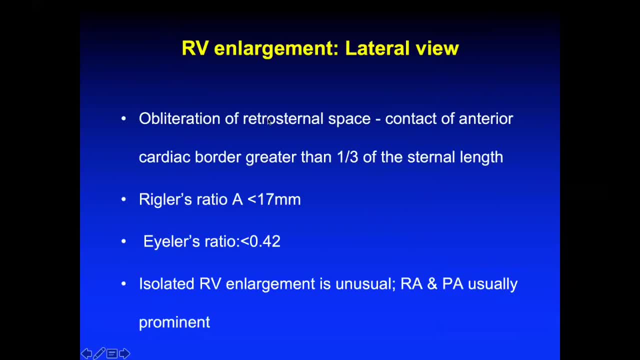 are two points: rv enlarge in a lateral view. this is the most important question. examiner asks you: how do you see your lateral view? because obviously, uh, these days we are never tuned to see a lateral view x-ray and, uh, the examiners know this, so they'll ask you to obliteration of retro strenuous. 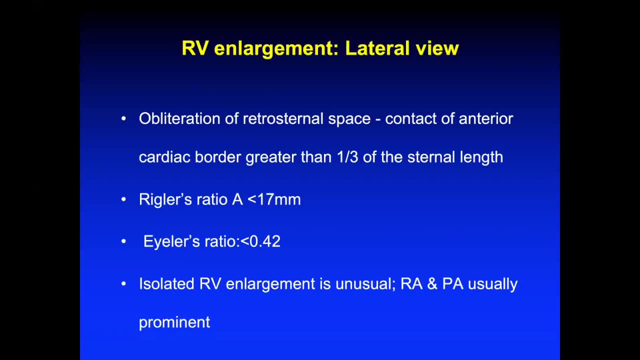 space. as i said you, that rv is the anterior structure on a lateral view. so if the rv enlarges the retro strenuous space behind the sternum, whatever space is there, it will obliterate. so the contact of anterior cardiac border is more than one third of the sternal length. this is the 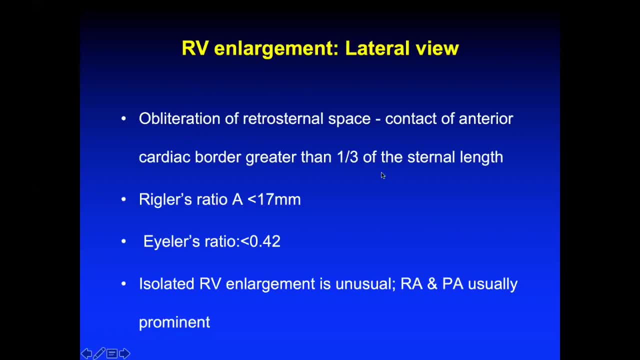 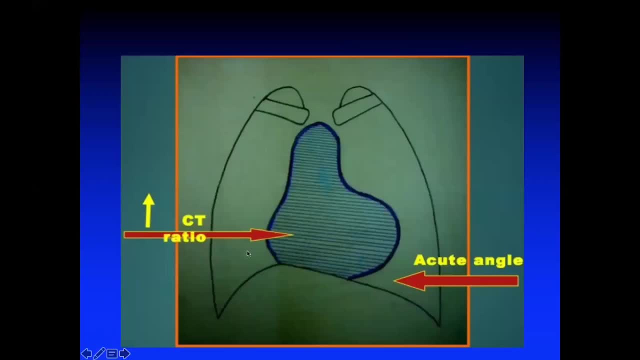 criteria for rv enlargement on lateral view, if you just just remember that that this is the criteria, eiler's and ratio regularization not being required at your level. so this is again cardiothoracic ratio and this angle. i was saying this is the angle which is acute, less than 90 degrees if 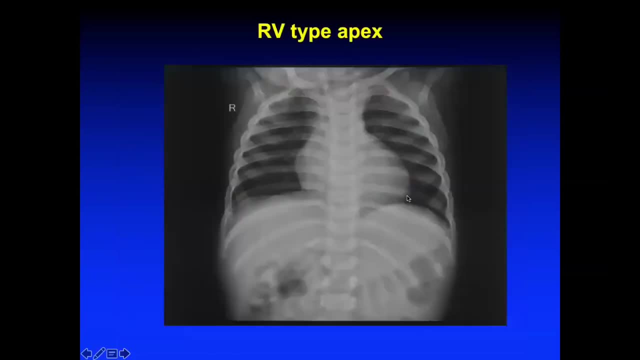 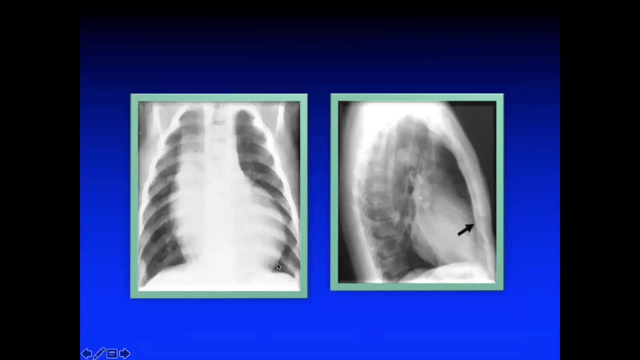 the angle is more than 90 degrees obtuse. so here you can see this angle which is less than 90 degrees. so this is basically a classical example of tetralogy of fallot, an x-ray which is right. again, this angle: less than 90 degree. so this is basically an angle which is an acute 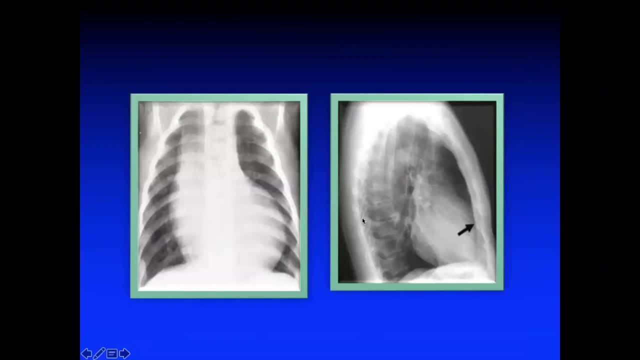 angle which is less than 90 degrees. so this is basically an angle which is less than 90 degrees. so this is basically an angle which is less than 90. the depth angle: uh, around 40, 35, 40. the depth angle, uh, around 40, 35, 40 degrees. and this was theấying, that obliteration of the 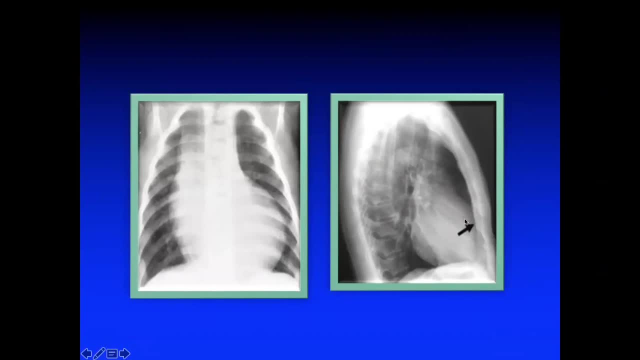 retro strenuous space. normally this black area is present because the lung is present. if the right ventricle enlarges, this area becomes more radial, uh, opaque, and you will have obliteration of the uh right, uh. this board erased space. second point would be one THIRD of sternum, so sturnum. 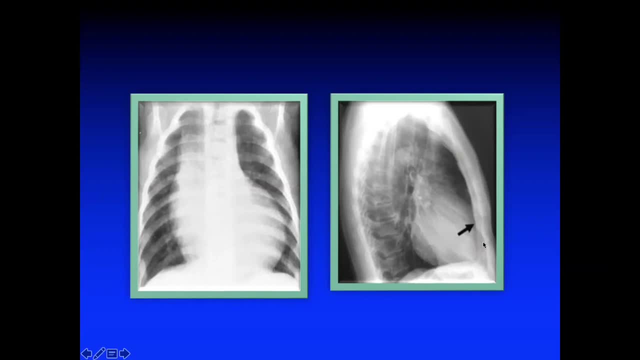 the length of the sternal is from here to here. at least one THIRD of the stue calibration length is being in contact with the right ventricle. so these are the classical examples. so, based on the location line, you will have the lateral sphincters here in this system. so we are representing Hakari. 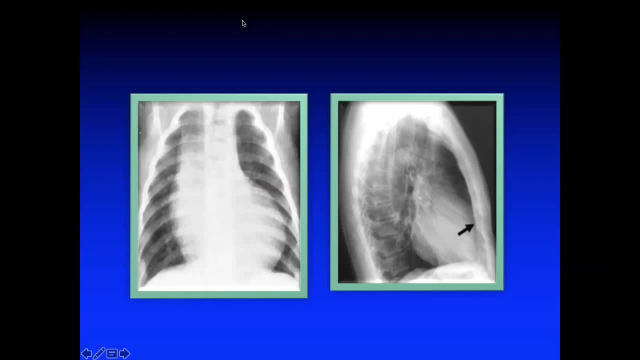 which comes out of the ordinarycribed трassal at braring leg. uh, which is coming this narrow 뭐�, module, which again, exam of retrology, of fallow and uh, that is how you describe our rbfx and uh, lbfx, acute angle, obtuse angle and the direction of enlargement. so here you can see the rv. 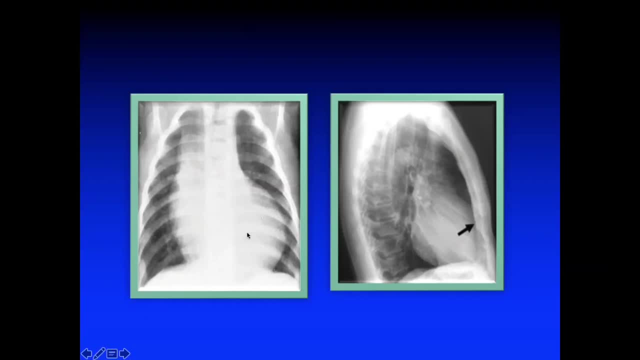 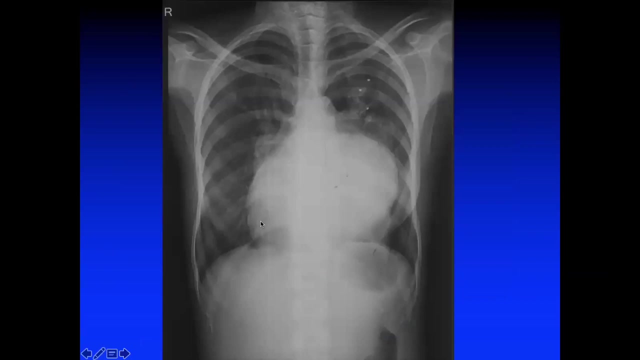 uh, the fx is going around the left side so it is horizontally displayed in an uh lbfx. it is obtuse and uh inferiorly or downward displacement, so with that you can clearly make out an lb versus rbfx. so sometimes you know, apex might not be visible and here you can say that, uh, so this. 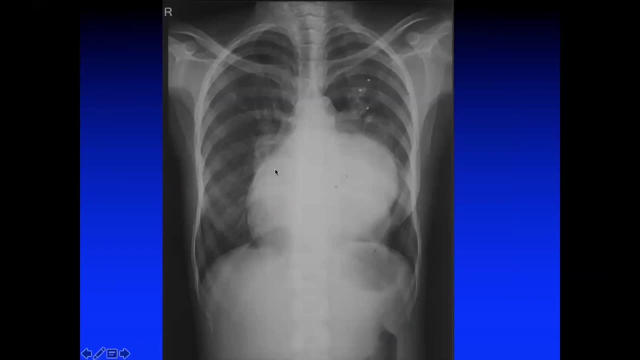 is because a left atrium which just tends to occupy everything and it might blur out, uh, your appearance of left ventricle. this is because an la which you have so much and last, that, uh, the lv is pushed up behind and only you can see is the left atrium. so this might, you might get confused, that.